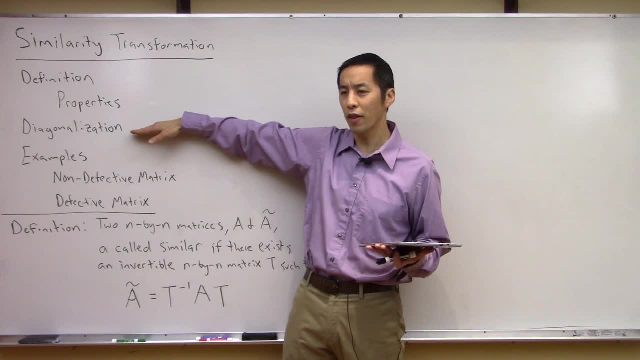 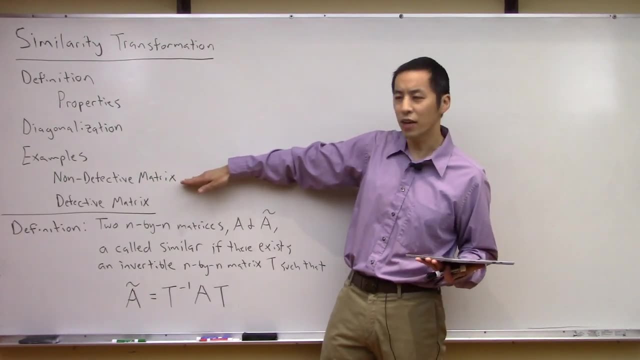 is to perform what's known as diagonalization, and we'll talk about that Before going into some examples, we'll do two examples, One using what's known as a non-defective matrix and the other using a defective matrix, just so we can see the difference. And again, this will make sense. 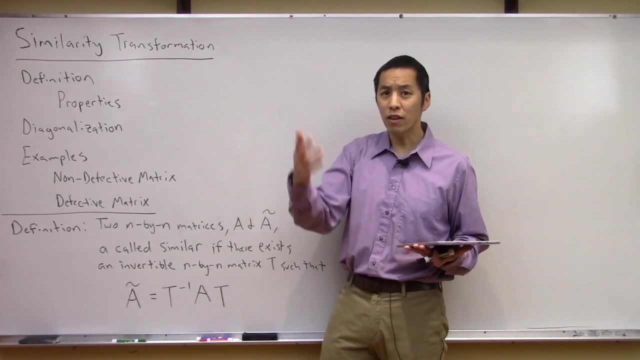 what these two mean when we get there. So if that sounds like fun, why don't we just go ahead and jump right into it? So what's the definition of a similarity transformation? So what's the definition of a similarity transformation? So what's the definition of a similarity transformation? 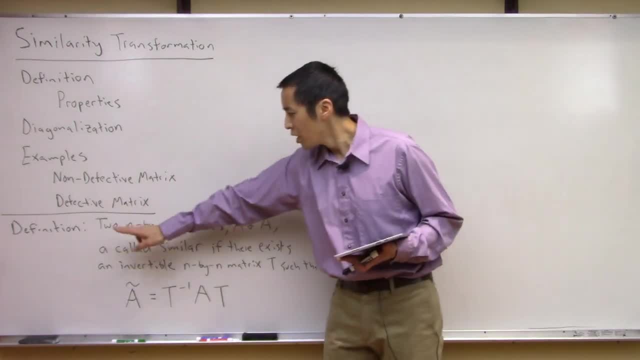 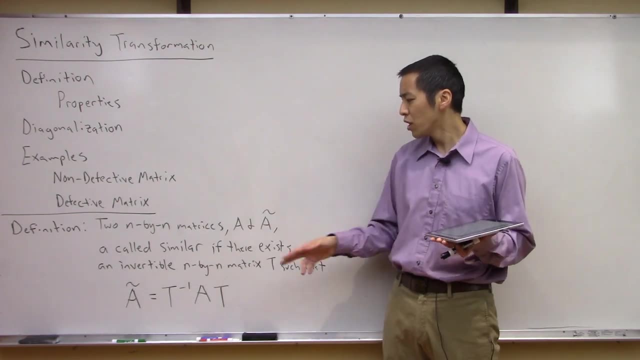 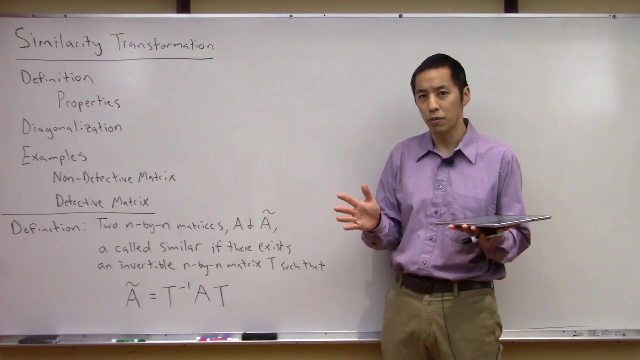 The definition is that if you have two square matrices- square meaning they're of dimension n by n- let's call these matrices a and a tilde. These two matrices, a and a tilde, they're called similar. if there exists an invertible square n by n matrix, Let's call this matrix t, for like a. 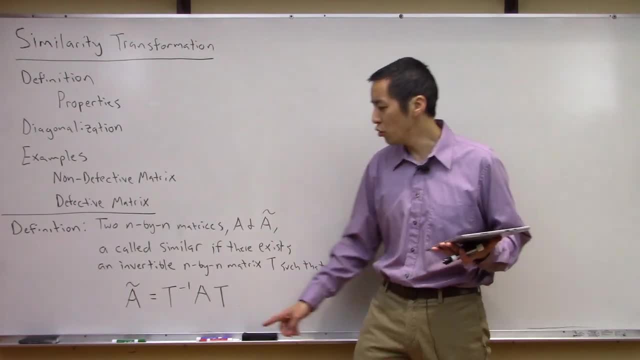 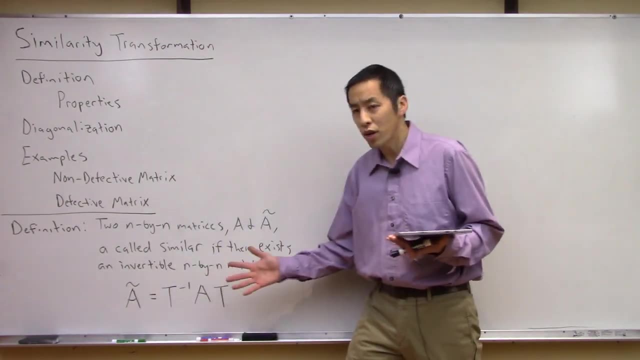 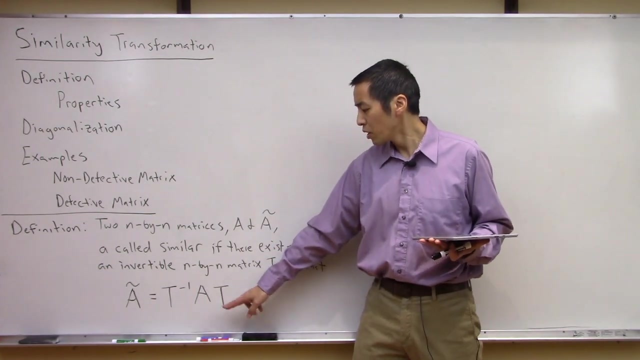 transformation or a similarity transformation matrix, such that you can basically take a left multiply by t, inverse right multiplies by t and you get a. So in other words, a tilde is equal to t inverse a t. So if this is the true, if you're able to find this matrix t, you basically have. 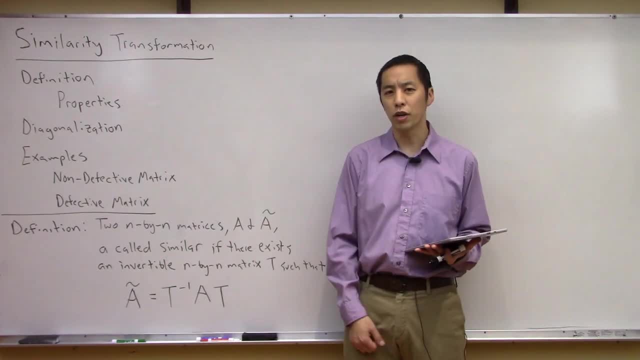 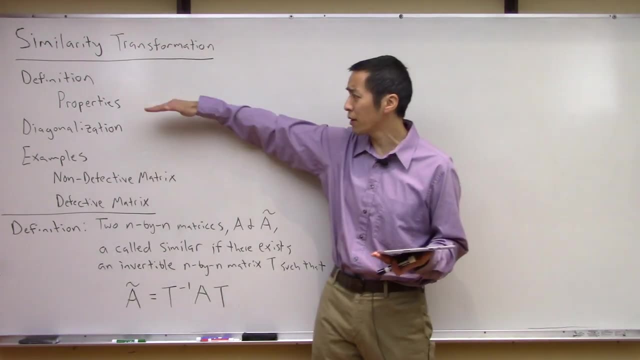 these matrices, a and a tilde, which are similar to one another. We're going to see what that means. It means that a and a tilde share some properties. In fact, why don't we start talking about that right now? Let's go through. we're going to see there. in this discussion I like to talk about 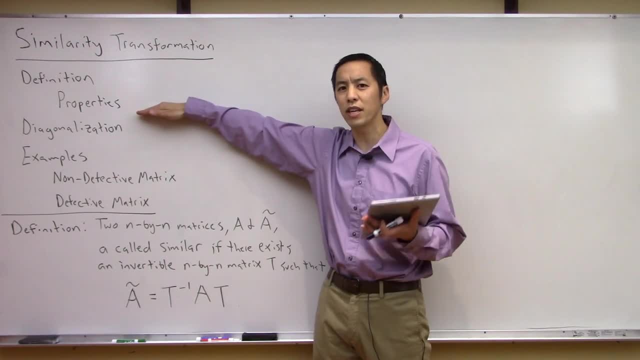 five different properties of the matrix t. So let's go through we're going to see there in this discussion. I like to talk about five different properties of the matrix t. So let's go through matrices a and a tilde and we'll see how they relate to one another. Okay, so the first property. 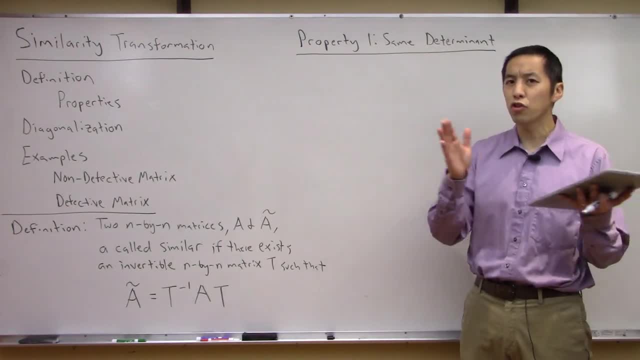 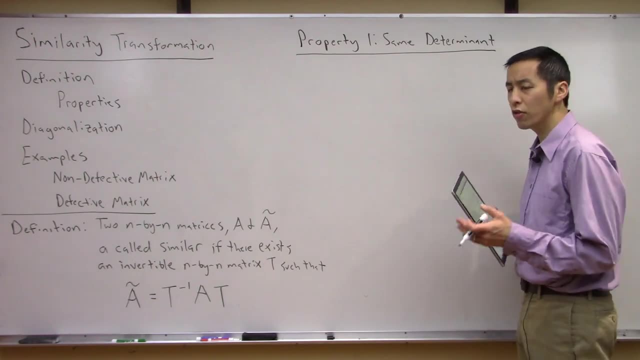 that I'd like to investigate is the determinant of a and the determinant of a tilde, and we're going to see that actually both of them have the exact same determinant. Okay, so to do that, let's go ahead and make use of a couple of matrix properties, and again in this video, I like to 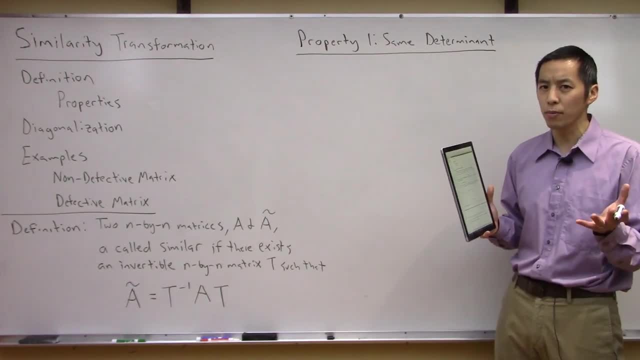 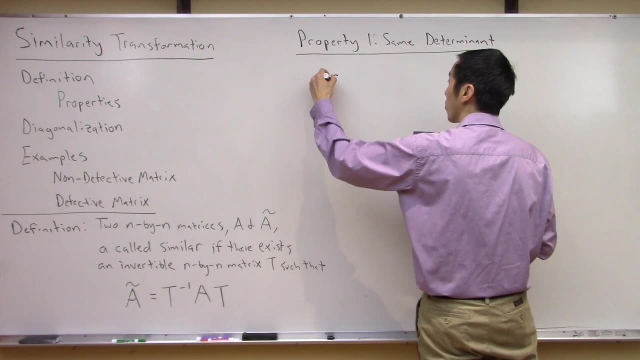 focus just on the similarity transformation, not some of these individual matrix properties. So, for example, I'm just going to pull this out of thin air. You feel free to verify this if you'd like, but if you recall right the determinant of a matrix, if it's a product, let's say a times b. 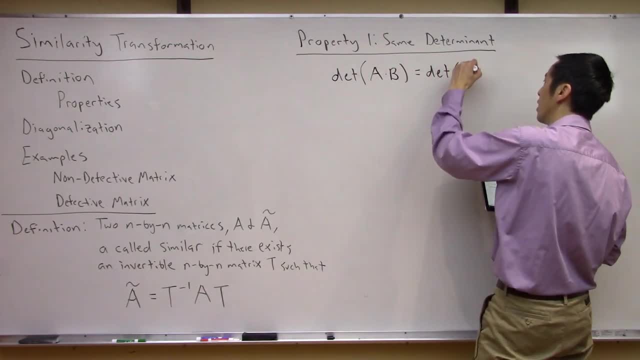 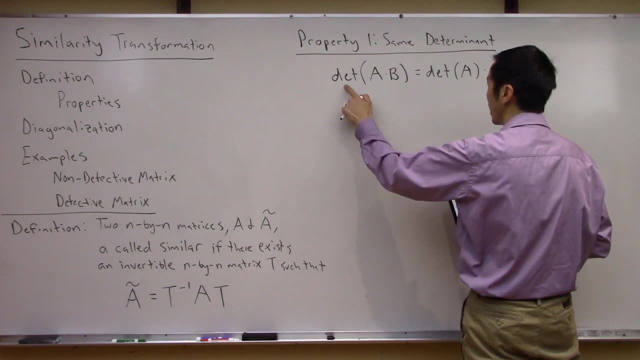 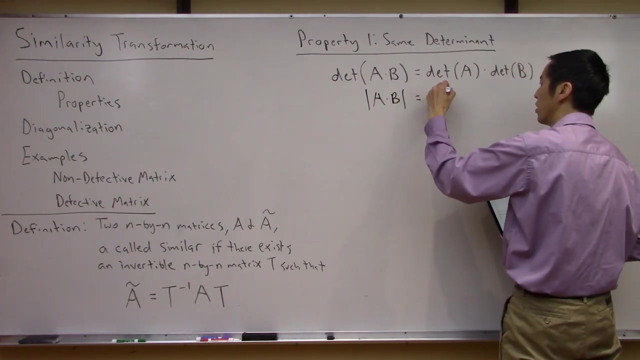 right, this is the same thing as the determinant of a times the determinant of b. Okay, so we're going to make use of this and, in fact, in order to avoid writing debt all the time, I'm just going to refer to this as a times b. determinant right is equal to determinant of a times. whoops, oh sorry. 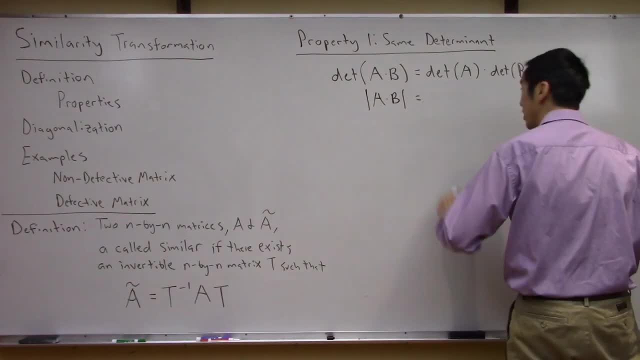 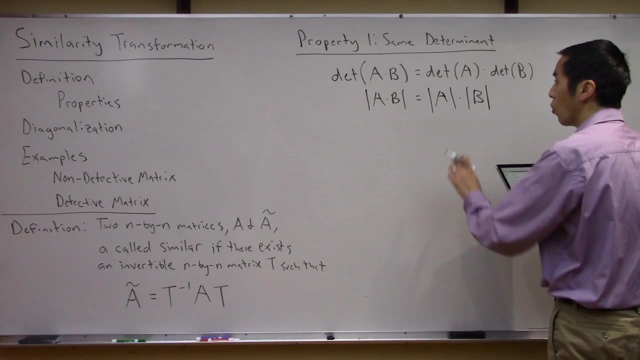 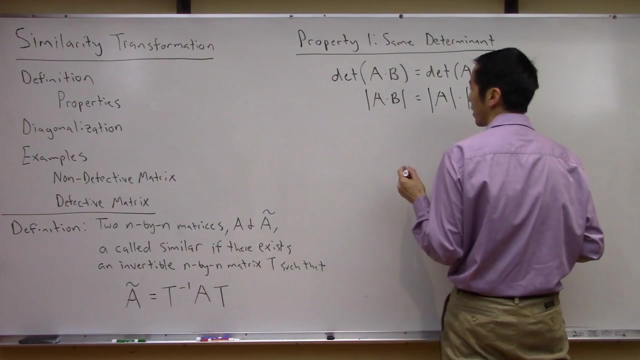 I just I did it the right here. I was trying to avoid writing d e t all over the place, So I'm going to use this bar notation to represent a determinant. Okay, so let's recall this. this is one property of determinants that we're going to use. The other one that I'd like to everyone to 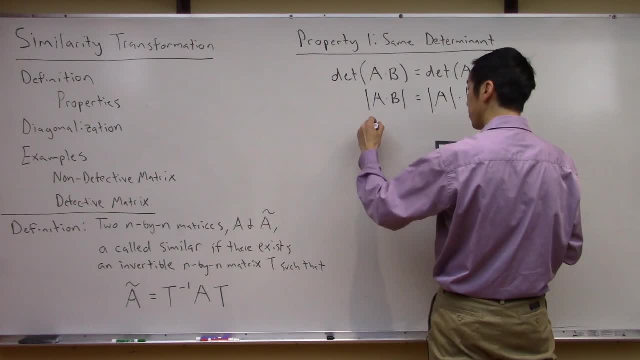 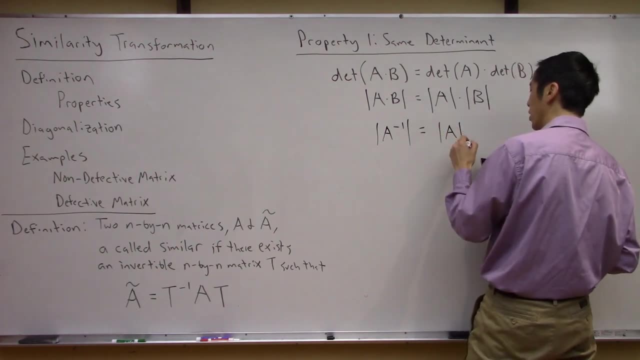 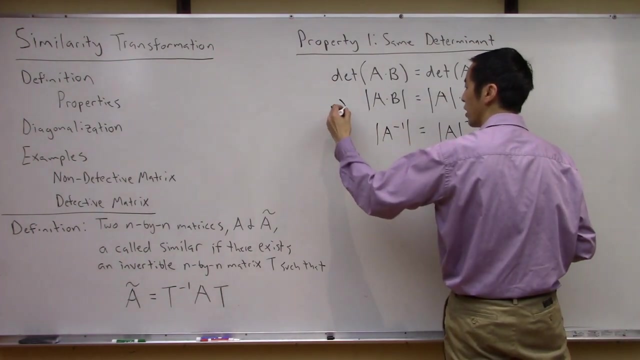 remember is if you have the determinant of a matrix inverse, this is actually the same thing as the determinant of the matrix to the negative 1 or 1 over the determinant of the matrix. Okay, so these are properties, p1 and p2. maybe again these are just properties of determinants They have. 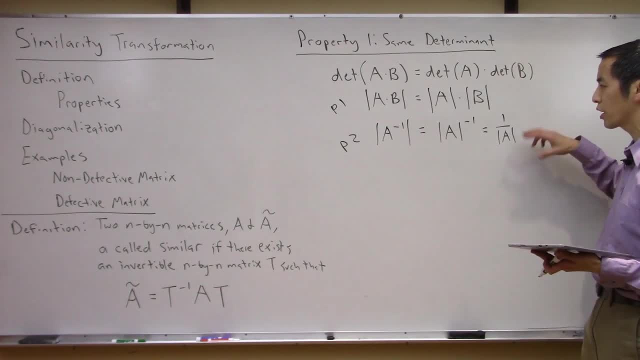 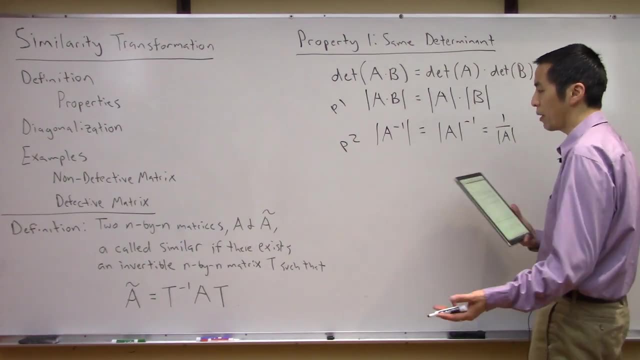 nothing to do with similarity transformations. this is just how determinants of matrices work. Again, feel free to verify this on your own. but now let's apply these two to our definition of our similarity transformation and see what pops out. So let's go ahead and investigate. what is the 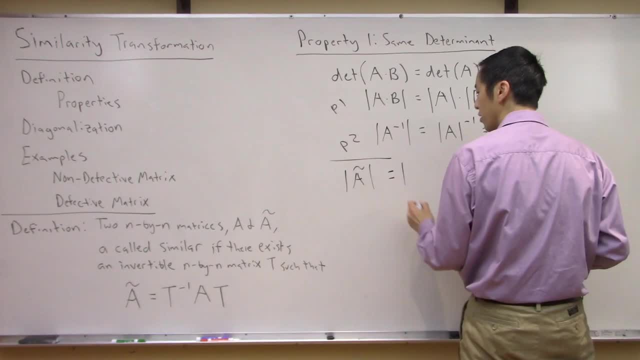 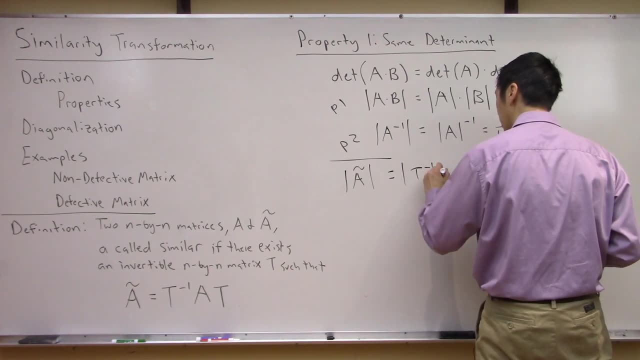 determinant of a tilde, right? Well, the determinant of a tilde, what we said, a tilde is just t inverse- oops, sorry, t inverse a tilde, Right? okay, now let's go ahead and use p1. this is the, a product of three matrices, so I can break. 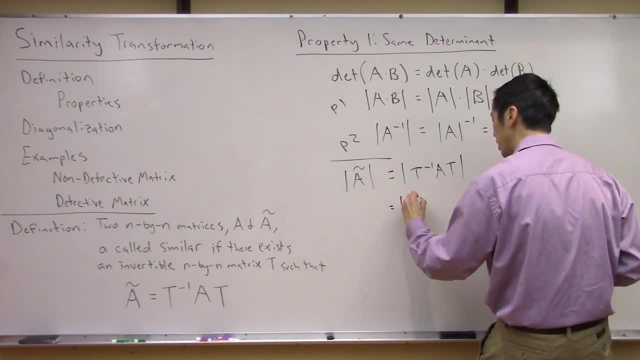 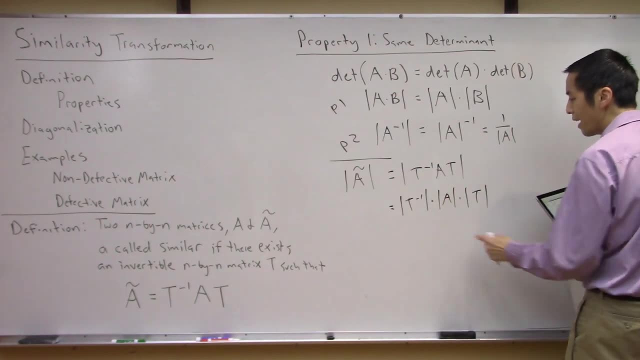 them up into individual determinants. In other words, I can write this as t inverse determinant times the determinant of a times the determinant of t. Okay, great, and now let's go ahead and use this p2 property right where we can see that this is the inverse of t. so that's just one over the. 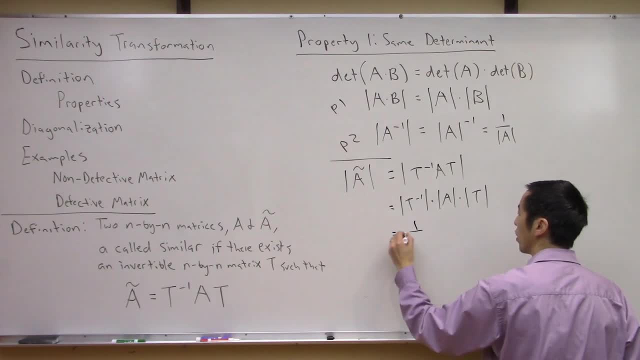 determinant of t. So in other words, this first term can be rewritten as one over the determinant of t Right times determinant of a times the determinant of t Right. and we remember that the determinant it's just a scalar value, right it's just a number. so this determinant in the numerator is going to 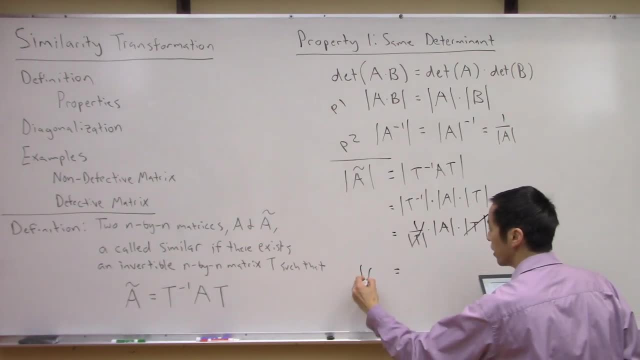 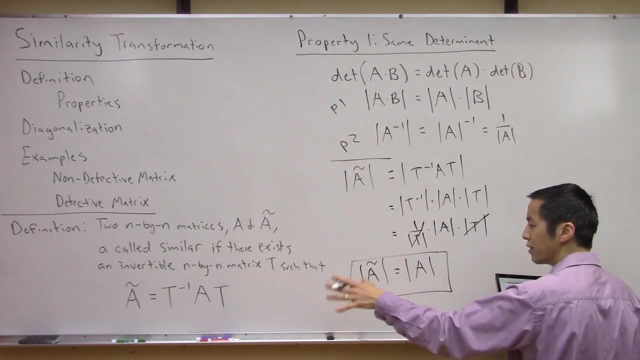 cancel this determinant in the denominator, so we end up with: the determinant of a tilde is actually equal to the determinant of a. So this is fascinating that basically, under a similarity transformation, the determinant remains unchanged, right? So even if you provide this, you know you. 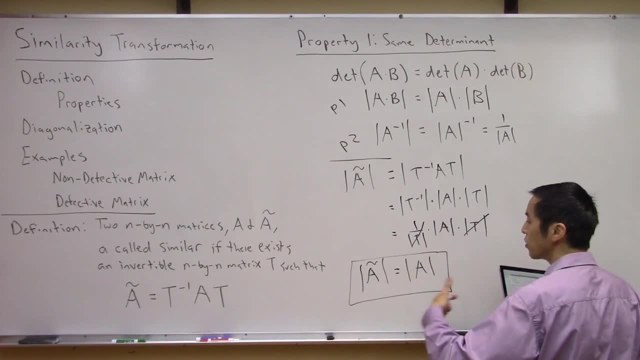 perform this determinant of a tilde, you're going to get a determinant of a tilde. So this is similar to transformation. as long as t is invertible, you can use absolutely any t and it's not going to change the determinant: A tilde will still have the exact same determinant as a. 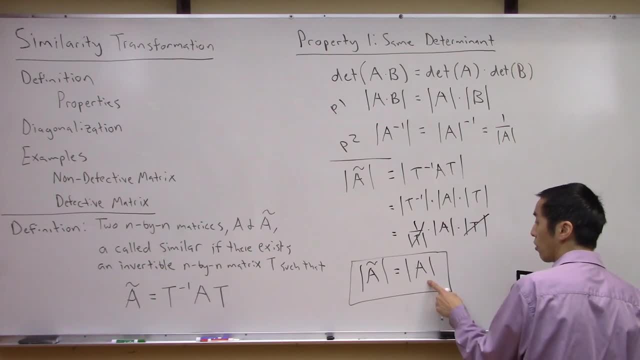 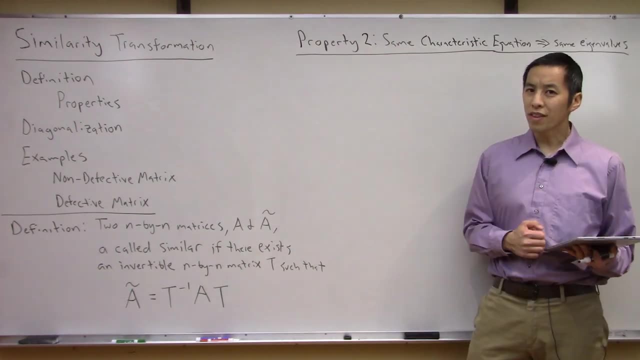 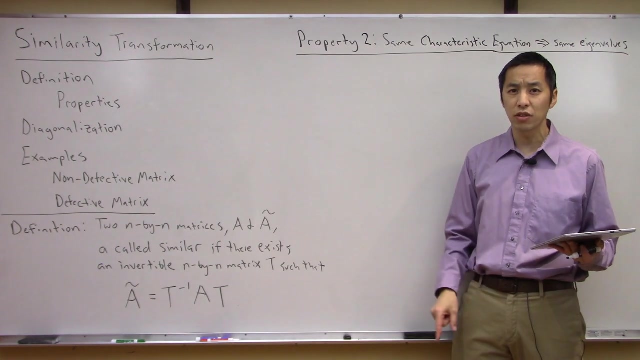 basically the same determinant that you started with. Okay, so that's the first property. Let's go ahead and look at another property. Okay, so the second property that I'd like to investigate, and we're actually going to see that the characteristic equations of both a and a tilde right the matrix. 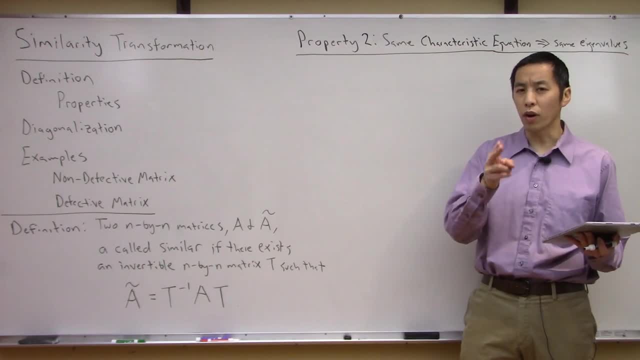 characteristics of a and a tilde are going to be the same. So let's go ahead and look at the characteristic equations. We're going to see they're the same and therefore, if you remember, you solve the characteristic equation of a matrix in order to find its eigenvalues. So if the 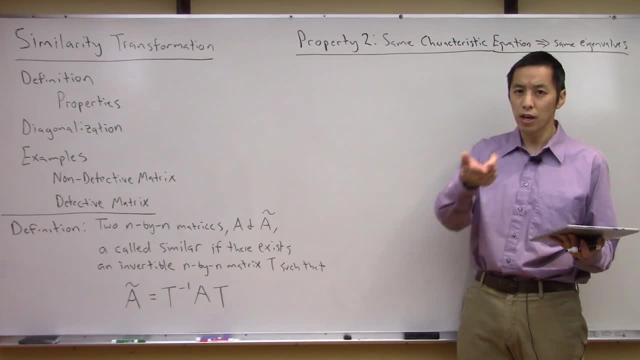 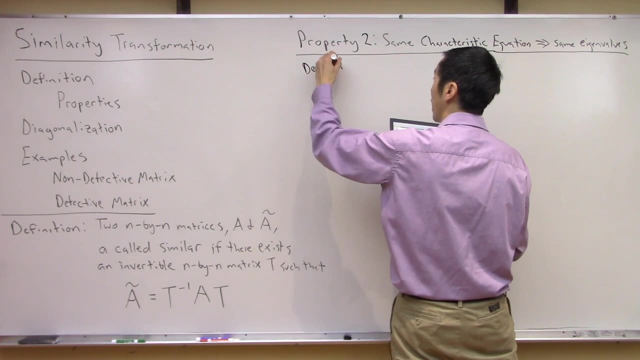 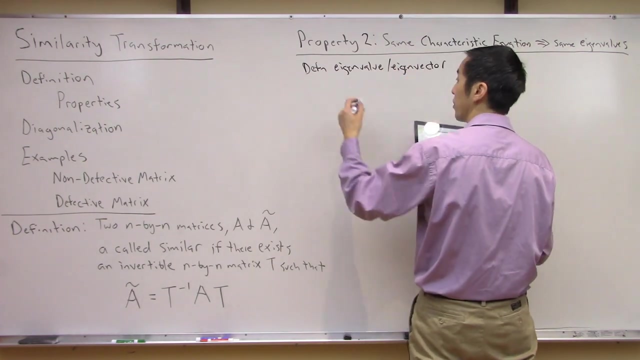 characteristic equations are the same, the eigenvalues are going to be the same, right? So let's go ahead and prove that right now. So if you recall the definition of an eigenvalue, slash eigenvector, right, Do you remember this? for matrices, this is very common. It basically says: let's start with. 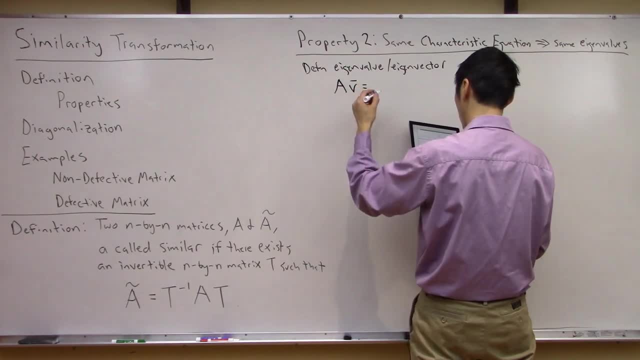 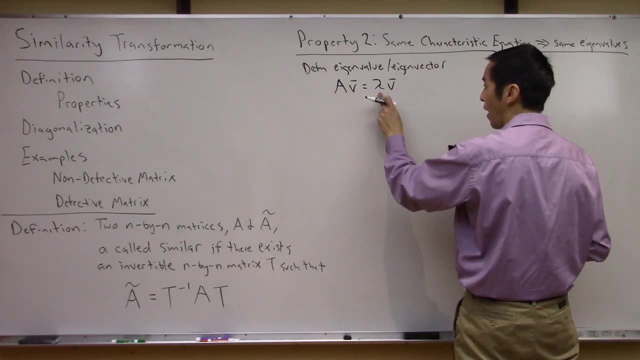 the matrix a right. So a v is equal to a and a tilde is equal to a tilde. So let's go ahead and look at the characteristic equations. So let's go ahead and look at the characteristic equations. So if this is true, then lambda is an eigenvalue of the matrix a and v is the associated eigenvector of. 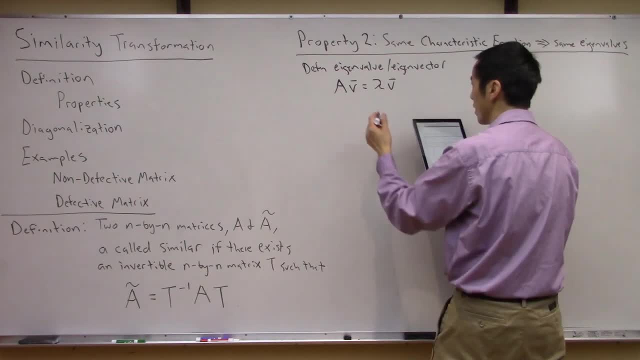 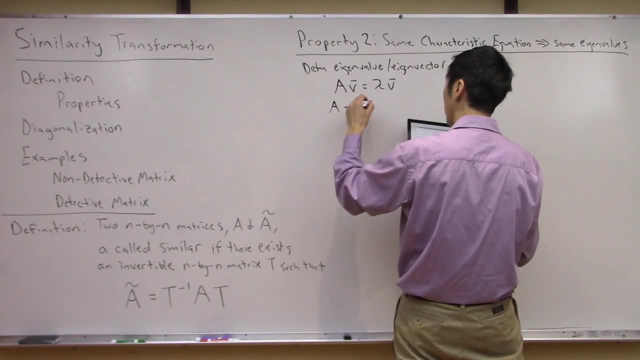 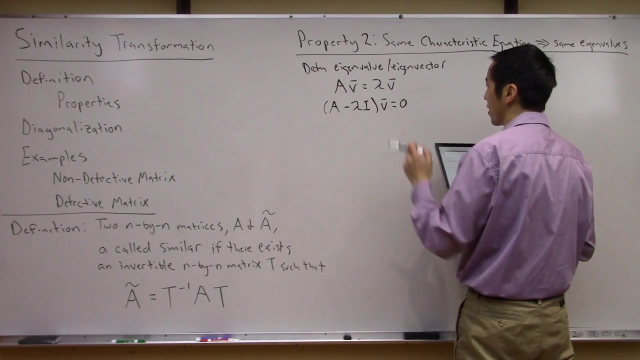 that matrix a right. So let's go ahead and rewrite this, So I can rewrite this as, basically, a minus lambda times the identity matrix, times v, is equal to zero. right, That's the exact same thing. Basically, move it off to the other side. factor out the v. This is the same thing. 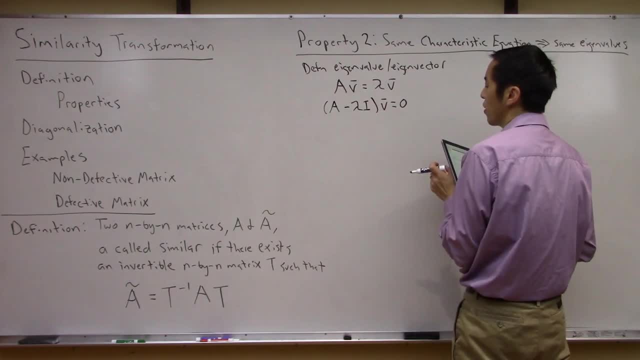 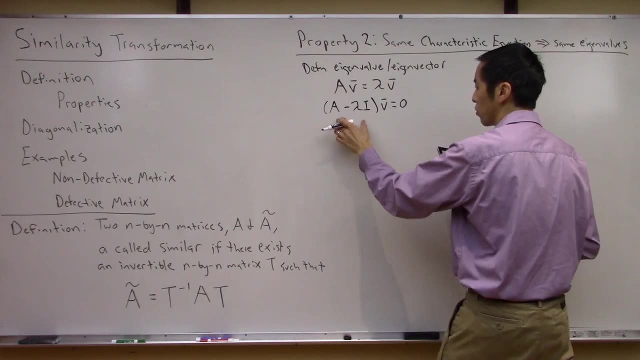 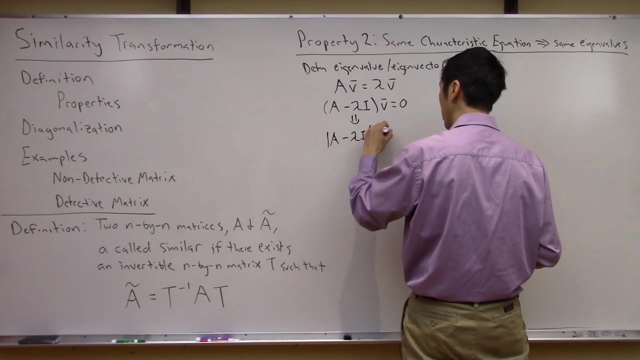 Right, And we see that basically, the only way that this is true for a non trivial v is that this determinant has to be equal to zero. So in other words, we see that basically, this implies the determinant of a minus lambda. i has got to equal zero, right, And this was your basically. 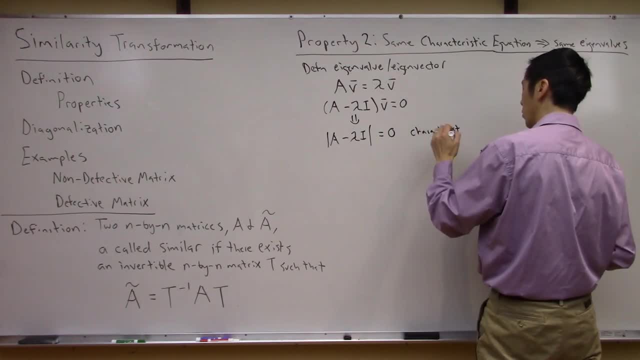 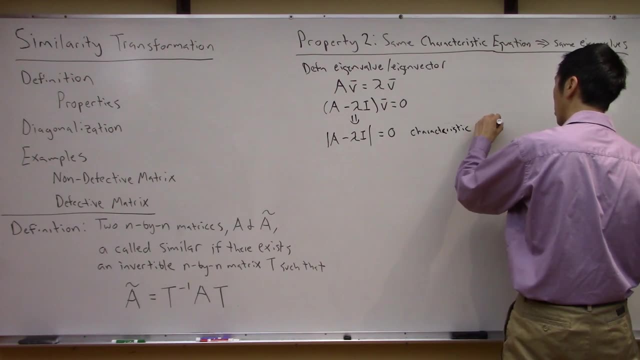 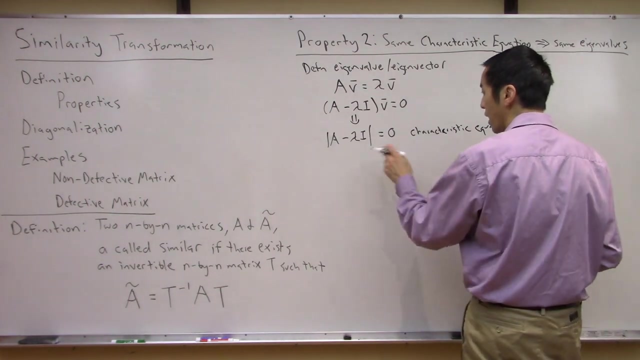 your matrix characteristic- Whoops, sorry, I totally spelled that wrong- Characteristic equation. Right, That's your matrix characteristic equation. You basically solve this thing for lambda, Right? OK? So now let's go ahead and rewrite this using the fact that a is related to a tilde. So 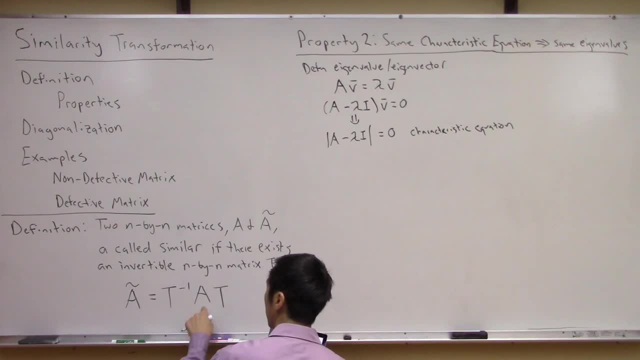 again. maybe it might be. it might help us if we come over here. since t is invertible, right, I could just go ahead and left multiply by t inverse and no sorry, left multiply by t right, multiply by t inverse. In other words, I can rewrite this thing as what it's: t a tilde, t inverse. 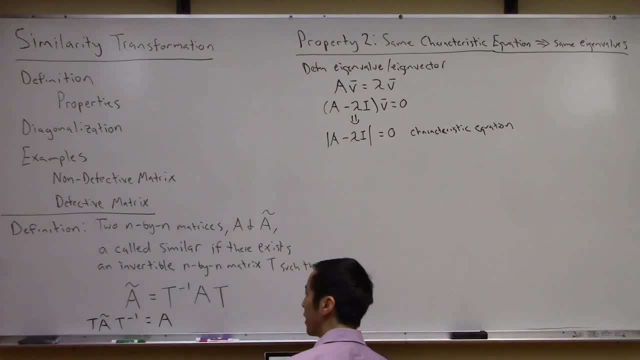 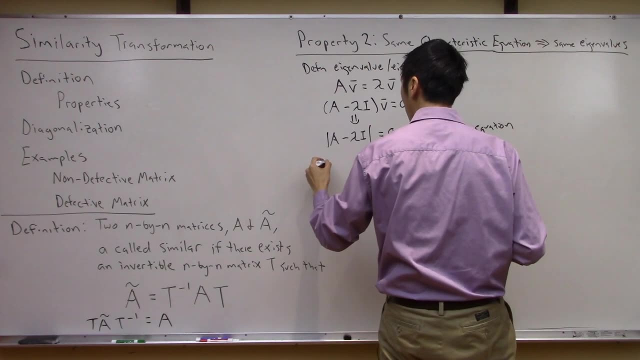 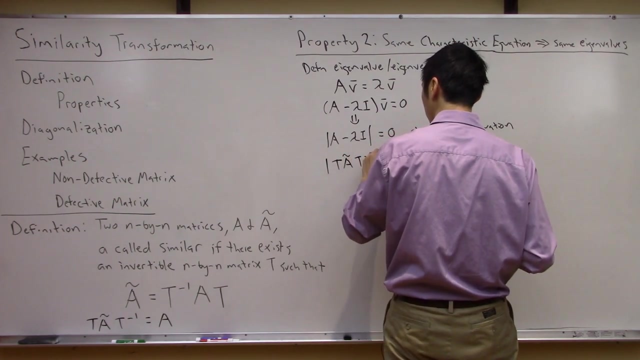 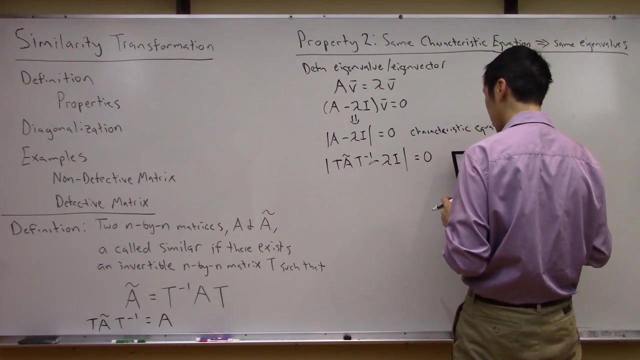 It's equal to a. That's the exact same thing, Right, OK? So now substitute this, this in for a Right, OK, So we have. what do we have here? This is t, a tilde, t inverse minus lambda identity matrix, Right. The determinant of that whole thing has got to equal zero, Right? OK, Let's go ahead. 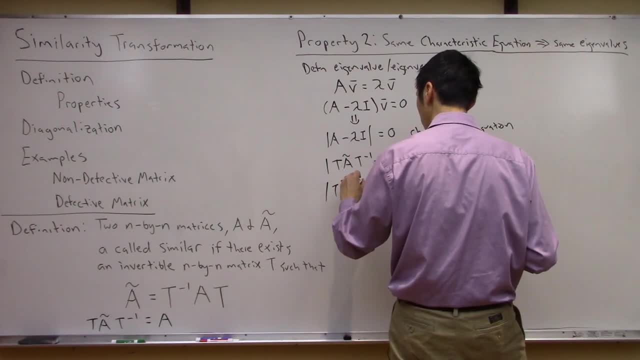 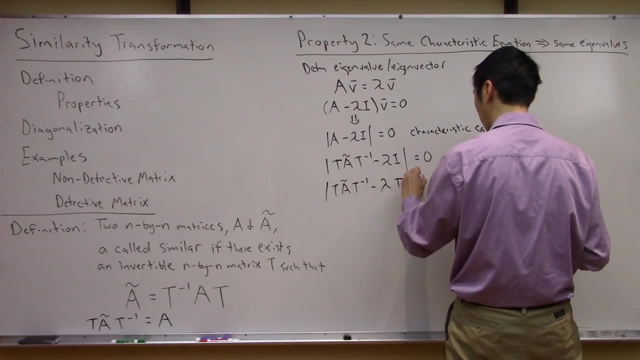 and write this again. So I got t a tilde, t inverse minus lambda. So the identity matrix- I can write this thing as t times t inverse, if I want, Right, That's the same thing as identity matrix- is equal to zero. OK, So that's going to. 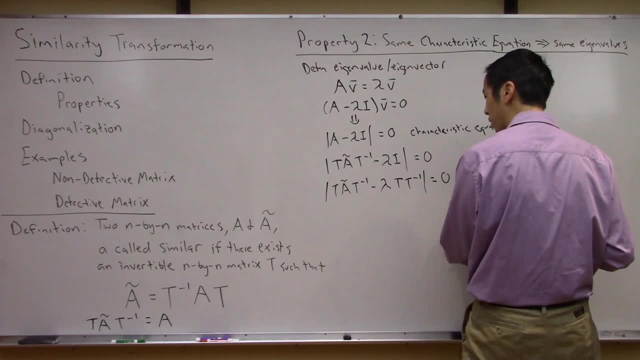 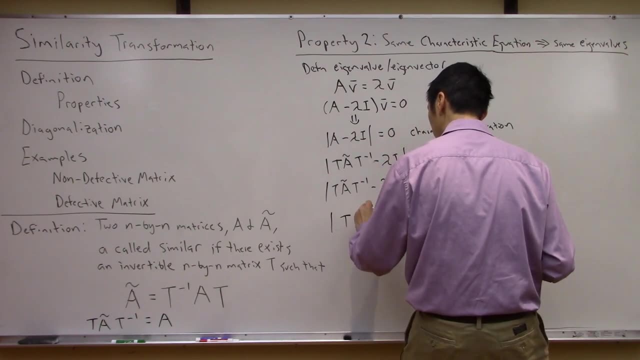 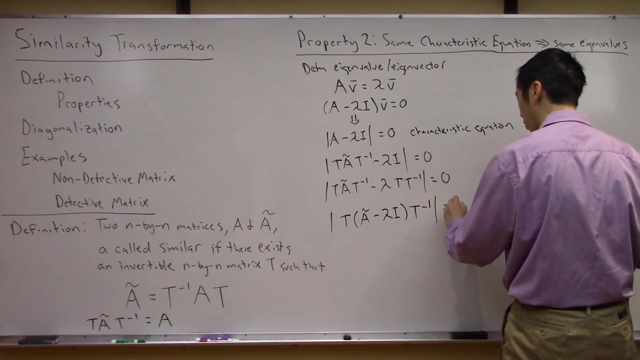 allow me to left factor out a t and right factor out a t inverse. So we end up with basically t times the quantity, a tilde minus lambda identity matrix, and then t inverse Right. The determinant of that whole thing has got to equal to zero Right Now. this looks a whole lot like what we did. 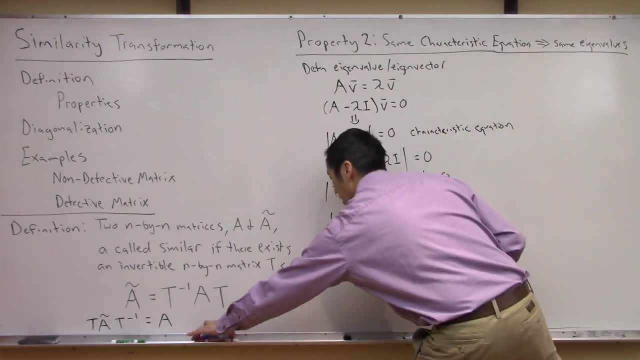 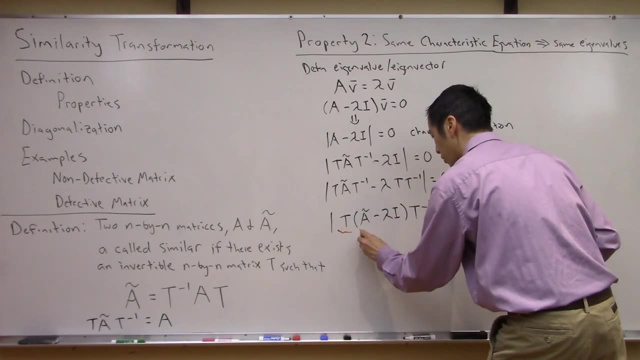 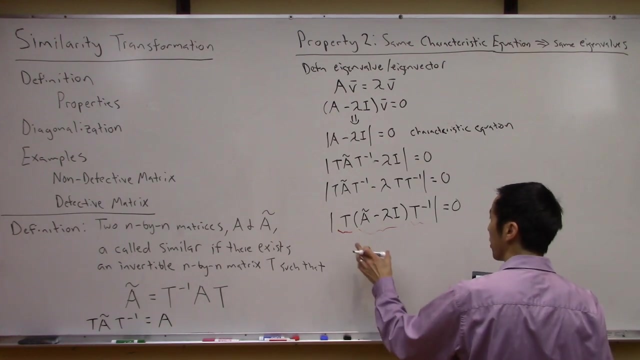 in property one. This is a product of three matrices. Right, You've got t here. Here's whoops, that pen is totally dying. That's one matrix. Here's second matrix. Here's the third matrix. Well, that pen's also dying, OK, So let's go ahead and use our property of. this is the determinant. 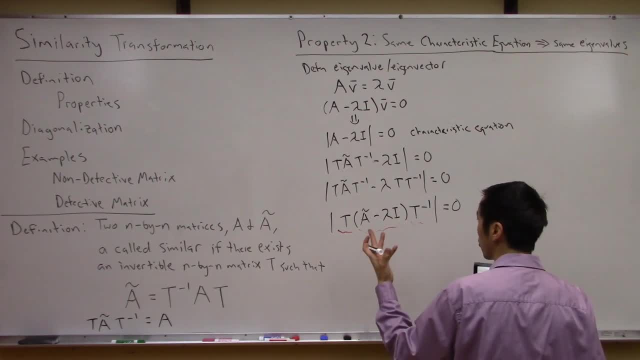 of the product of three matrices. Let's break this up into three individual determinants. So I have determinant of t, That's matrix one times determinant of a tilde minus lambda. I times the determinant of t, inverse Right. That's got to equal zero. OK, Now we do the exact same thing. 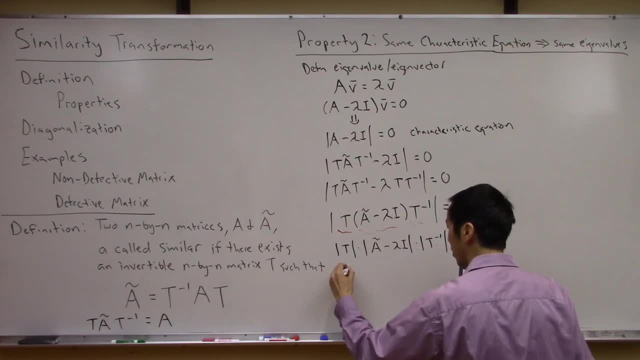 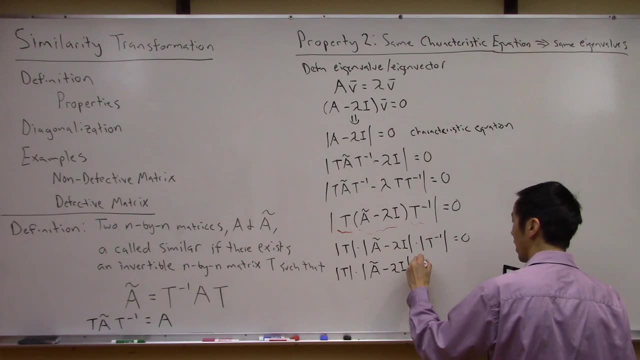 we did last time, Right This. Well, let's not skip any steps. Right Times a tilde minus lambda, I times Right. This is now the same thing as determinant of t to the negative one, Right. So again, this is a scalar number which cancels with that scalar number, Right. So we end up with: 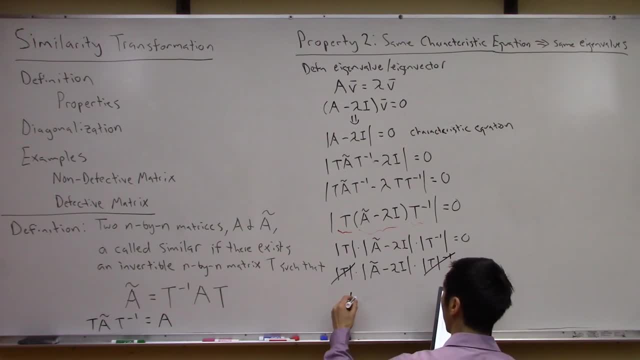 basically the same equation Right. We have a determinant of a tilde minus lambda. I is equal to zero Right. So this is the characteristic equation Right For a tilde Right. This one up here is a characteristic equation for a. 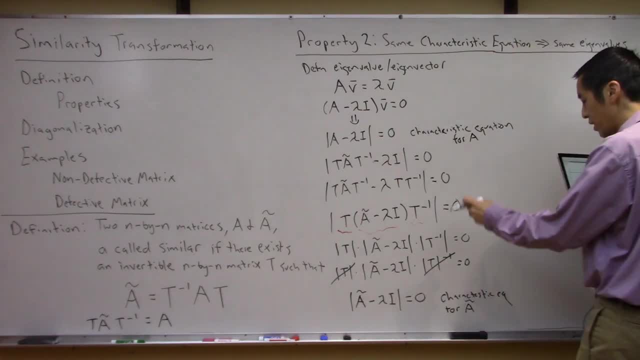 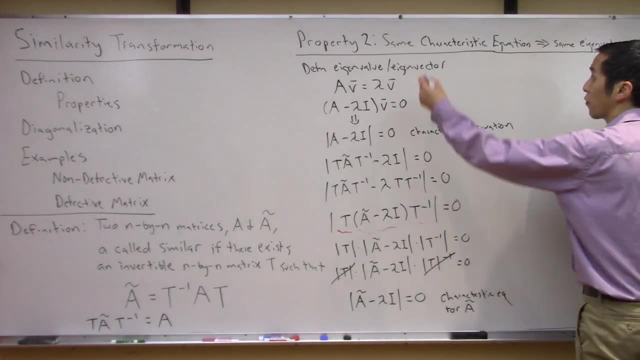 Right, And it's basically the same thing. We basically see that this characteristic equation for a is the same thing as a characteristic equation for a tilde Right. So that shows this first part, that we have the same characteristic equation And basically, since we're solving this, 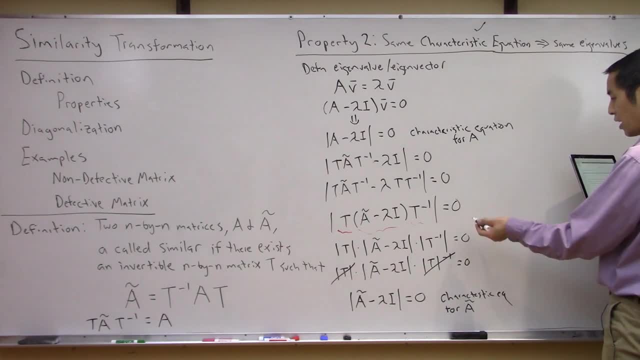 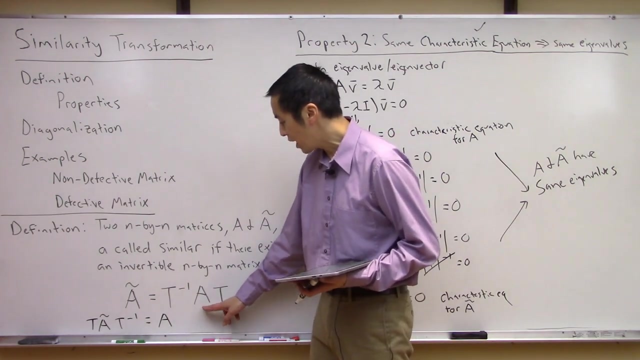 characteristic equation to get eigenvalues, basically those together, Right? Basically, just imply that both a and a tilde have the same eigenvalues, Right? So the eigenvalues remain unchanged underneath any similarity transformation. So as long as t is invertible again, you are not going to change the eigenvalues of a. A will have the same eigenvalues. 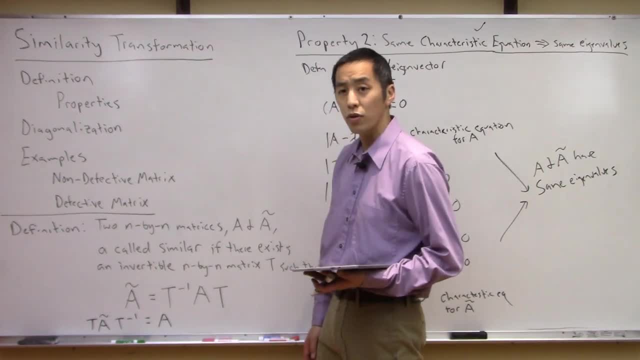 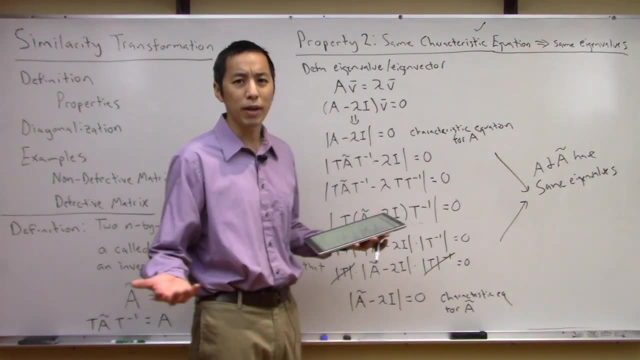 as a tilde, even after you do this, this similarity transformation, Right? So that's, that's pretty interesting, OK? So I guess, naturally, your next question, since we're talking about eigenvalues, is: what about the eigenvectors? All right, So we just show that the eigenvalues of a tilde are actually. 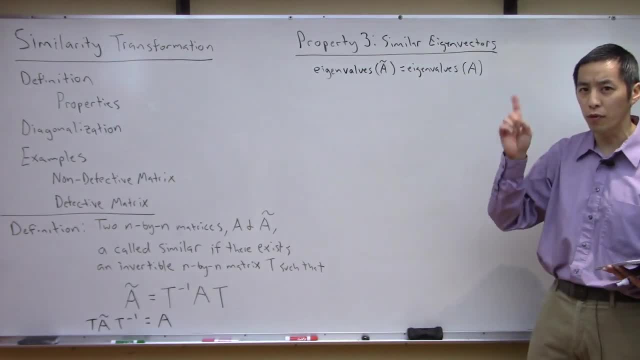 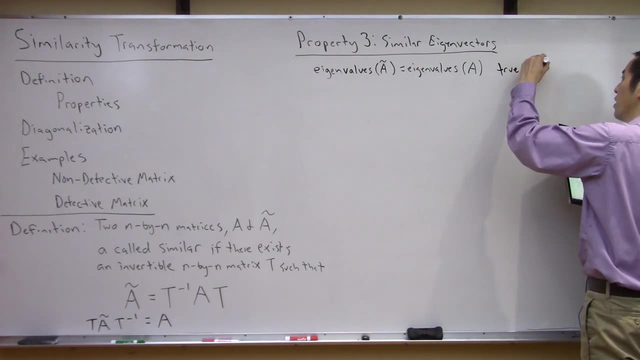 the same as the eigenvalues of a tilde, Right? So we just show that the eigenvalues of a tilde are, and actually I should probably mention, before we move on to the third property: is this is true even with multiplicity? Let me write that down: Even with multiplicity. 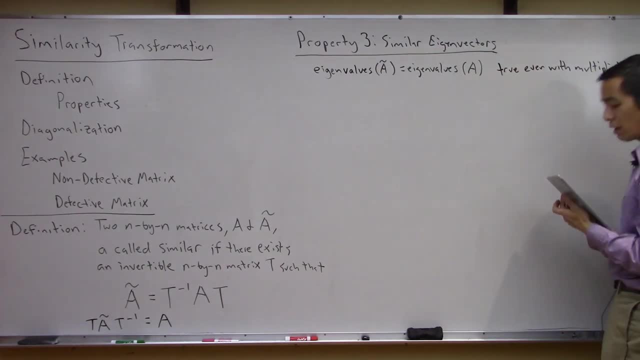 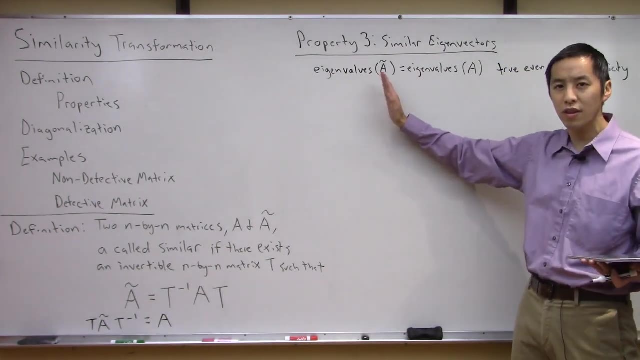 meaning, even if there are repeated eigenvalues in a or a tilde, it's it doesn't matter. This is still going to hold true under the similarity transformation. You'll still have those same repeated eigenvalues showing up in a tilde. OK, So that's the discussion on the eigenvalues. So 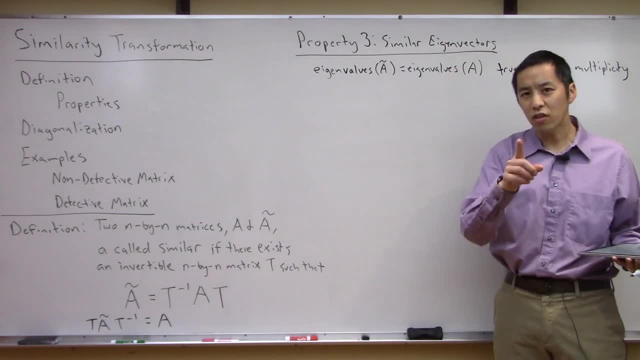 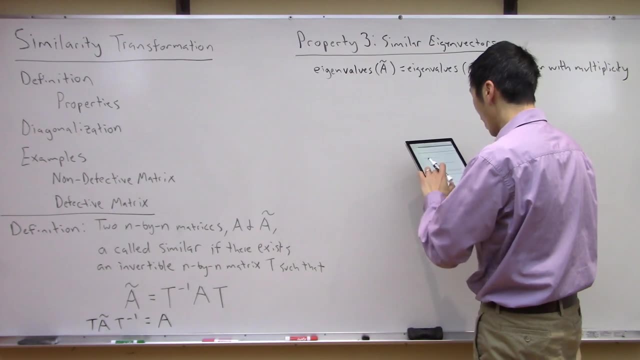 property number three looks at the eigenvalues of a tilde. So property number three looks at the eigenvectors And actually this is where it's not the same, but they're similar. So we're going to, we're going to take a look at that right now. So to do that, maybe what we should do is let's go. 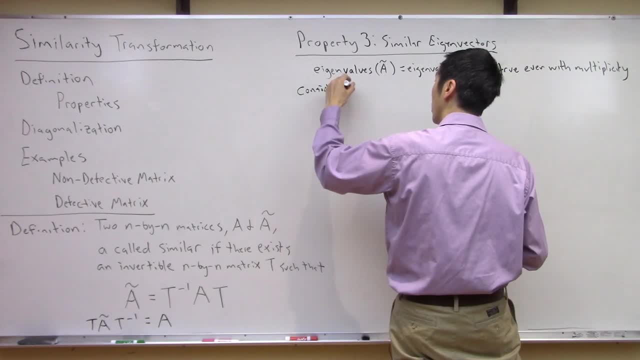 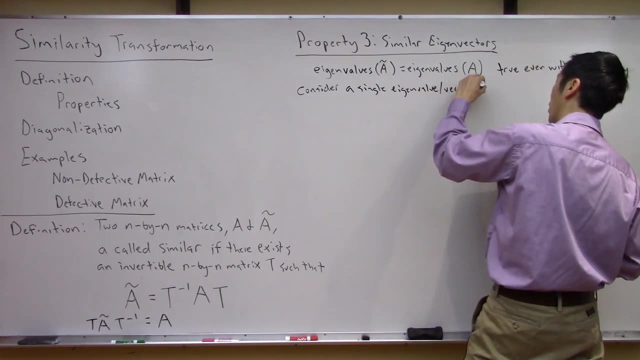 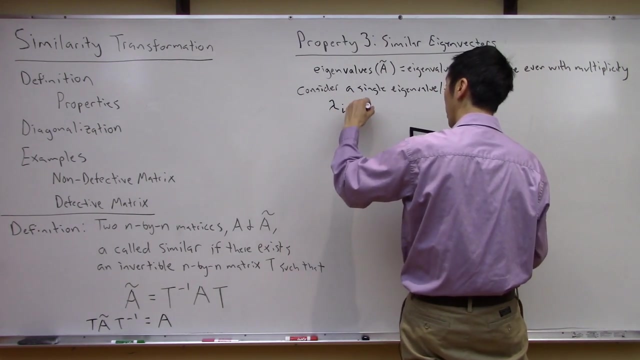 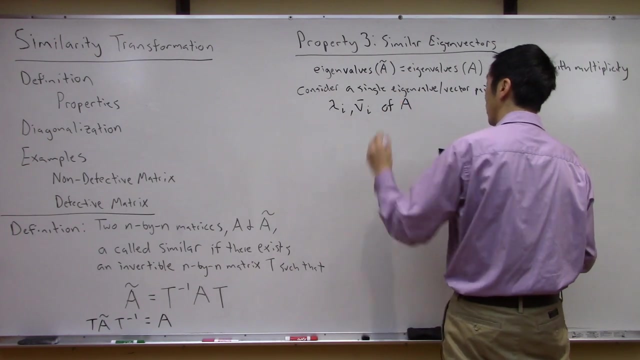 ahead and consider just a single pair, Consider a single eigenvalue, slash, vector pair, And I'm going to denote this as: how about lambda i and v? i? Right, So this is a, basically an eigenvalue, eigenvector pair of a- How about let's call this- of the original matrix, a. OK, So v? i. 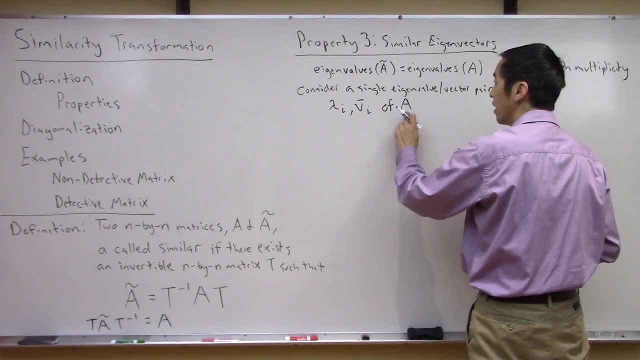 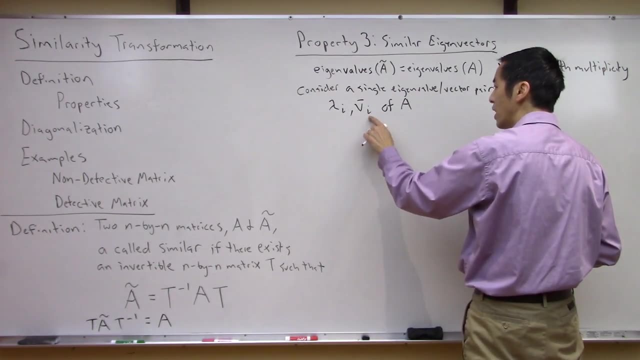 Again we saw lambdas don't matter, Right, The lambdas for a are the same thing as the lambdas for a tilde. OK, But v. I want to make the distinction here, that I'm going to use the notation v i to denote this is an eigenvector associated with eigenvalue. lambda i of the 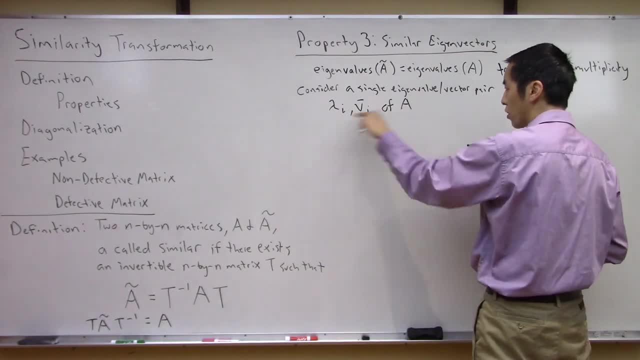 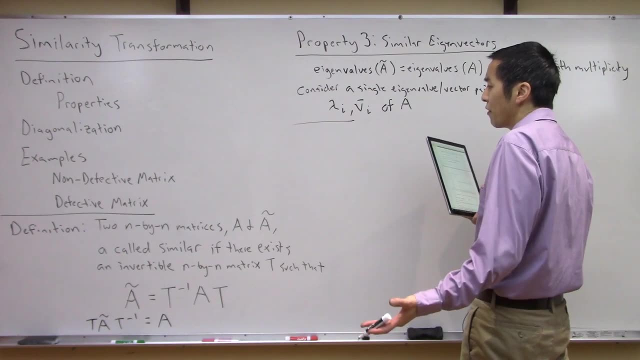 original matrix a. OK, So that's, we've got that on the board. So now let's go ahead and take a look at. well, how does this relate to to eigenvectors of? how about a tilde? OK, So let's just look at a tilde. 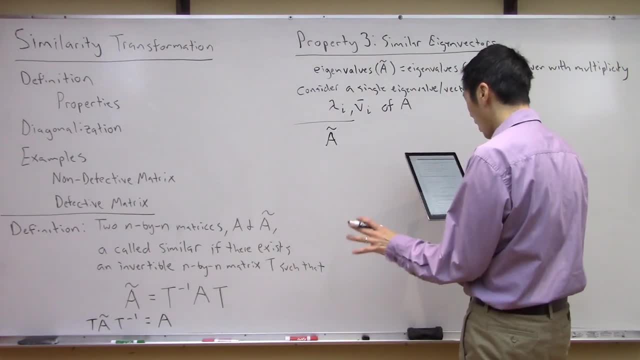 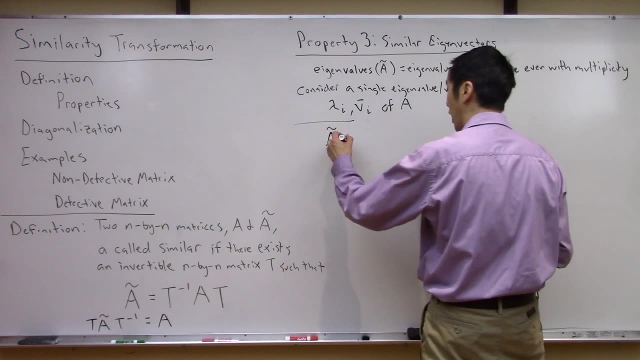 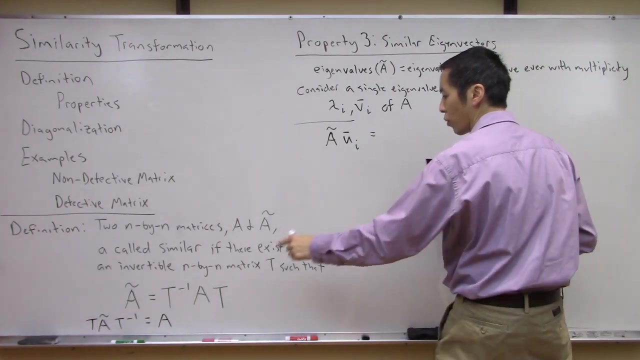 OK, OK. And what I want to do now is let's just multiply this by some arbitrary vector. How about u i OK? Now again a tilde. we said a tilde was. well, I guess we had it right here. Right, A tilde is t. 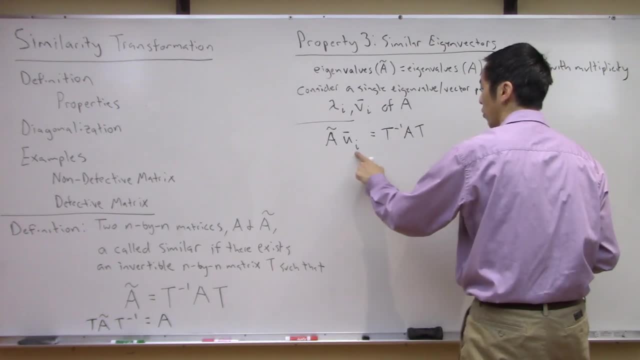 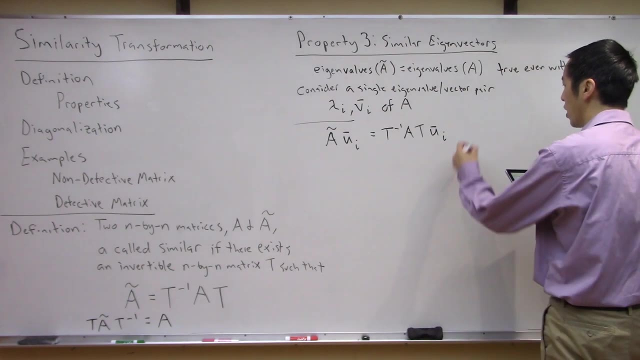 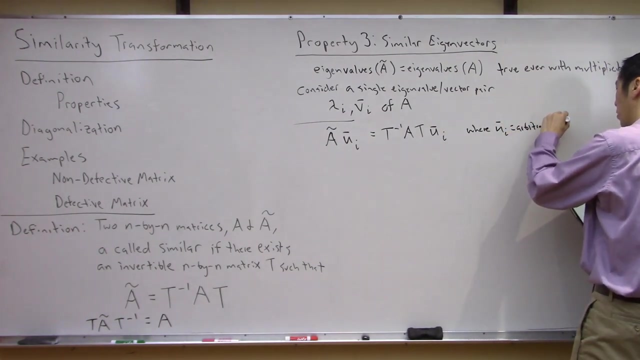 inverse a, t. So again, since I multiplied on the right by this arbitrary vector, I better do it over here as well. OK, All right. So again, this, this u, i is just some arbitrary vector. OK, Now, since it's kind of arbitrary, why don't we go ahead and make it equal to? let's just use? how about the eigenvector? 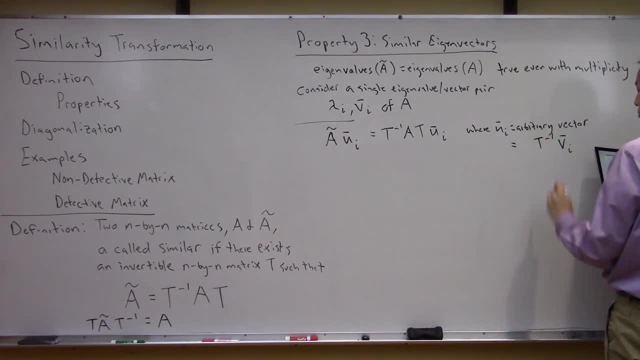 of a multiplied by t, inverse Right. Let's just pick this, OK. So this is going to be my my u that I want to multiply it by? OK, Great, So let's go ahead and substitute that in over here. So what do we end up with? We end up. 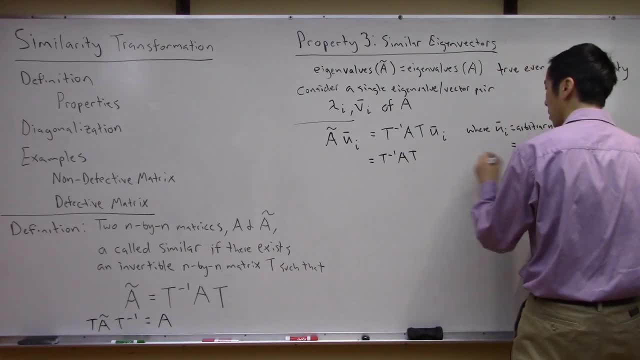 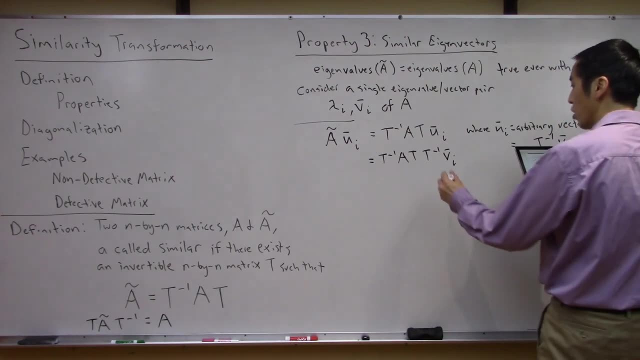 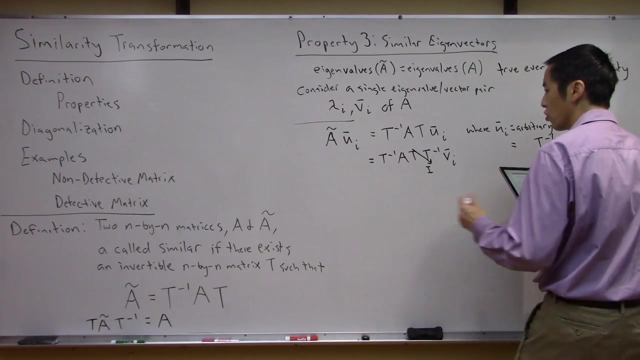 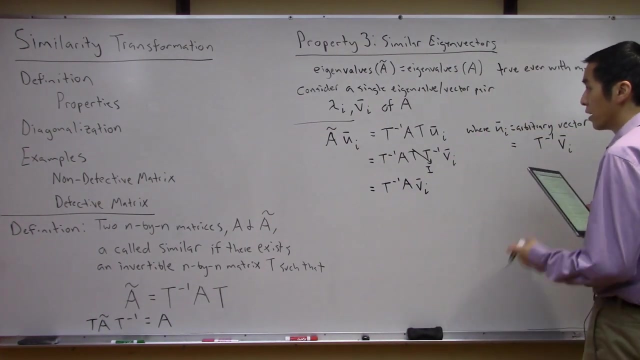 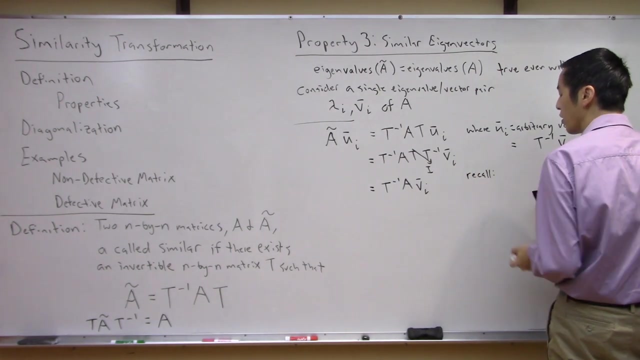 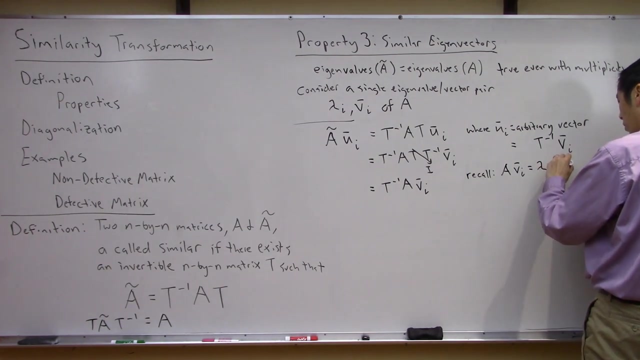 with t inverse a t times t inverse v i. Right, OK. So these here. basically, this is lucky. this becomes basically the identity matrix, Right? That helps us. So we end up with t inverse a v i. OK, Now you remember what's the whole deal. What is a v? i Remember the idea with an eigenvalue eigenvector. Right Is the definition of an eigenvector. is this Right? Because v is this magical eigenvector. If I multiply a by itself, I basically get the same eigenvector, just 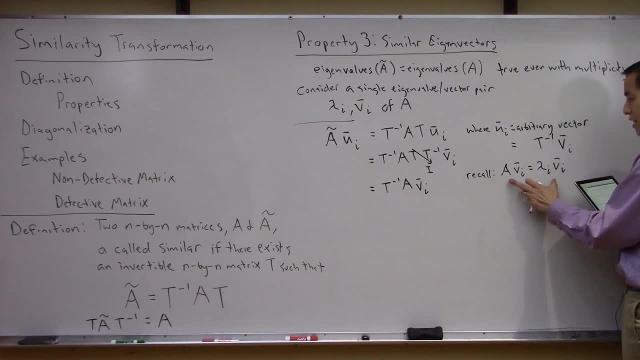 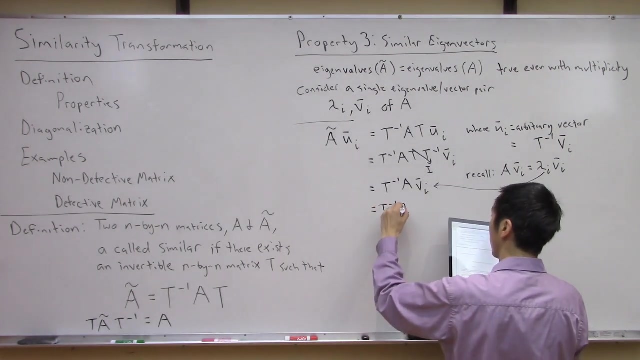 scale by the eigenvalue, Right. So this is again. this is the definition of the eigenvector lambda i and its associated eigenvector v i for the matrix a. OK, So great. This here. I can now just plug in this: a v i is the same thing as lambda i v i, So let's substitute this in for that, OK, So we end up with what the t inverse is still hanging around, and we now end up with lambda i v i. Right, And again now the nice thing about. 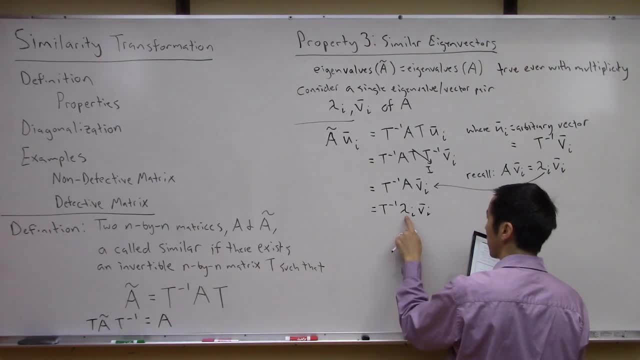 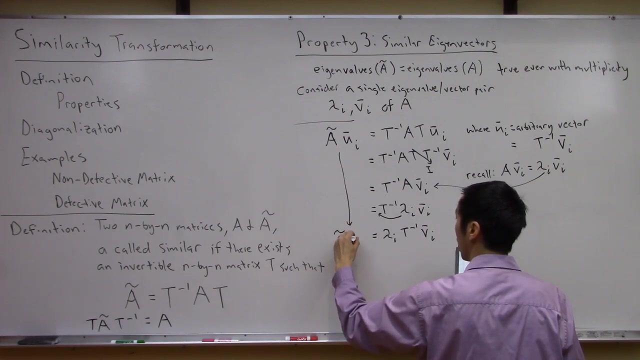 this is lambda i is just a scalar number, Right. It's not a vector, It's not a matrix, It's a scalar, So I can just move this to the front with no hassle. So this is the same thing as lambda i t inverse. v i Right, OK, And now tell you what? let's let's come over here on the on the left side. What was the left hand side? The left hand side is just. I haven't manipulated this at all, So this is still a tilde. u i Right, OK. Now look at this. u i here. 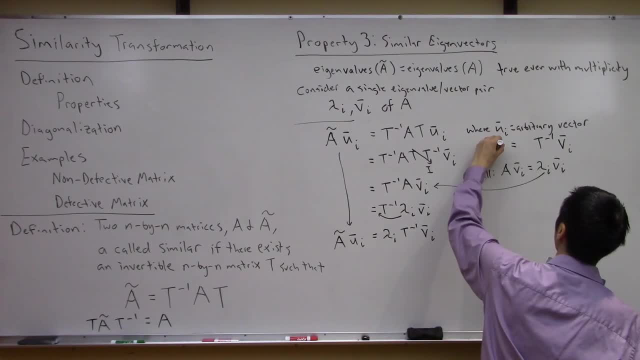 Remember what was u? i? U i was this up here, Right? This was u? i, Right, It's t inverse v? i. OK, So let's go ahead and plug that in for u? i. So maybe what I'll do is I'll just make a little note so we can recall what we're doing. So we're going to say: recall that u? i Right. This arbitrary vector that we're using it's, it's t inverse eigenvector v i, Right. So I'm going to plug that in over here. So we end up with a tilde. 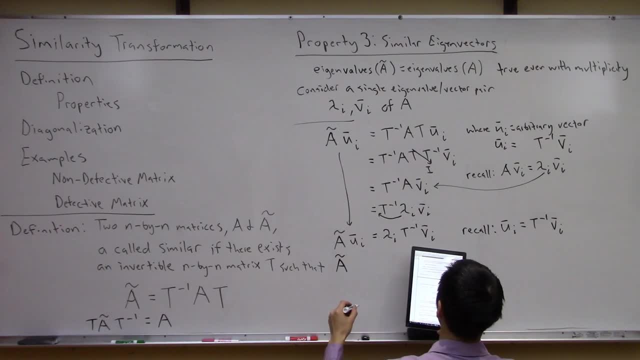 with Yeah, Yeah, OK, A tilde, A tilde, Sorry, Where, Yes, OK, T inverse v- i is equal to lambda i t inverse v i Right, Oh, no, Yeah, You know what I Actually wanted to do? I actually wanted to. I wanted to make it the other. Sorry, Sorry, Sorry, Let's. let's do this the other way around. This is the other way around It does. I wanted to keep the u here, So I wanted to make this a substitution. This thing right here, This is u i Right. Yeah, That that will That'll do better, Right, OK? So this thing right here, That's that's u i Right. So we basically have a tilde. 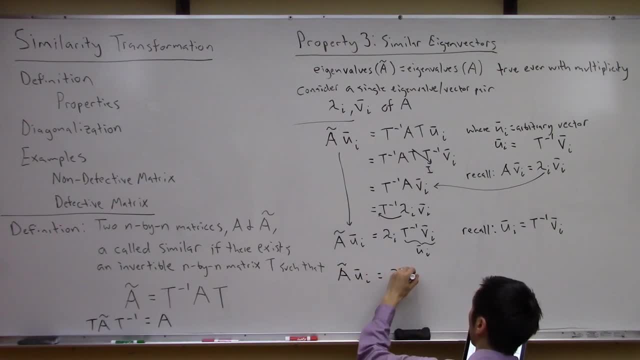 u, i is equal to lambda. i u, i, Right, Perfect. And this is perfect because if you stare at this thing long enough, Right, This is again. This is basically the definition of an eigenvalue, eigenvector pair for the matrix. a tilde here, Right, Because this is basically saying matrix times: some vector is equal to the same vector, just scaled by this. 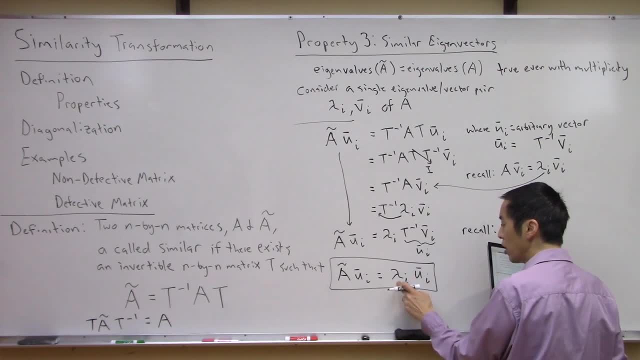 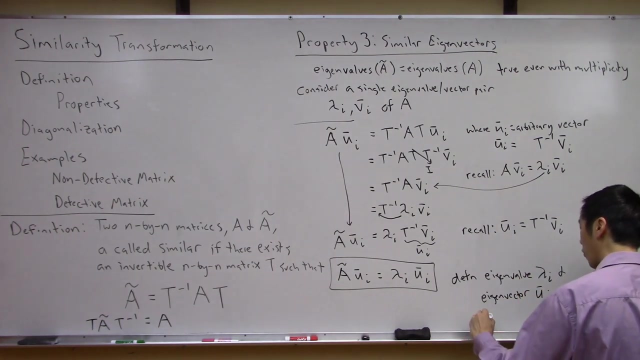 This, This value, the scalar- lambda i Right. So again, this is the definition of an eigenvalue, lambda i and eigenvector: u i Right For a tilde, for that matrix Right. So what we can deduce from this is the only you. This has to be an eigenvector Right. So we basically see that u i Right. 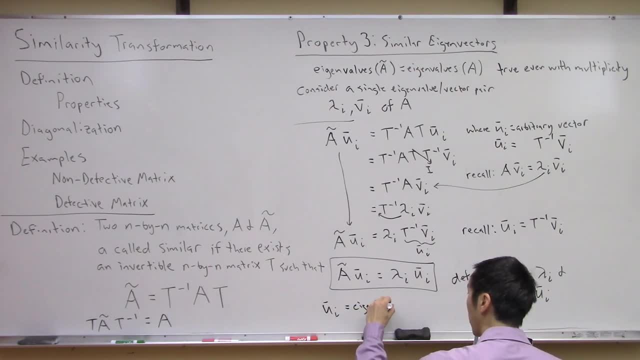 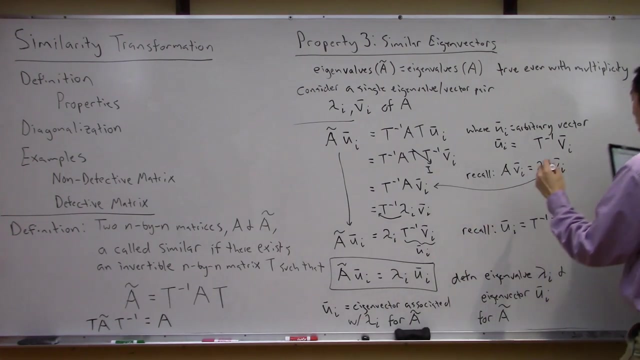 This is An eigenvector Associated With Lambda i For The matrix, a tilde Right. And again, What is u? i? So we see here That this Is how the eigenvectors Right. So we see this u. 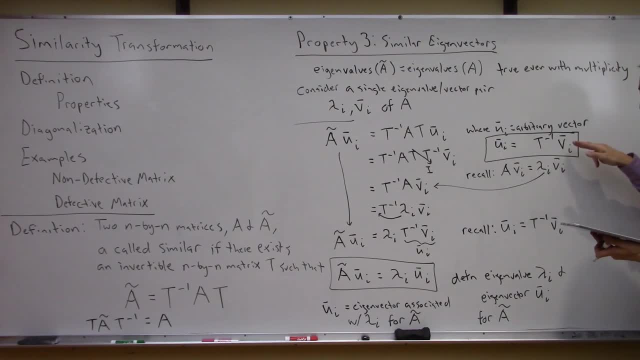 Is actually an eigenvector of a tilde And it's related to the eigenvectors of a Through this inverse matrix, right? so at the end of the day, what we end up with is a shoot. I ran out of room. I guess I can write it over here. so the end of property number. 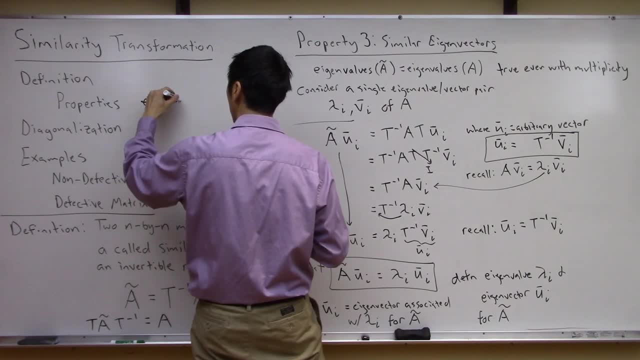 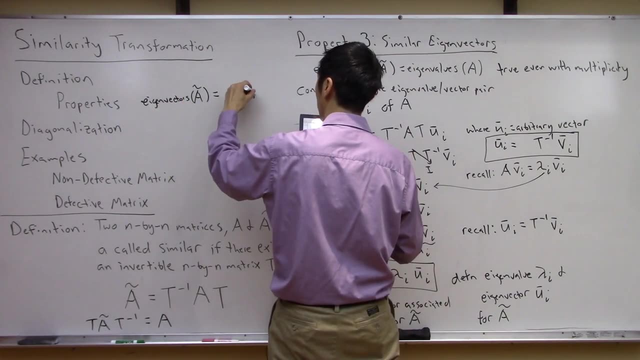 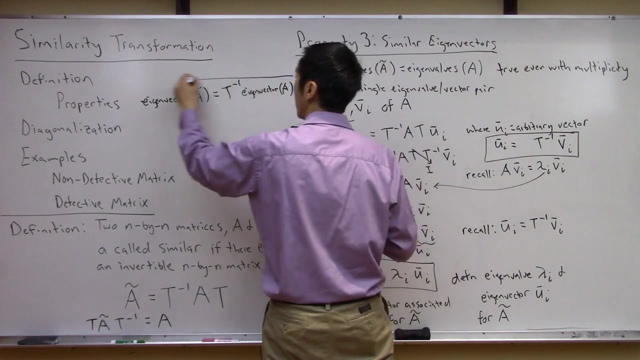 three is: basically it's the eigenvectors of a tilde are. basically they're the eigenvectors of a, but then you have to pre multiply by T- inverse right. so this is the takeaway for property. number three is that the eigenvectors of a 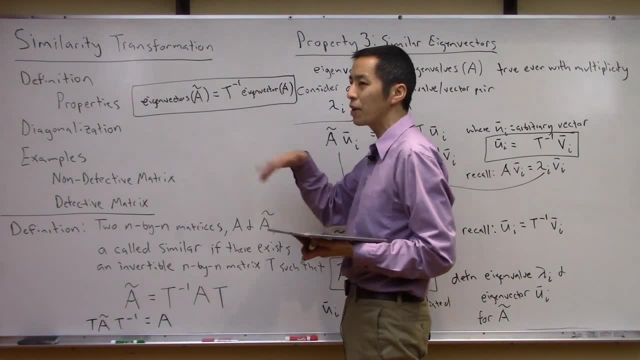 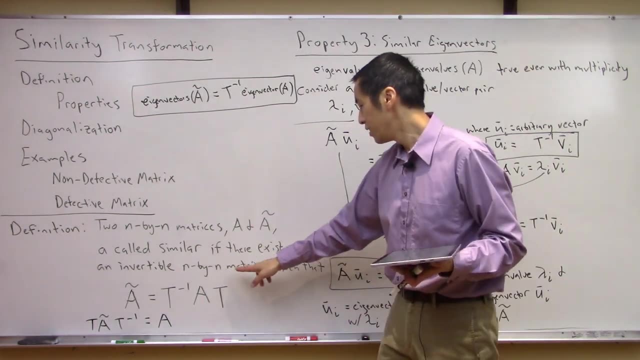 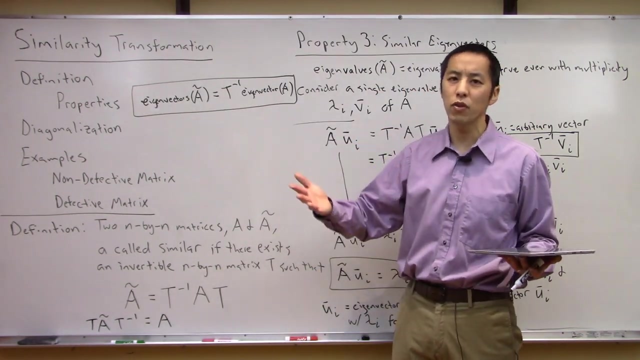 tilde are related or similar to the eigenvectors of a, but they're not exactly the same. there you need this T inverse and again, this maybe highlights the fact of why we needed T to be invertible, right. so again, as long as T is invertible. this is true and again should hold true, even if you have. 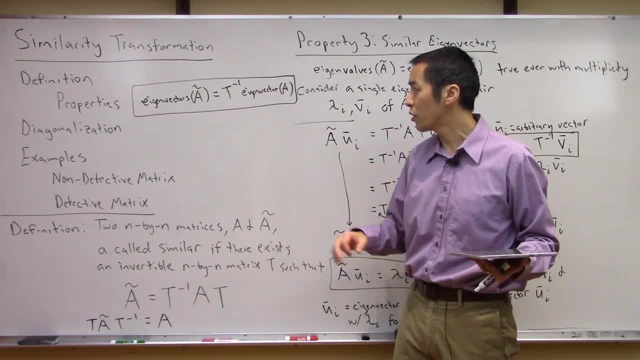 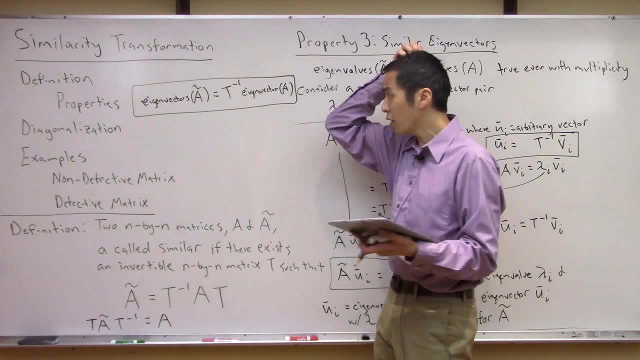 multiplicity of eigenvalues, right, so this is always how you can find the eigenvectors of a tilde. if you know the eigenvectors of a right, so great that is, that's interesting for this property. all right, give me a second. erase the board. let's move on, all right. 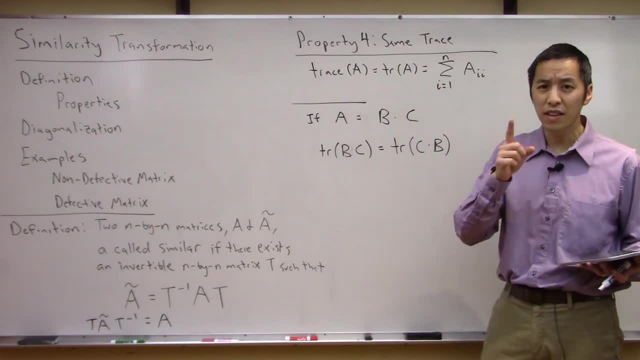 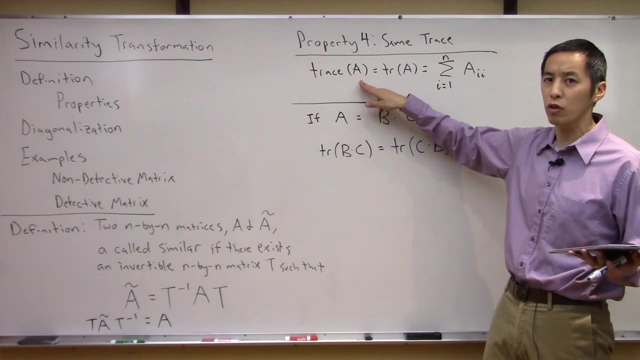 so property number four of similar matrices is actually: they have the exact same trace. now, remember the idea with the trace, the definition of the trace of a matrix, a. I remember again, we're talking about square matrices. it's just the sum of all of the diagonal elements, right? so you just basically take the one. 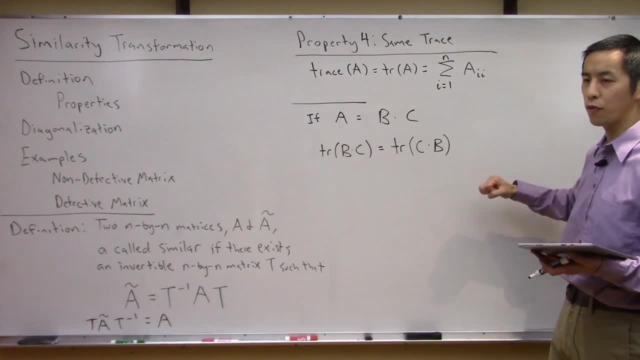 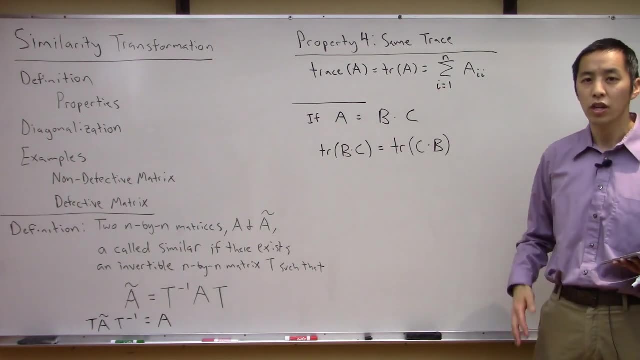 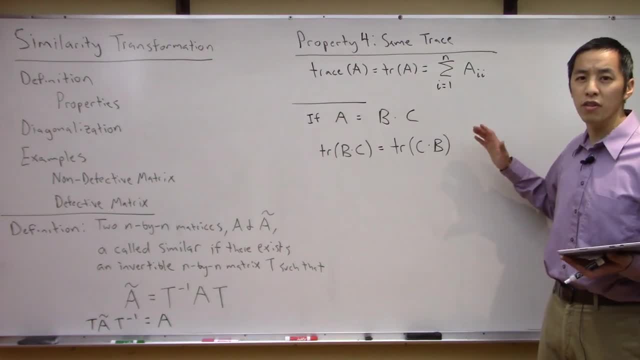 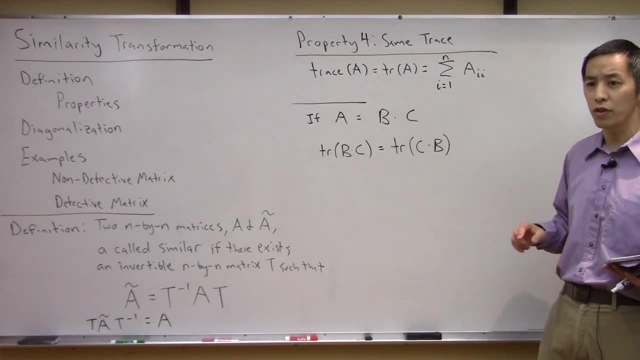 and again we are going to use some properties of the trace. I'm not interested in deriving those or proving those here, we're just going to use them. but we will apply them to our similarity transformation. so again, the property I want to use for trace here is that, again, if a is the product of two matrices, B, 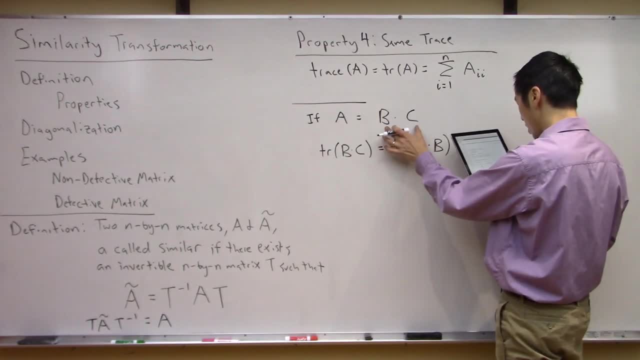 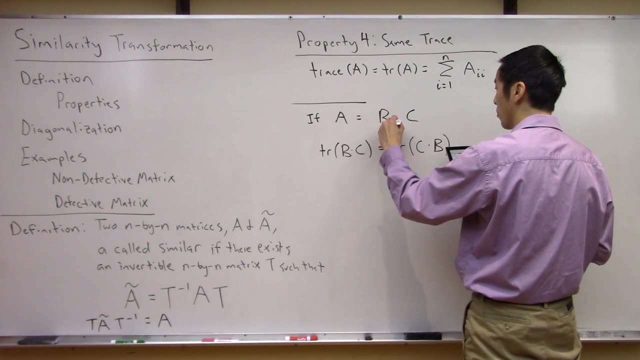 and C and actually these two don't even have to have the same dimensions. they have to have common matrices and they're not going to have the same dimensions, but they don't have to be the same. so, for example, B could be of n rows by m columns. 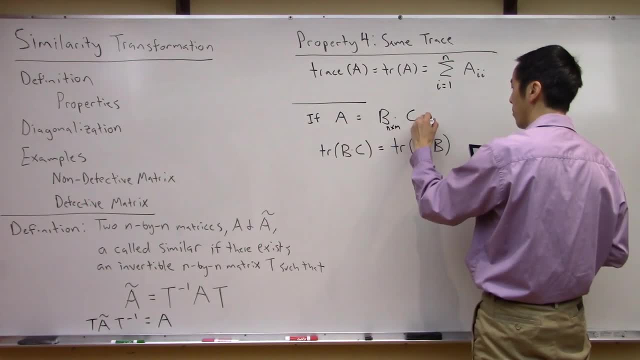 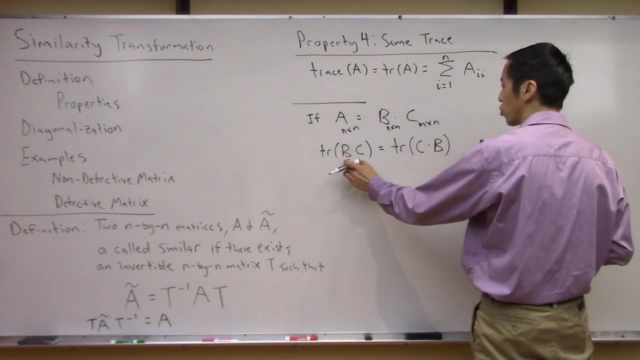 and C. I guess, in order with this, better be m by n, right? so at the end of the day we have an n by n matrix a. okay, so if we're looking at the trace of B times C, right, that's actually the same thing as a trace of C times B, obviously again. 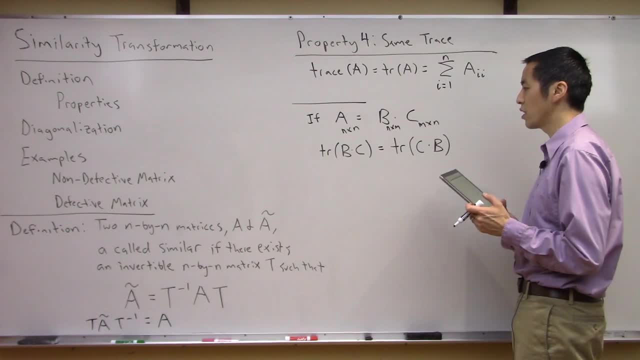 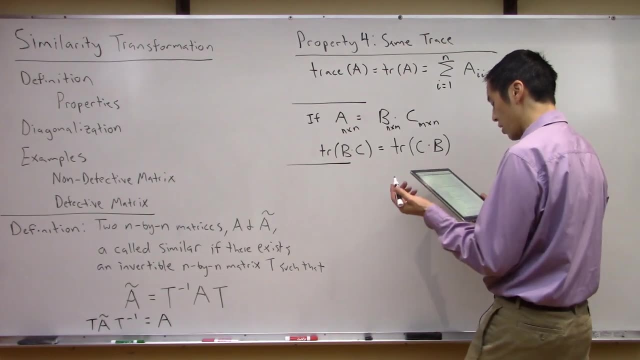 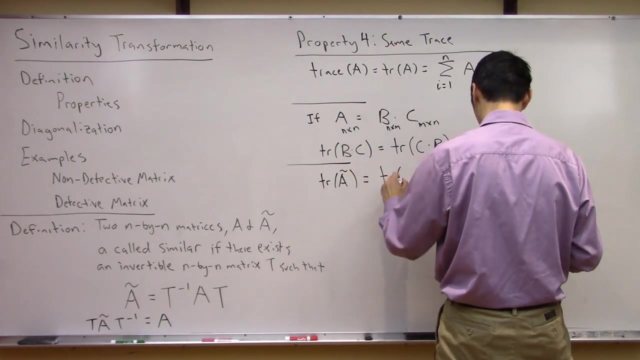 this times its matrix multiplication, right? as you can kind of clearly see here. okay, so that's the property I want to use. let's go ahead and apply that to our similarity transformation and see what we end up with, right? so let's go ahead and compute the trace of a tilde, right? so again, a tilde, right? we said was: 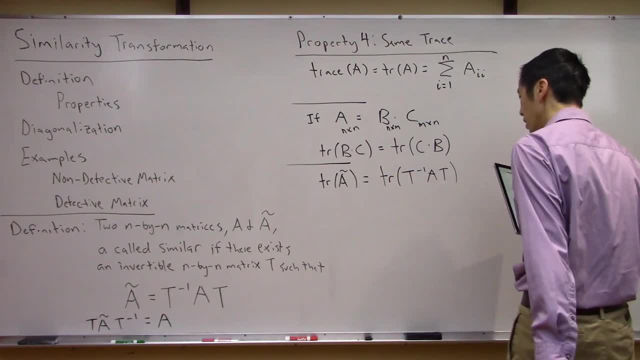 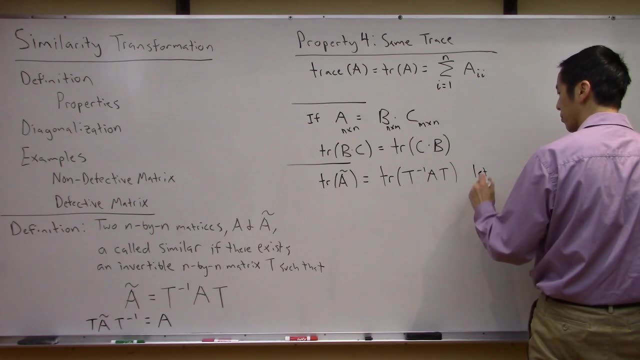 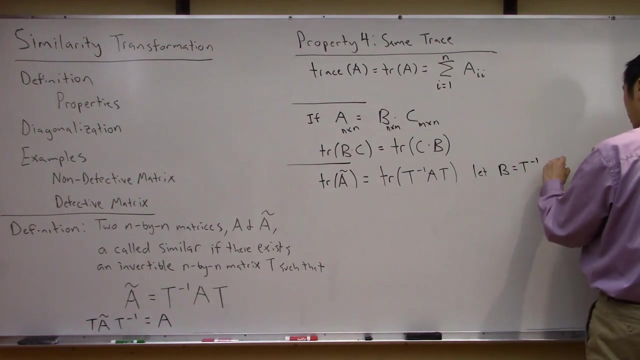 just T inverse, a T, right? so let's break this up into two steps, right? so let's go ahead and make a substitution. let's go ahead and just say: I'm going to call this matrix B as just T inverse and let's call the matrix C as sort of a. 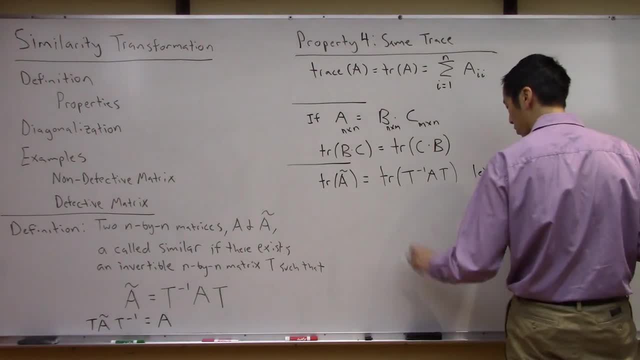 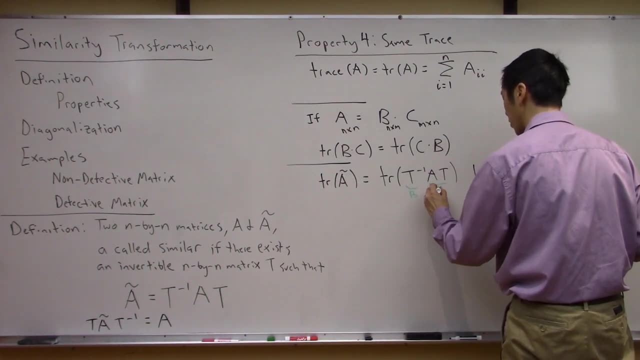 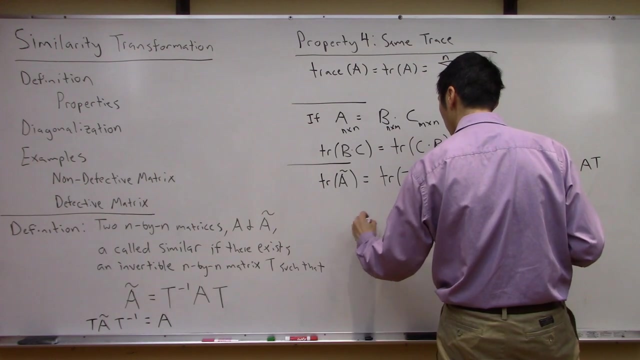 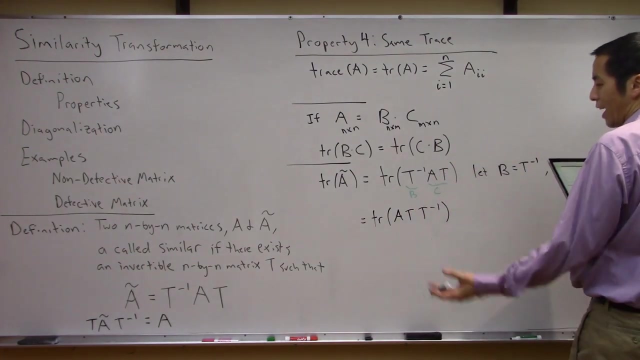 product, this matrix AT, right. so this bit right here, let's just call this matrix B and let's call this matrix C, right? so then using our trace property, where I can basically just flip the order of these matrices, right, we end up with this is the same thing as trace of AT, times T inverse right, and then this is super. 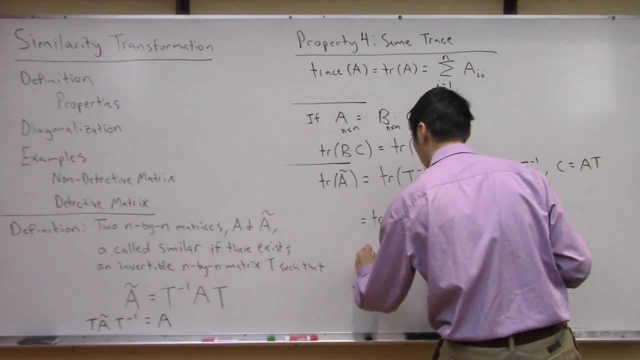 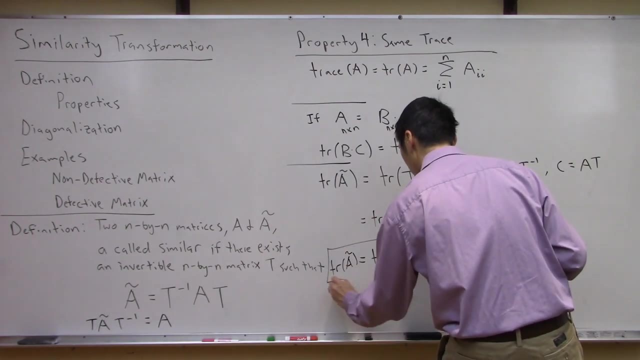 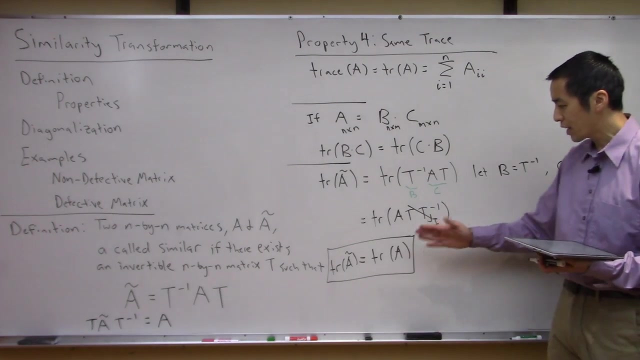 easy, because now this becomes an identity matrix and we basically end up with just trace A right. So we see that trace of A tilde is the same thing as trace of A. So again, pretty interesting, We see that the trace of the matrix, again, is not changed under a similarity. 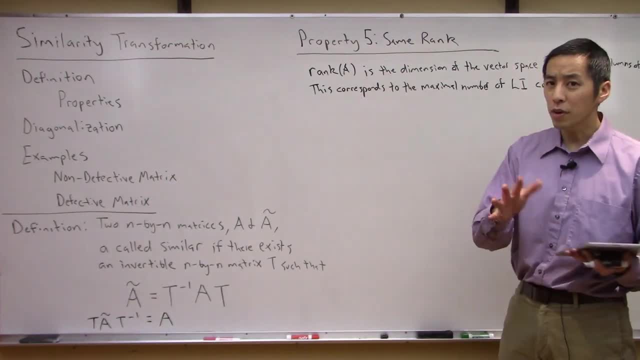 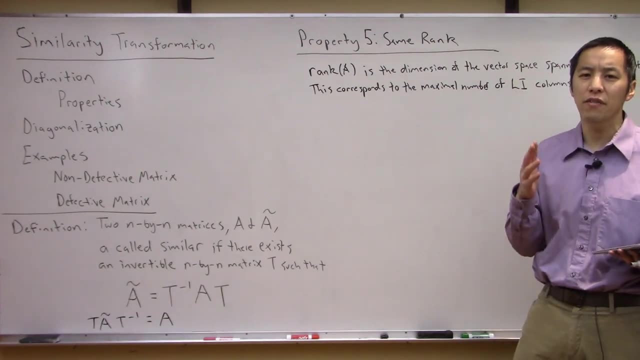 transformation. All right, so with property number five concerns the matrix rank right, And we're actually going to see that again A and A tilde have the same matrix rank. So again, just to refresh your memory, the idea with the rank of a matrix right is it's basically the dimension. 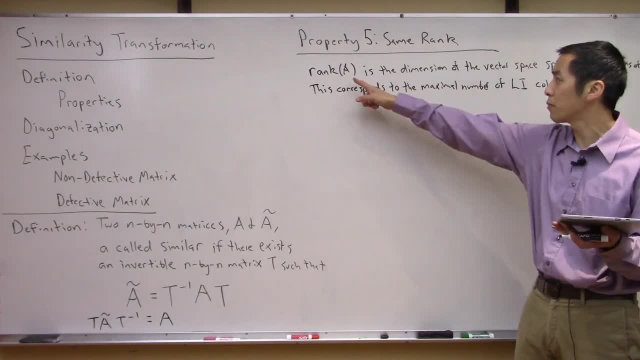 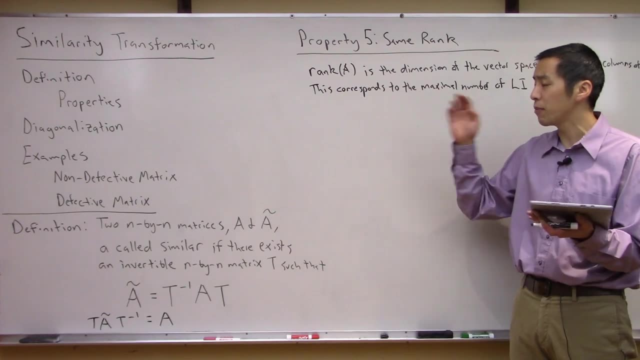 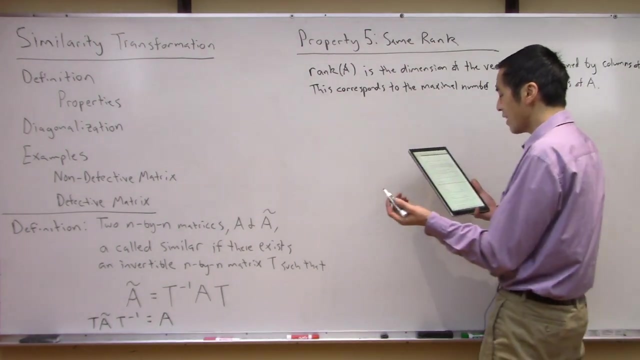 of the space spanned by the columns of this matrix A right. And again, the other way to think about that, it's the number of the maximum number of linearly independent columns of the matrix A right. So if we take that perspective of what the rank of the matrix is, you can see that basically. 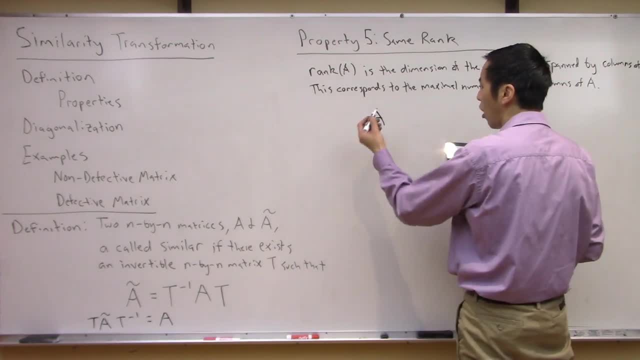 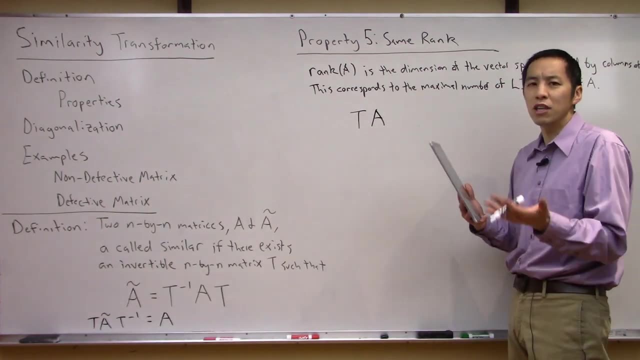 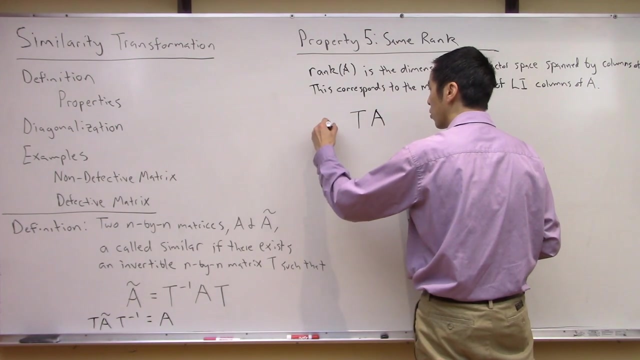 if you have a matrix, A right and you operate or transform on this by some invertible T right, You're basically not changing the number of linearly independent columns of that matrix right Because T is invertible right. So basically you can see that the rank of this 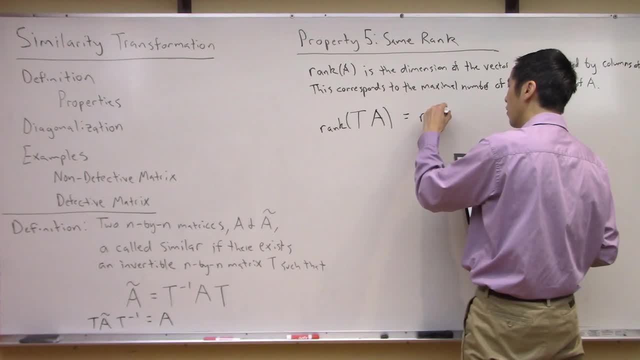 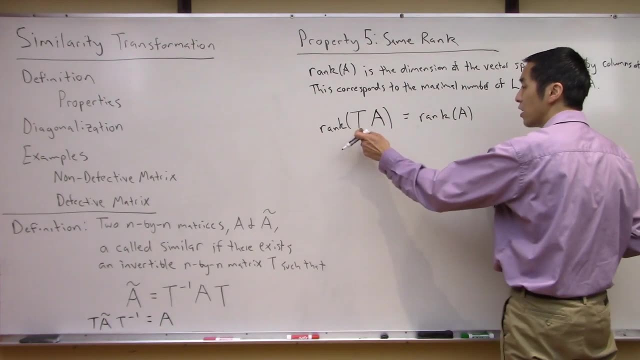 thing is the same thing as the rank of A, right? You haven't changed the rank of it by multiplying by an invertible T, And, in fact, the invertible T can be on this side or it can be on the other side, right, It doesn't really matter. In fact, here, let me do this, Let me write this. 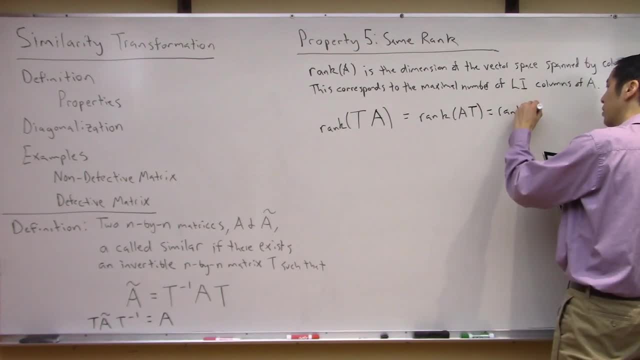 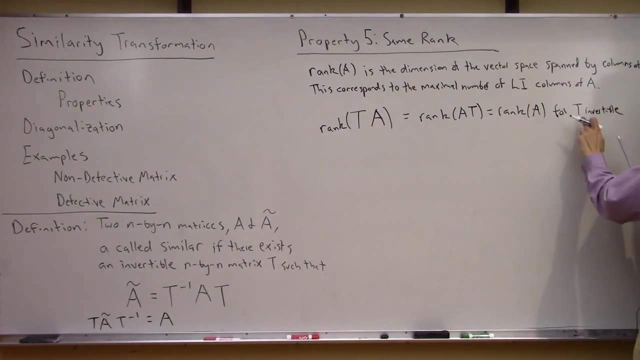 Right, All of these are the same thing. right For T, invertible. right, Because that's the whole idea, with invertible means that T is full rank. right? It doesn't. it's not singular, it's full rank. So it's not going to change the number of linearly independent columns of the matrix A by 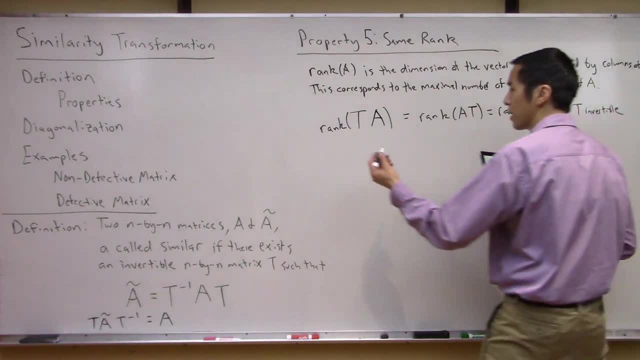 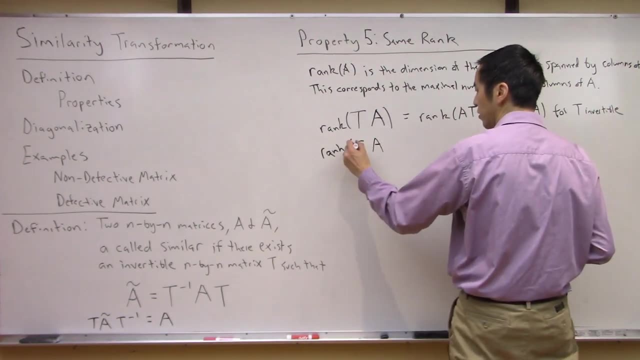 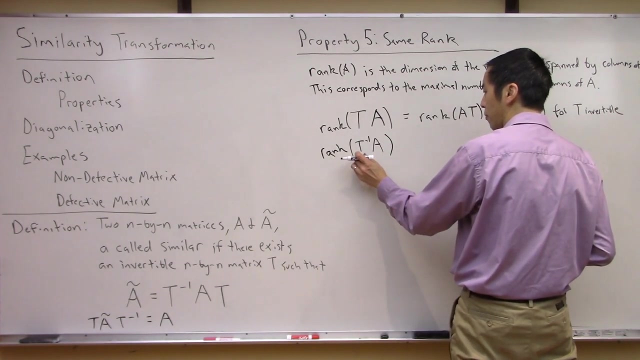 just multiplying, right, And in fact you can think about this the same way of you know. again, you have A. here's another invertible matrix. How about T inverse? right, Because T is invertible. T inverse is also invertible, So it's the same idea, right? I've got an A, I've got some. 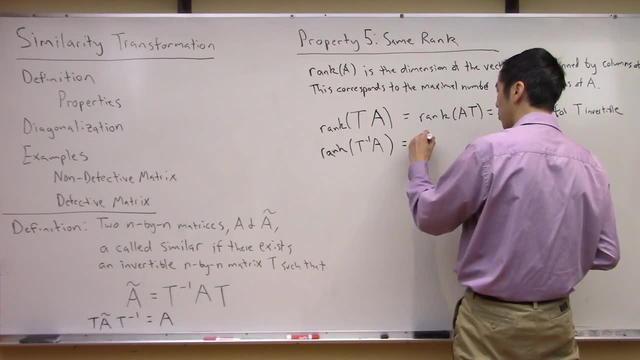 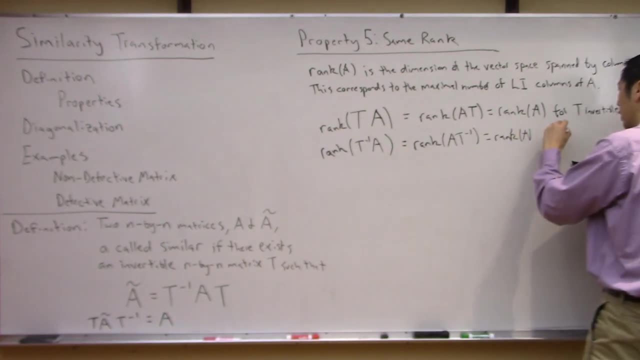 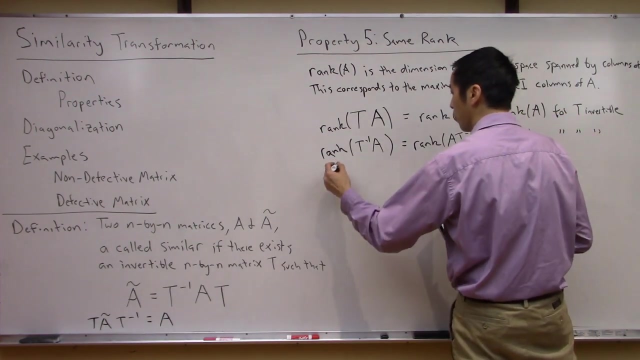 full rank matrix that I'm multiplying it by. So again, I can multiply it by that on either side right, And you still end up with rank of A right Again for T, invertible right. So again, let's go ahead and we'll put these in the bank. 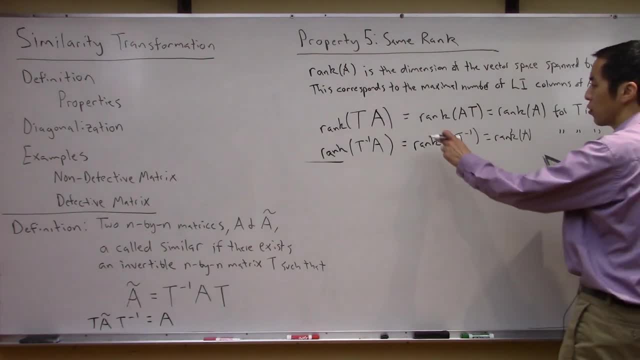 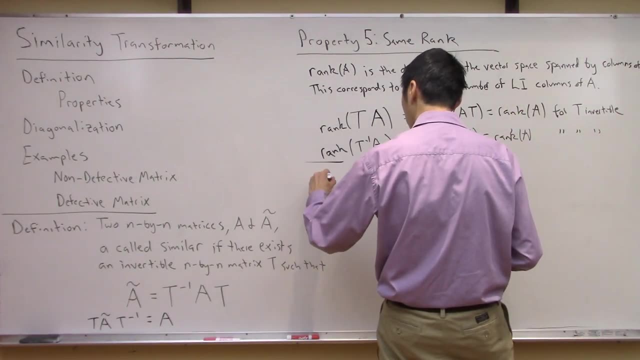 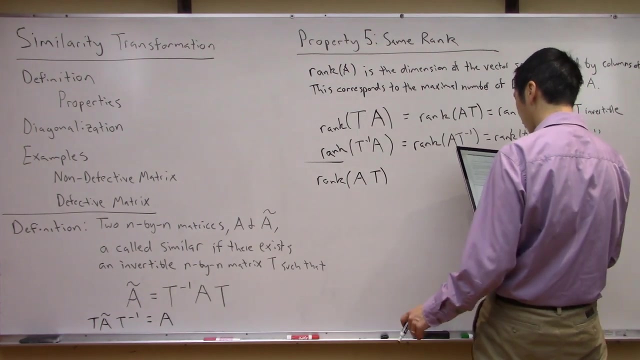 Right. The other way that we could prove this, if you want to make sure that this is true, right- Is, again, we can use the property of matrix rank. that says that the rank of A times any matrix T- right Again. let's forget about T being invertible, for now. 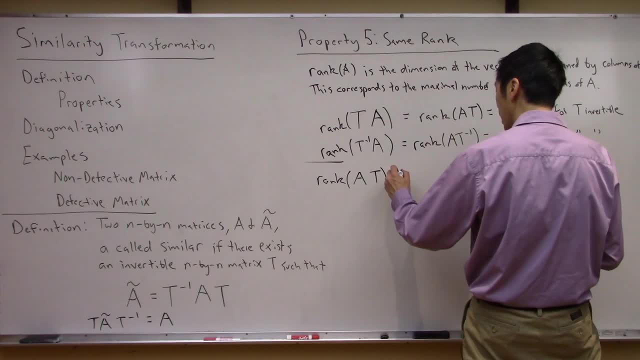 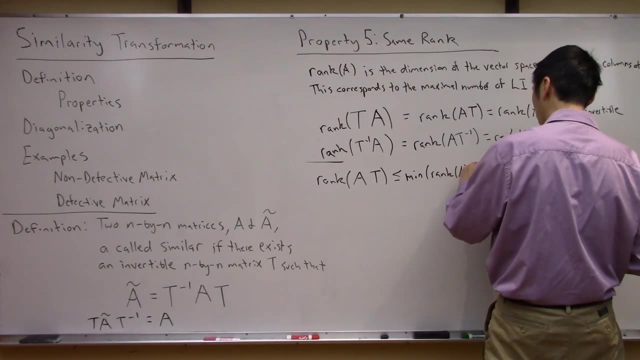 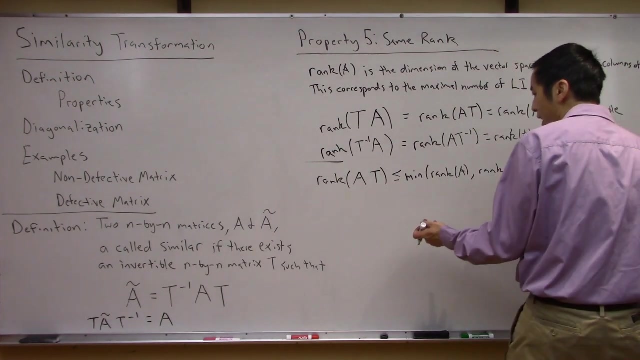 but this is the product of any two matrices. If you take the rank of this, this rank has got to be less than or equal than the minimum of the rank of A and the rank of T. Right, So we can know now if T is invertible. Well, actually, maybe tell you. let me take away. 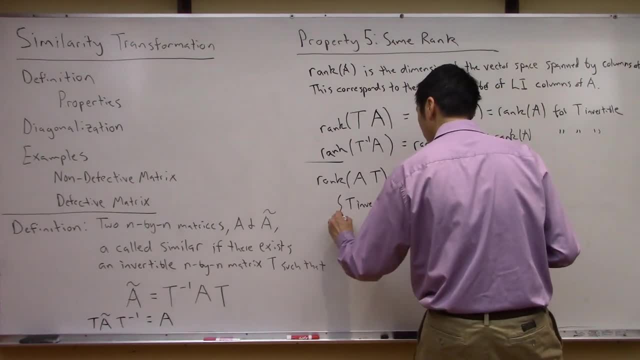 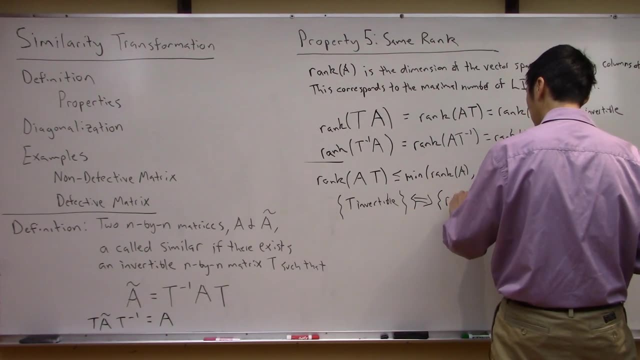 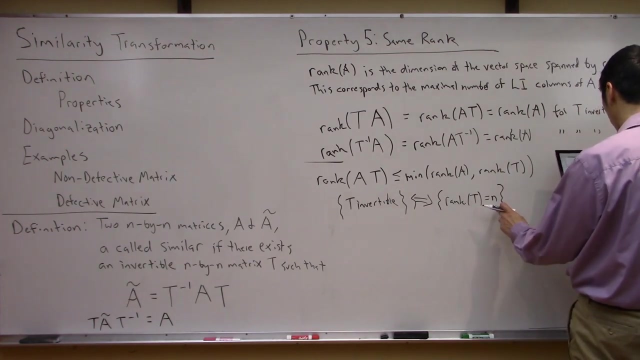 the if right, Let's just make the statement that right, If you have T invertible right. This basically only happens if, and only if, the rank of T right Is equal to the full dimension of the space, right. So this is only happens if rank T is equal to N for our square. 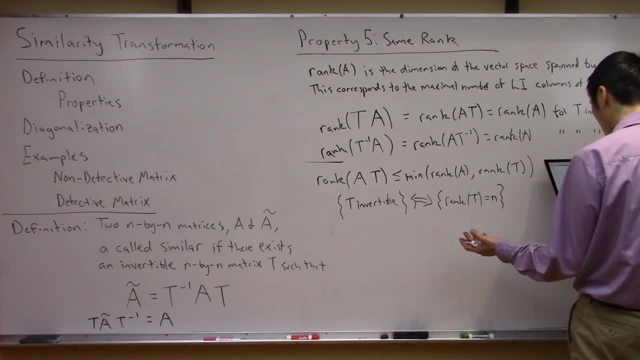 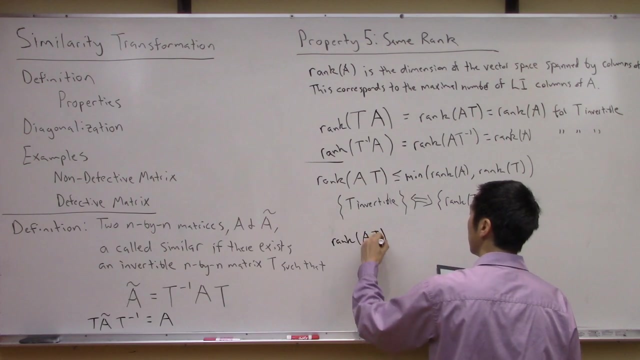 matrices, right. So therefore, I think if you look at this minimum, you know that this has the rank of T has got to be greater than or equal the rank of A. So we can basically write that if T is invertible, we have rank of the product A, T. it's got to be less than or equal to the rank of A. 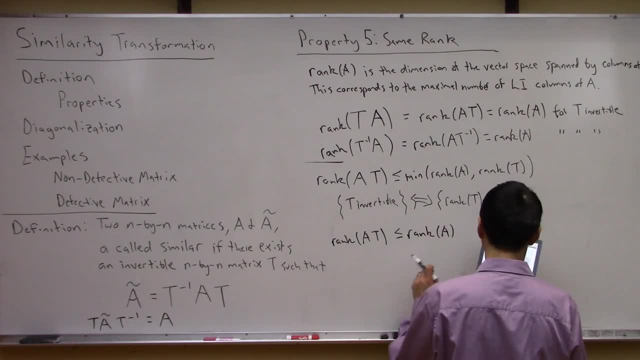 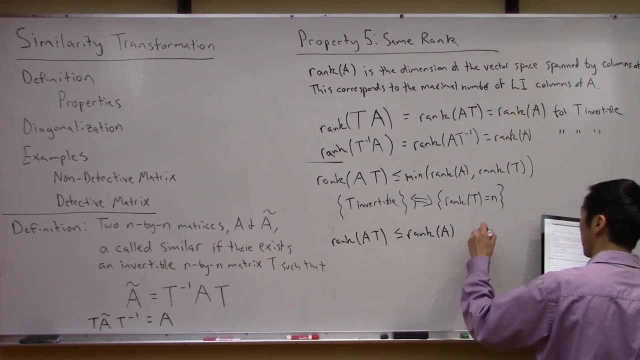 Right, And let's tell you what: let's, let's, let's. I don't want to box this, but maybe we should star this or number this In my notes. I've got this as equation 6B. Let's just use my same numbering, so we don't. 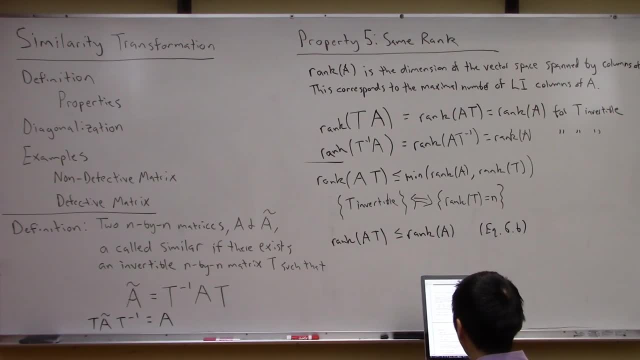 get mixed up And I could basically, you know we could, we could, we could do a very similar thing. Let's just actually use 6B again, but let's go ahead and change the matrices. So I'm going to. 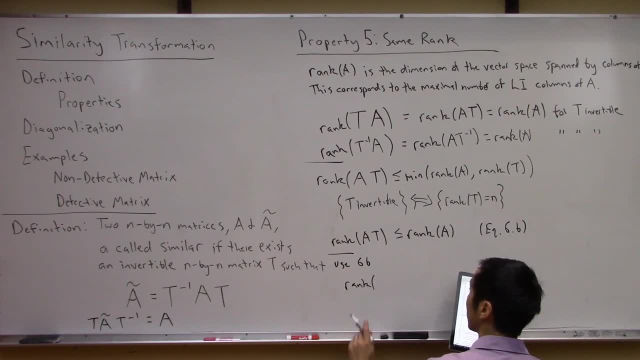 look at the rank of a product of two matrices. Let's just, instead of A, let's turn this into the product A, T, And instead of T, let's turn this thing into T- inverse, Okay, So what I mean by that is: now we have the rank of the matrix. 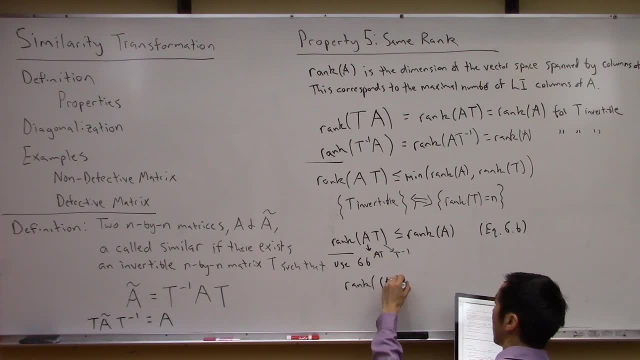 this thing: A T right, That's that one times T inverse right. This thing has got to be less than or equal than the min of the rank of A T right And the rank of T inverse right. Okay, So again this we can write the left-hand side. This is basically going to be rank of A. 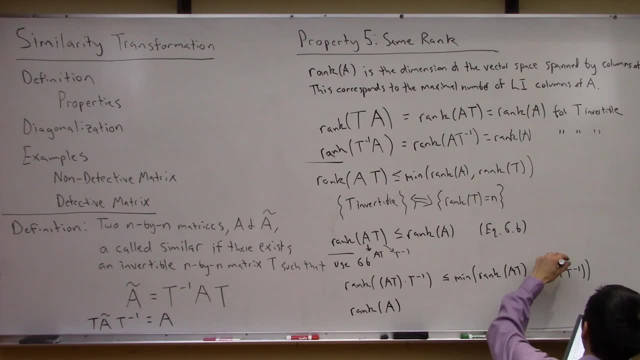 right. And again we see that this here is full rank, right. So rank of T inverse: because T is invertible, T inverse is a full rank, So we can write the left-hand side. this is basically going to be: T inverse has to be invertible. So the rank of T inverse: this has got to be N, So this has got to. 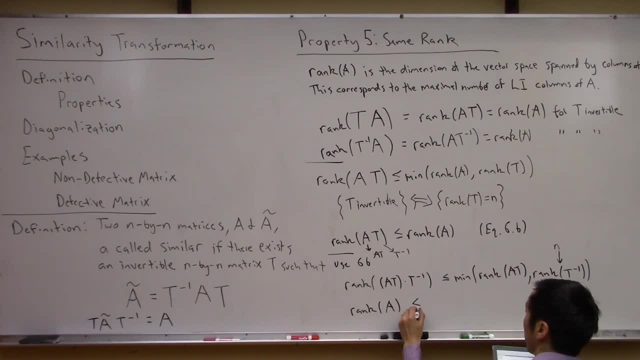 be bigger than this. So we basically have this: has got to be less than or equal to the rank of A, T, right? Okay, So that let's call this equation. how about 6C? right, If you look at equation 6B? 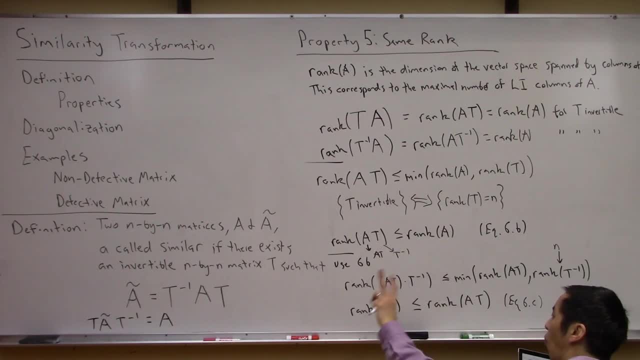 and equation 6C. you see, the only way these two are satisfied simultaneously. right Is if the rank of A is equal to the rank of A, T. right Because it's on the opposite side of the less than or equal sign on both sides. So basically combined. 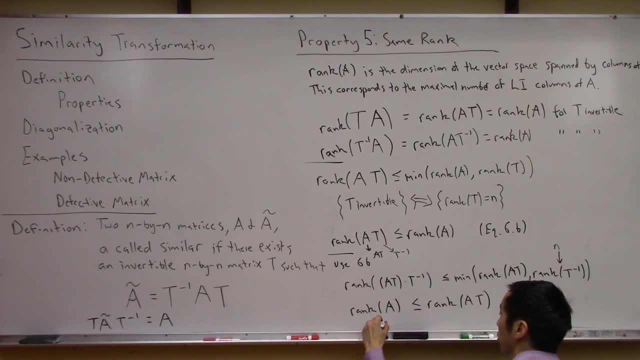 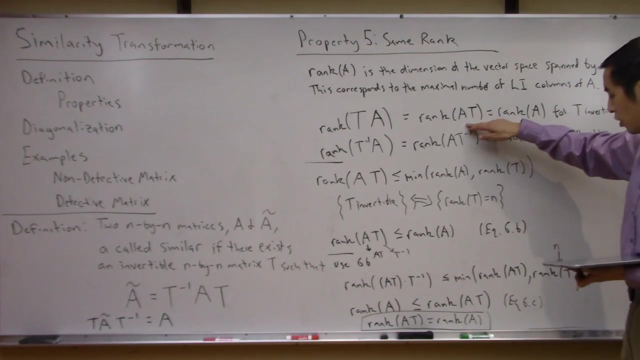 6B and 6C and we end up with, basically, the rank of A- T has got to equal the rank of A right. And again. this is exactly what we did up here And again. you could do the exact same thing for TA, which is this part of it, And again. 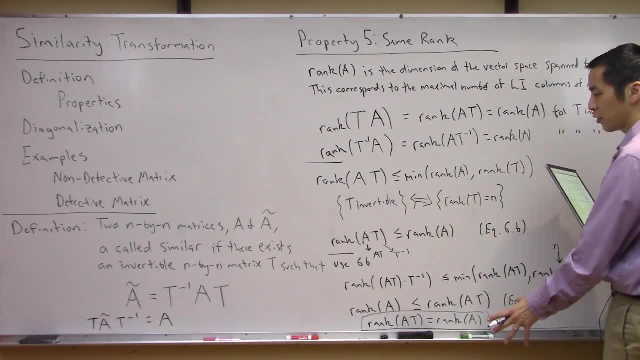 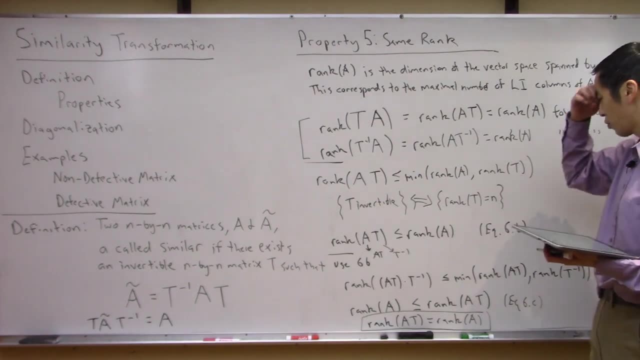 you can do the same thing with T inverse. So again, this discussion here- if you glossed over that- is basically just to get us and convince ourselves in the head that these two things are true. And I know I said we wouldn't try to prove too much of this, but I think this is maybe. 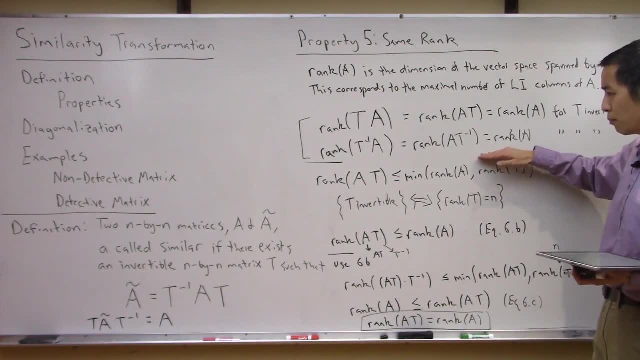 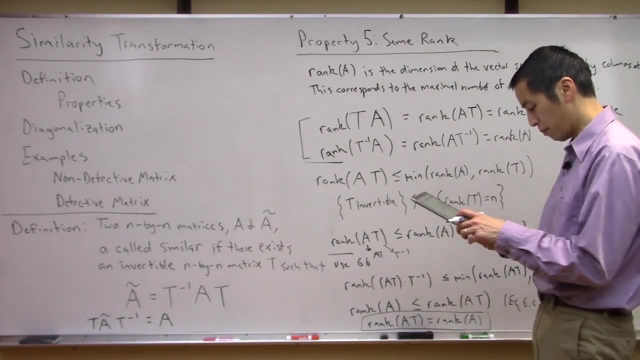 somewhat useful here, because now it kind of gets us in the mood for applying this result up here to our similarity transformation. So, uh, yikes, I'm kind of running out of space. Um, let's, let's come over here, How about? okay, so let's go ahead and look at now, how about what? 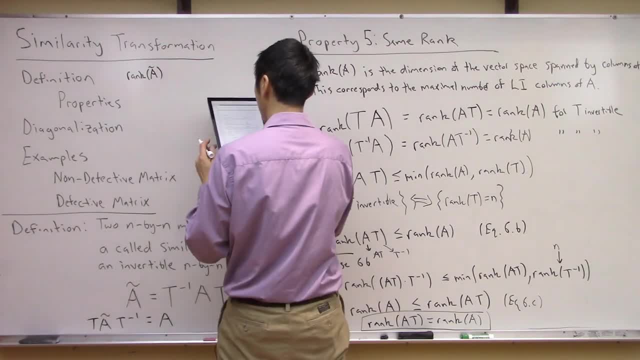 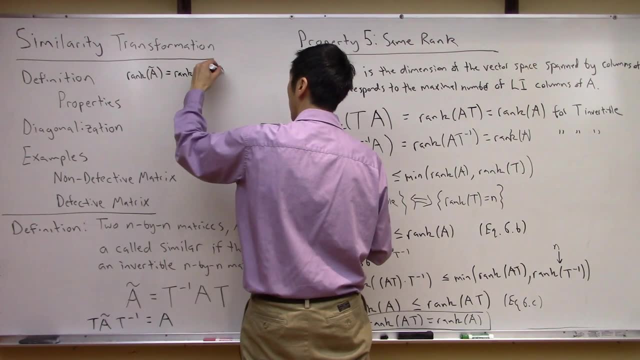 what is the rank of A tilde? right, So the rank of A tilde is basically: well again, what is A tilde? A tilde is just T, inverse AT right. Okay, So tell you what. let's again break this up into. 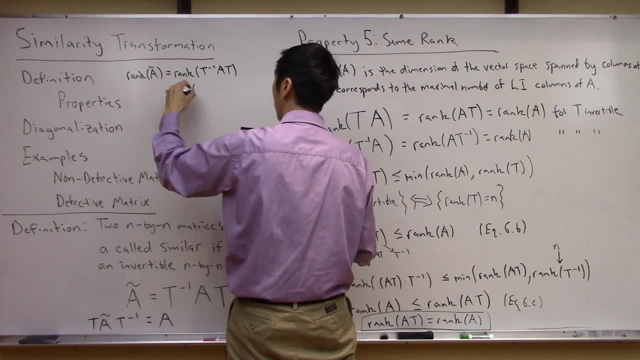 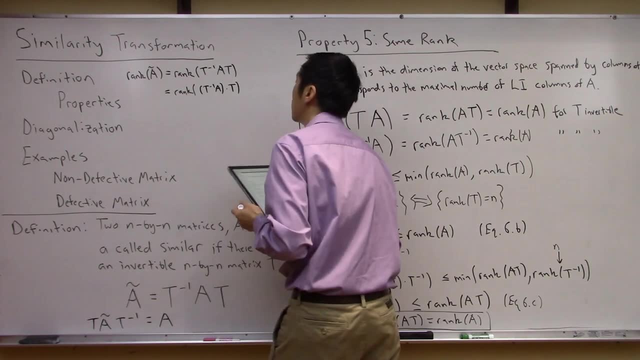 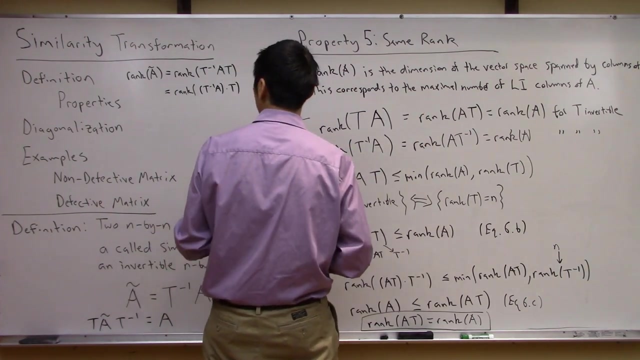 the product of two matrices. How about the rank of let's group? uh, let's do T, inverse A as one matrix And then times T right Now, pursuant to this set of equations, right where we basically see that. 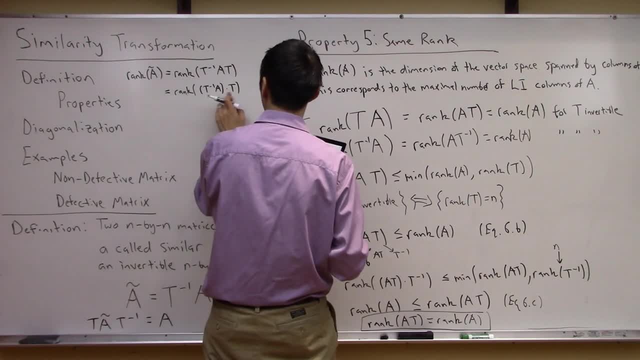 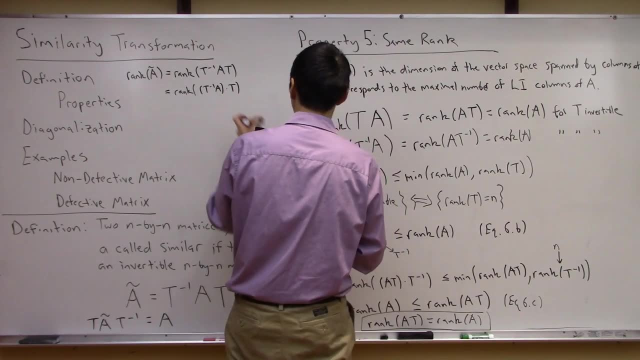 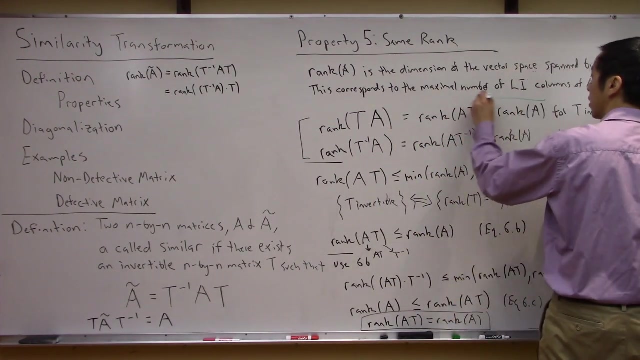 uh, again, this is the product of two matrices And this is something here times T, which I know is full rank right. So this is basically. I'm going to use this portion maybe, so let me circle this in green right, Where the rank of some matrix times an inverse right. So this is the 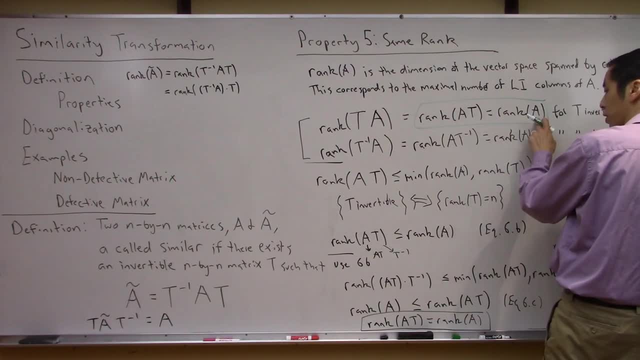 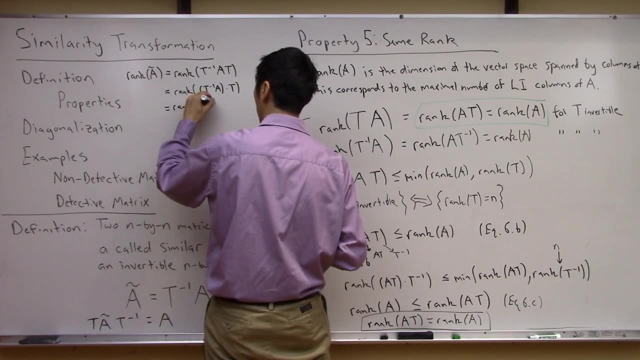 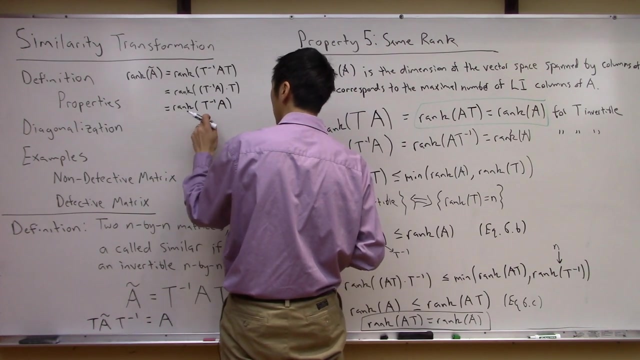 invertible full rank. T is basically the rank of that original matrix, right? So this thing can be basically be written as rank of just T, inverse A, right, It's just the matrix thing in parentheses, right? And now this is the exact same thing. You look at this and we say, okay, this is a product. 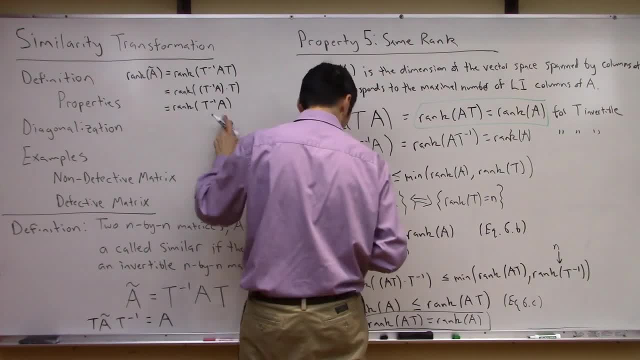 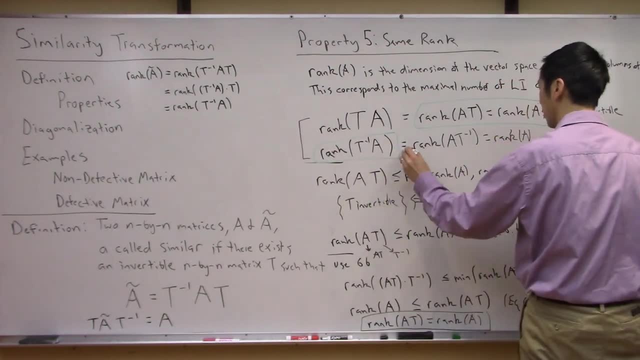 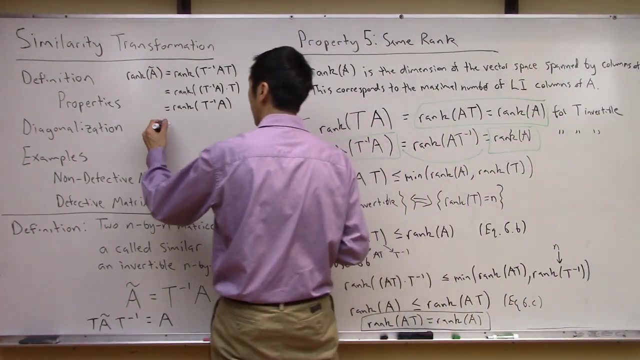 of two matrices. It's an invertible matrix times A. So again you can kind of come over here and we can say this part- uh, sorry, I should have put right This T inverse A is basically the same thing as rank A, So this is basically just rank A. 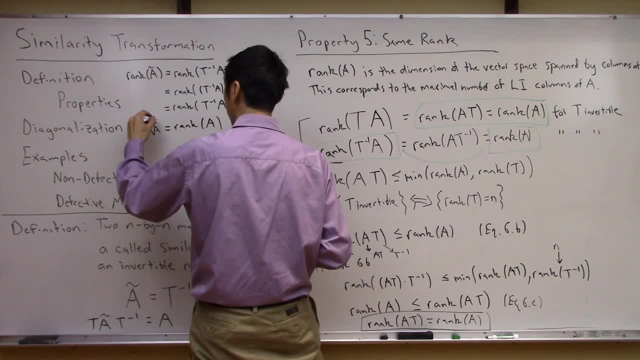 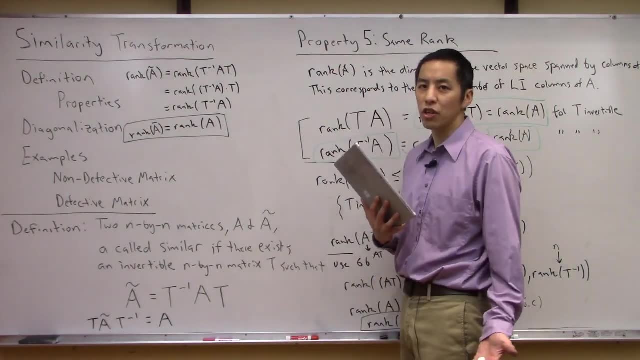 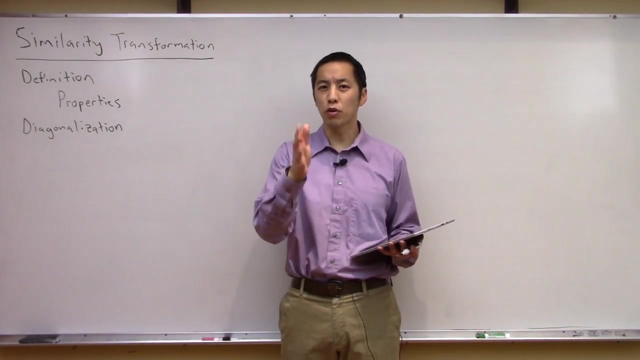 So here you go. We end up with rank of A. tilde is equal to the rank of A. So we see again. the rank of the matrix um is unchanged underneath a similarity transformation. All right, So that was great. We saw that way. Similarity transformation preserves a lot of. 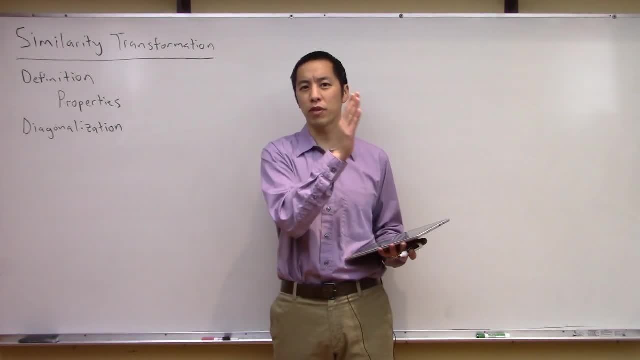 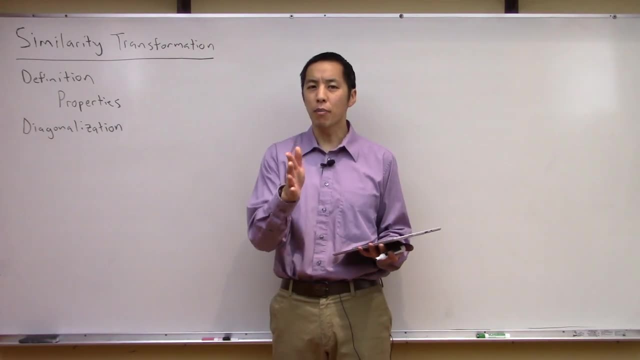 properties between the matrices. So we're going to go ahead and do that. So we're going to go ahead and look at the matrix A and the transformed or similar matrix A, tilde, with the exception of the eigenvectors, which we saw were somewhat similar and related. Um, now, remember those properties. 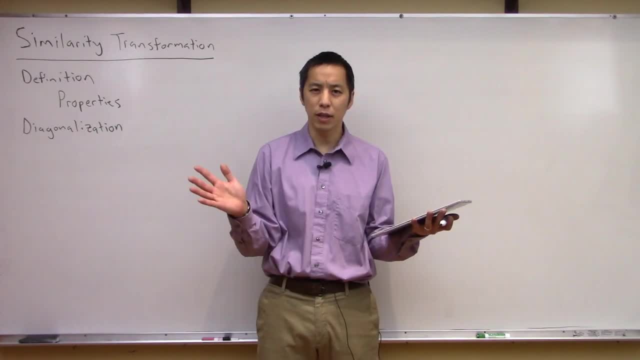 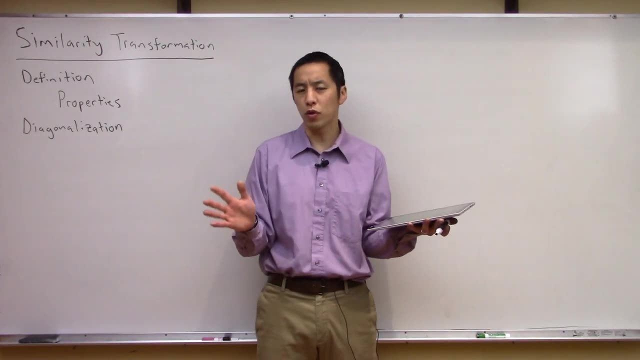 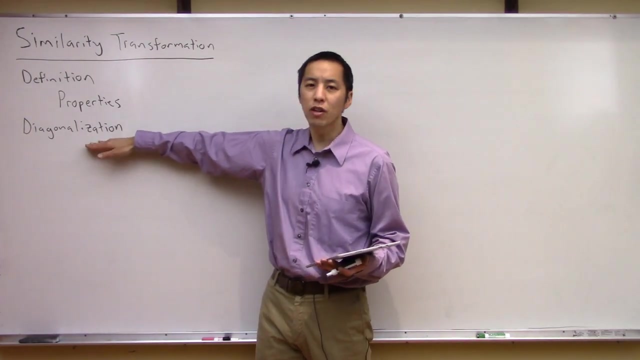 that we just talked about are basically true for any similarity transformation, as long as T is invertible. right Now, what I want to talk about now is one of the most useful types of similarity transformation, So I would like to look at a particular T that is going to, uh, diagonalize. 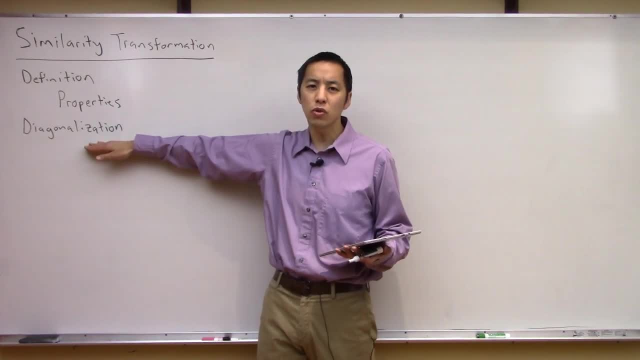 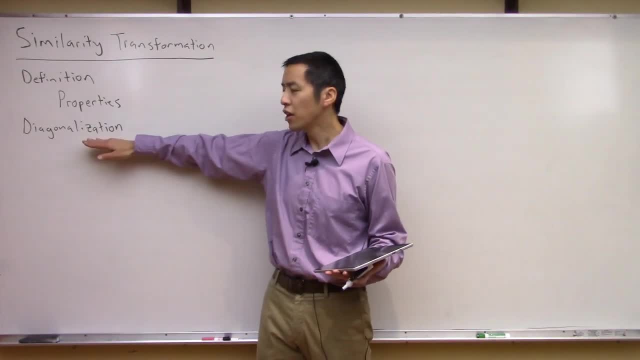 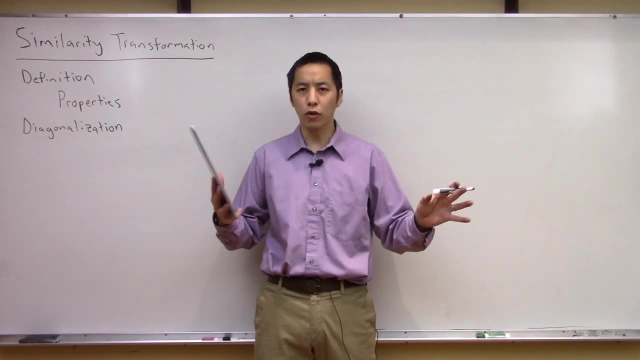 values along the diagonals and zeros everywhere else. And again, this process is known as diagonalization because we're going to take a matrix A which is- uh, you know, might have entries all over the place, And then, through a similarity transformation with a very specific T. 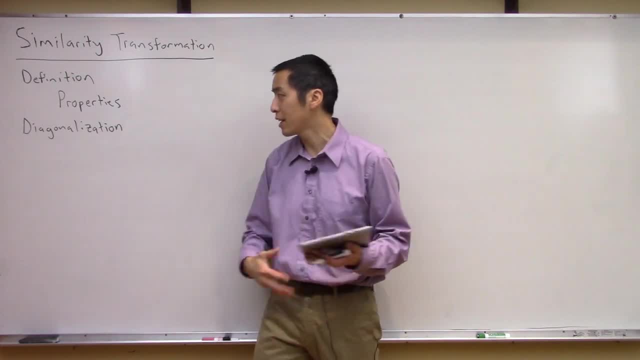 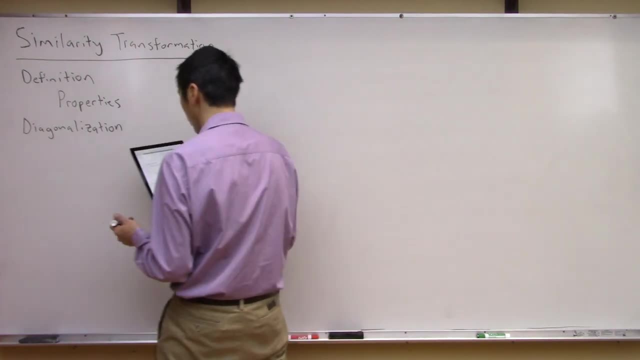 we are going to be able to turn that A tilde matrix completely diagonal. So to go about that, we're going to see this has something to do with the eigenvalues and eigenvectors, uh, of a matrix. So again, remember that for your matrix A right, The idea with the eigenvector. 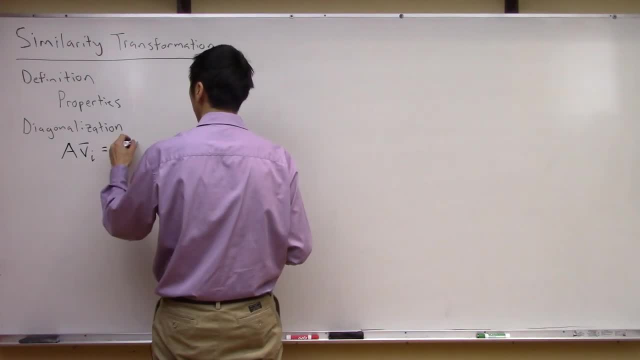 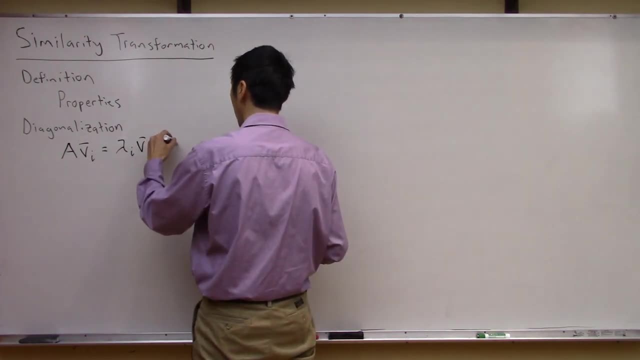 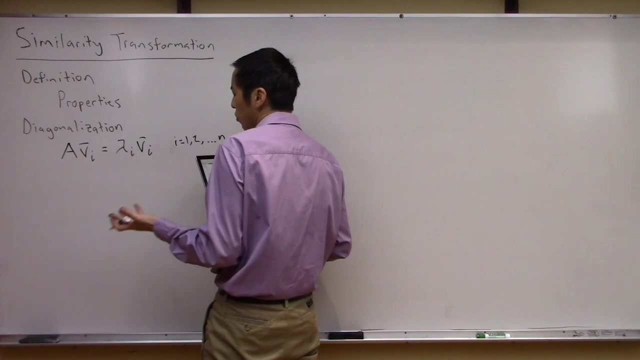 let's call it VI, is that if you multiply it with A, you basically get that same vector, but scaled by the eigenvalue, right? So again, this is for uh. N equals one, two all the way up to, or, sorry for I equals one, two all the way up to N. right? So tell you what let's write. 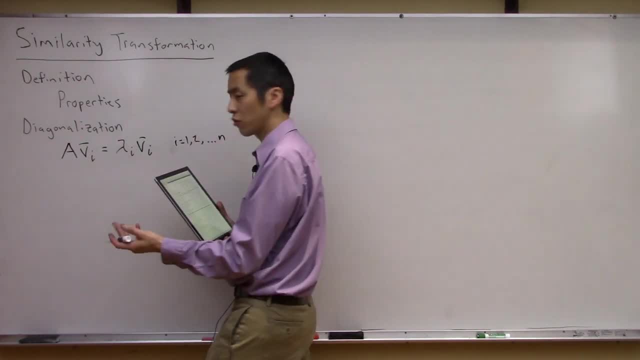 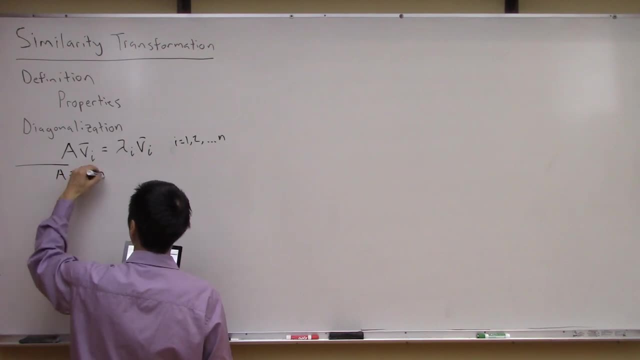 this out: as you know, N separate equations, right, So you could write this as: uh, N separate, as basically: um, you know, a V one equals Lambda one, V one right. A V two is equal to Lambda two. 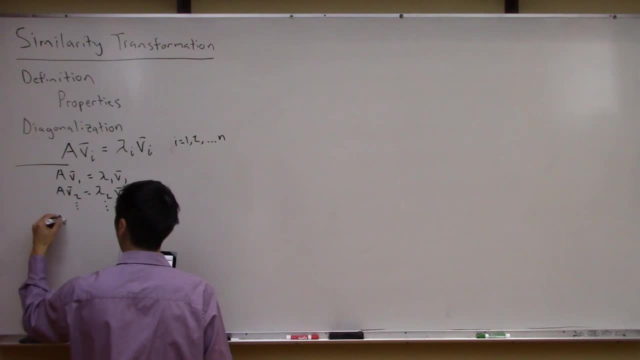 V two, et cetera, et cetera, all the way down to a V. N is equal to Lambda N, V N right. So these are basically N equations, right Individually, one of them at a time. Okay, So what I would like? 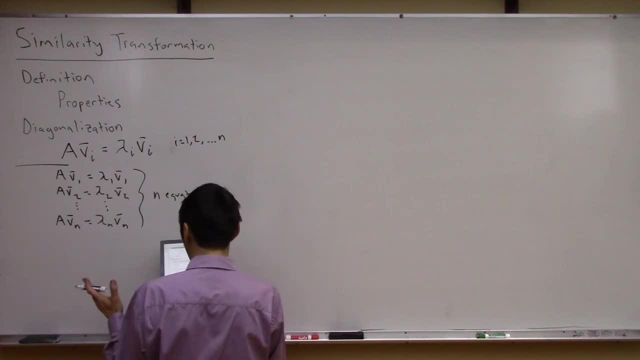 to now do is: how about let's stack all of these up together? So what I mean by that is: I would like to uh take this first. let's look at one of this one equation. right Again, maybe we should be a little more. 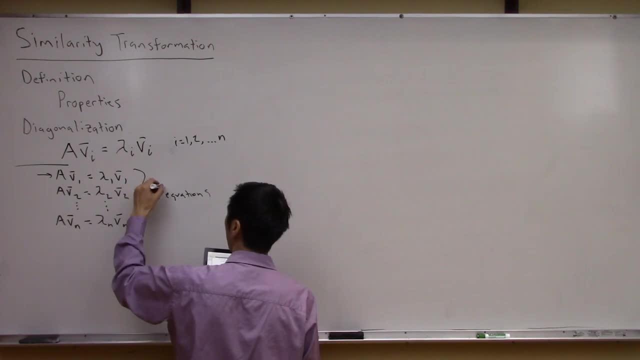 specific. This is any equations and it's an N sort of vector equations, right? Because this first equation right here it's basically says this is a vector uh is equal to another vector, right, And it's an N element long vector. So you can think about the left-hand side, this A V one. 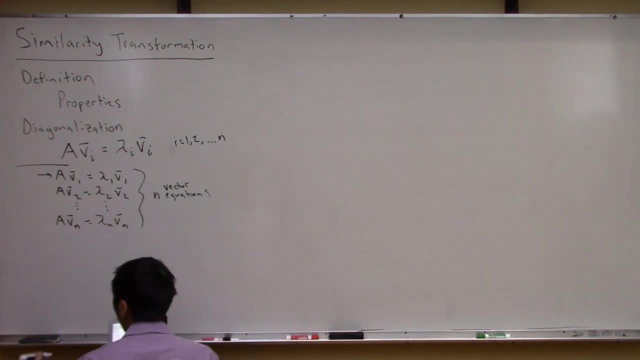 right, It's an N by one element vector. So you know what? Let's stack this, Let's, let's start making a matrix where this first column is going to be this thing here, right? So this is going to be a V one, right? So I'm going to basically just take this first part here, put it over here in the 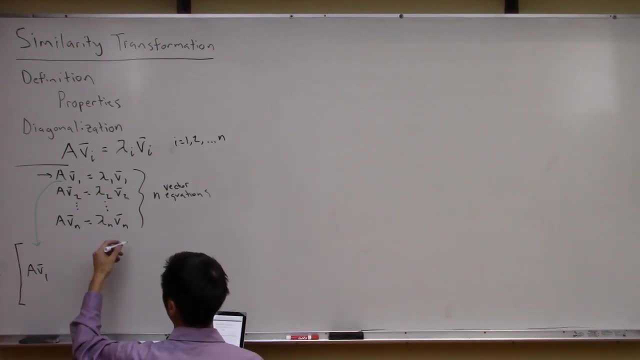 first column of this matrix, uh, that we're going to build up, Okay, And again, uh, let's leave the entries over there as something else. Uh, and I guess we're going to take a look at that in a second. Um, this is equal to: uh, you could. 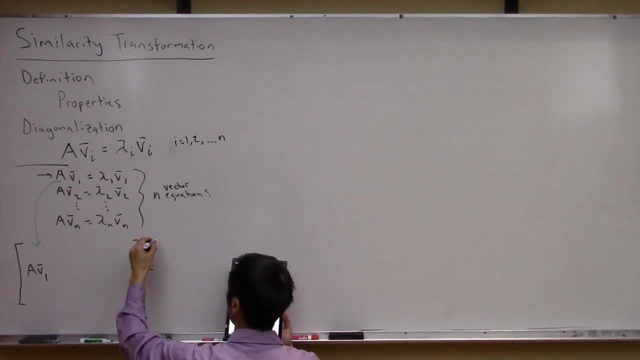 write this as um and again. let's write it again as another vector over here. Uh, the right-hand side of this is Lambda one V one. Would everyone agree? That's the same thing. So I'm basically just taking this part and jamming it in over here. So these again, you can think about these. 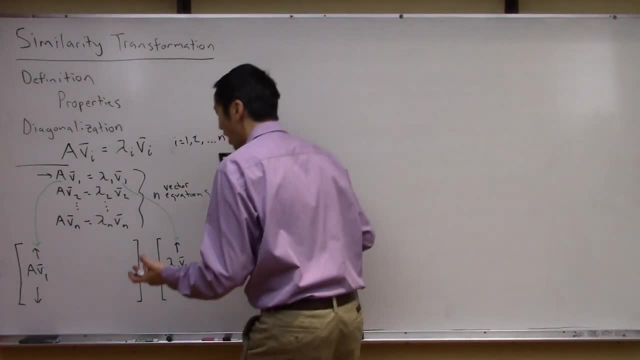 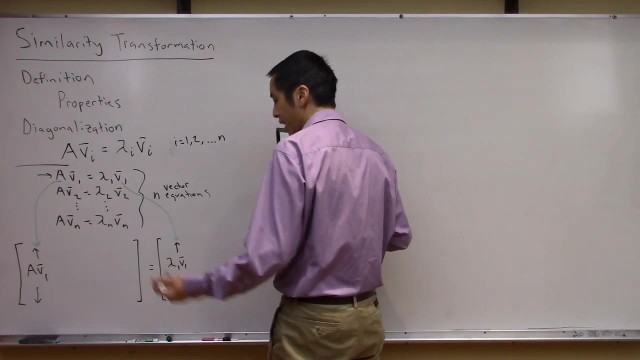 things. So I'm really I haven't. I haven't rewritten anything, I've just stacked it up. So this first equation is basically the first column of this matrix. right, Let's do the same thing, for the second column of this matrix is going to be the second entry, So this is going to be a V two. 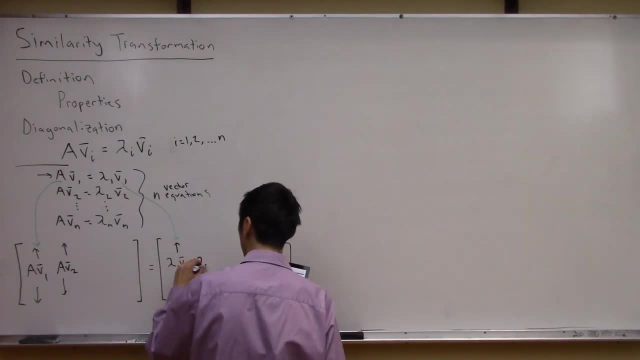 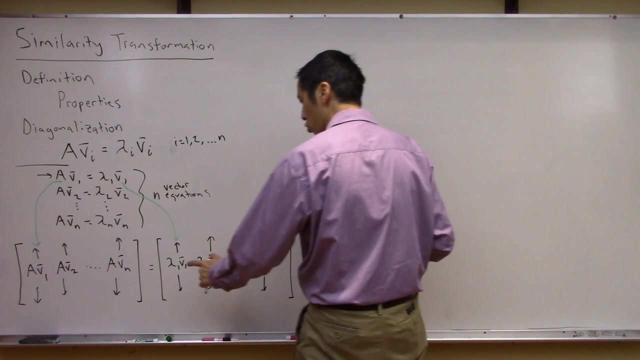 right, That's this column is equal to Lambda two V two, right, Right, Et cetera, et cetera. As you can see, and we're going to go all the way down to a V, N is is equal to Lambda N. V N, right, Right, Okay, Um, okay. So this is basically again, think about. 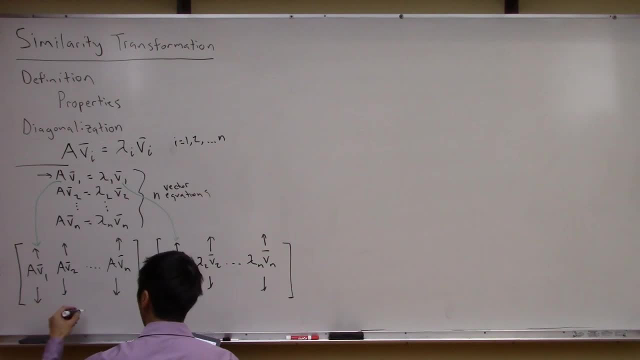 the dimensionality. This entire matrix. here is a N by N, square matrix, right Because this vector right here. this is an N by one, This is an N by one and all the way down to an N by one. So you stack up all of these. 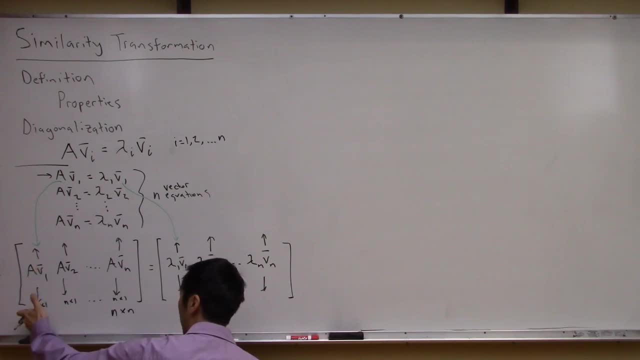 And you have these, this N element vector, N element vector, N element vector. You stack up N of them. You end up with an N by N matrix, right, And same thing over here, right? This thing is an N by one, This is an N by one, all the way up to an N by one. So you stack them all. 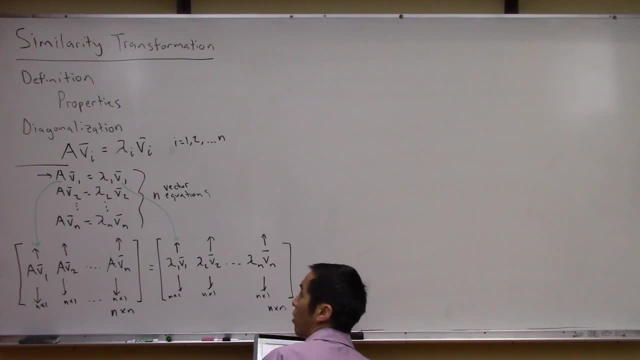 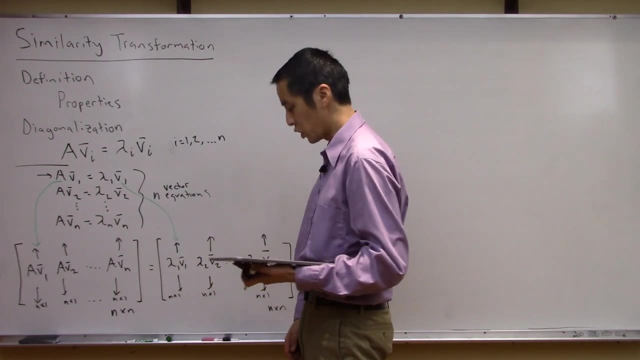 together. So this whole thing is an N by N. So you basically again, we now are basically taking all of your eigenvalues, eigenvector pairs, and we're just writing them as a basically a, a matrix equation, right? So now you know what we can do. Tell you what, let's move on. 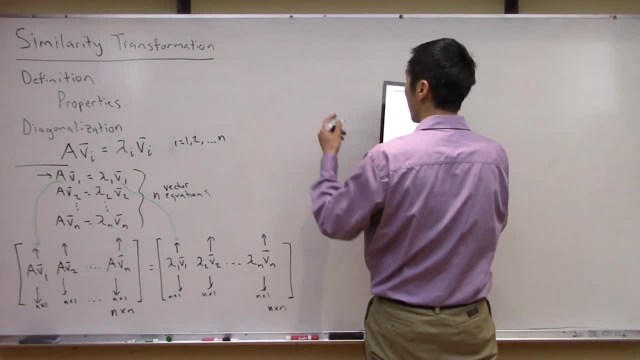 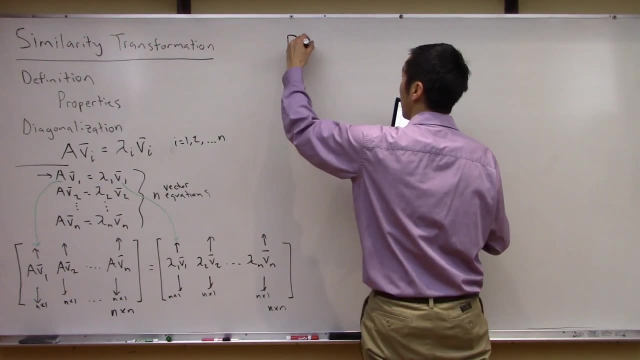 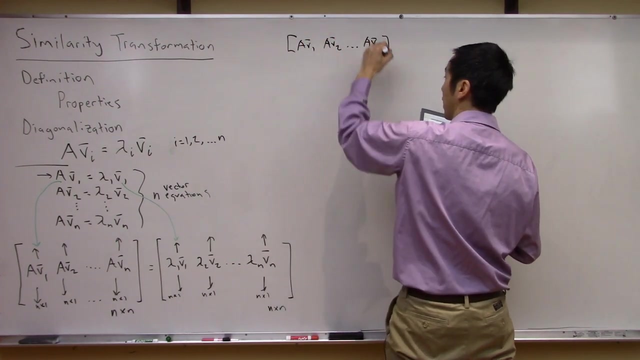 So everything over to one side, okay. So what I mean by that is I'm going to drop that, this sort of vertical vector notation, because I think we all understand that AV1, this is a vector, AV2, this is a vector, all the way up to AVN- This is a vector. right, And I want to move this to the. 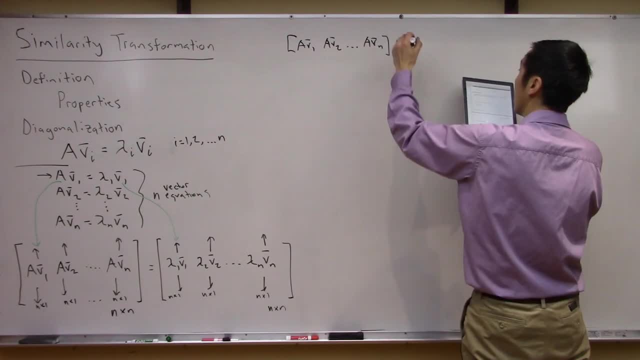 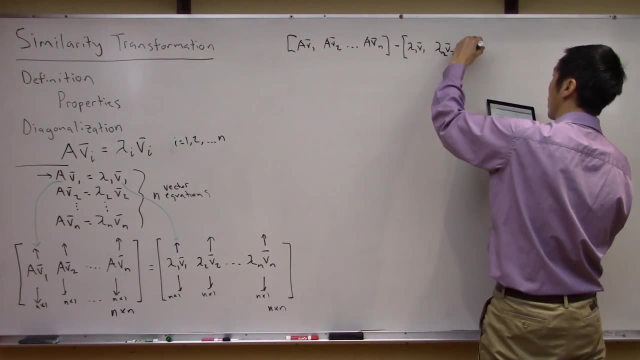 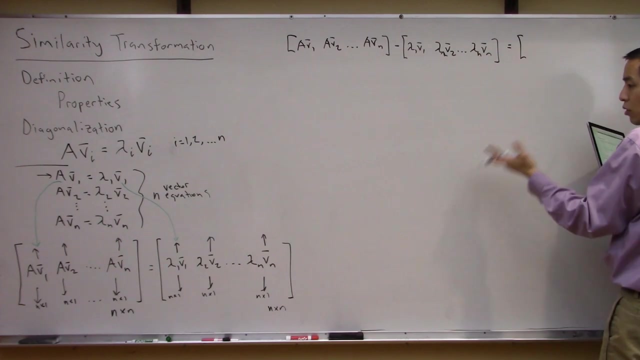 other side. So I have to basically say: minus right, Lambda one, V1, lambda one, sorry, lambda all the way up to lambda N, VN, right, This has got to equal. it's a bunch of zeros, right? Because? 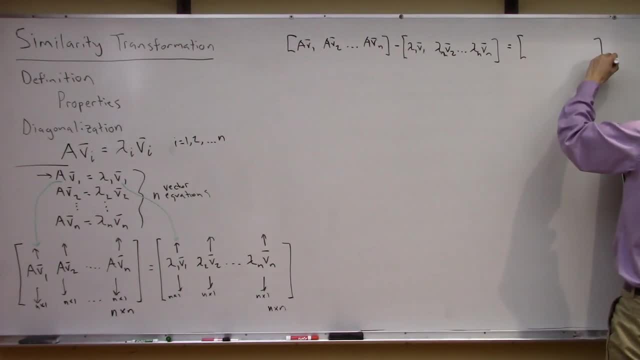 I moved it over to the other side. So this is basically a N by N matrix of zero. So you can think about this as like: again, a zero vector here, zero vector here, all the way up to another zero vector right, And again, each one of these is an N by one, N by one all the way up to N by. 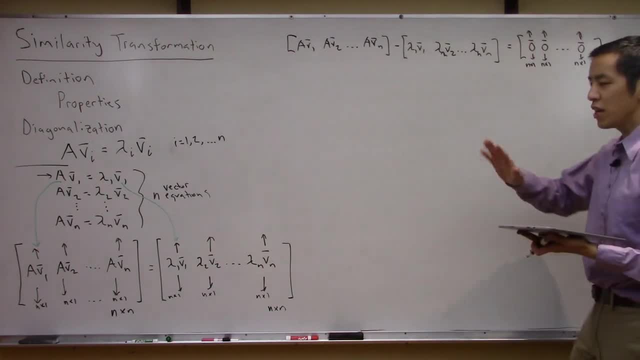 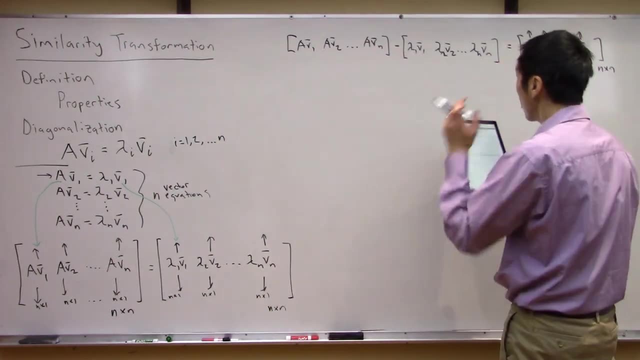 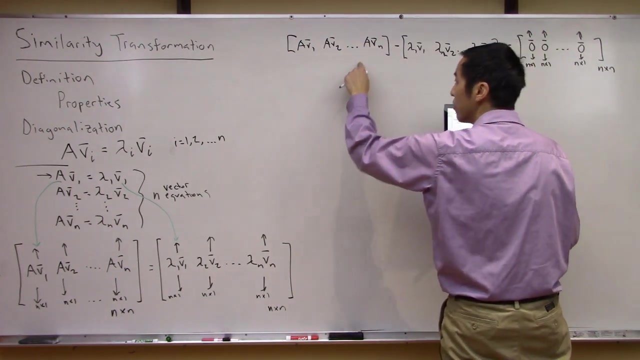 one. So you end up with an N by N. So again same thing. Well, I'm doing nothing more than just rewriting these N vector equations in matrix form, right, Okay? So now, what's great about this is let's examine this first term. here. You notice A is pre-multiplied everywhere, So let's pull it. 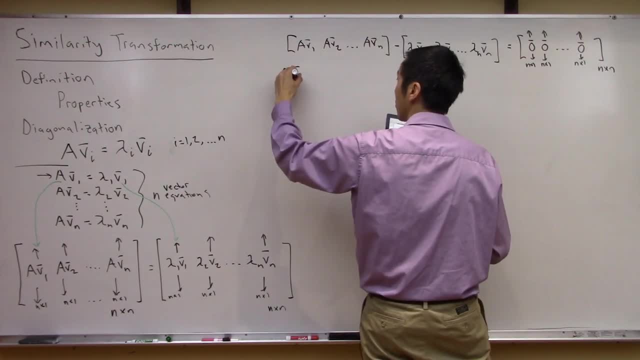 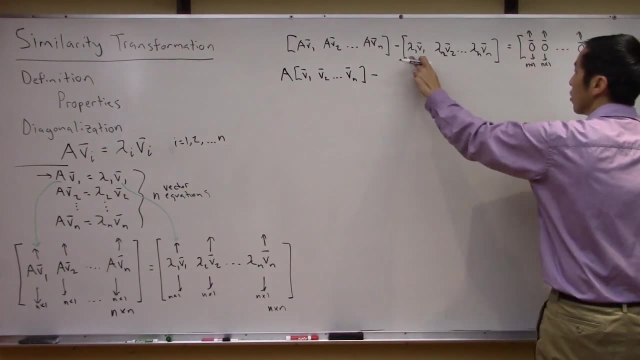 out on the left, So this can be rewritten as A times V1,, V2, all the way up to VN, right, Okay, Minus, Let's look at this thing. okay, This thing, lambdas, right, Remember all these eigenvalues. 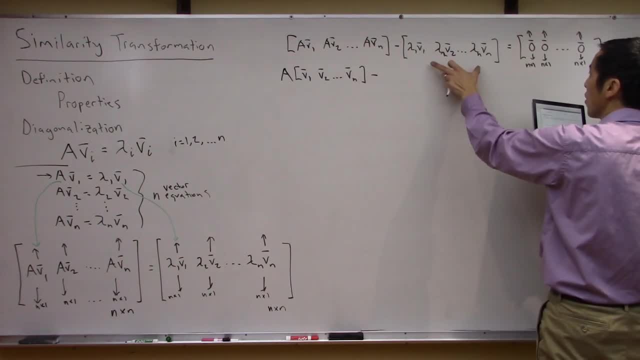 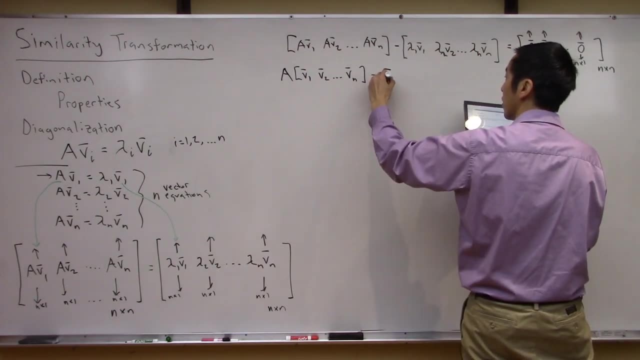 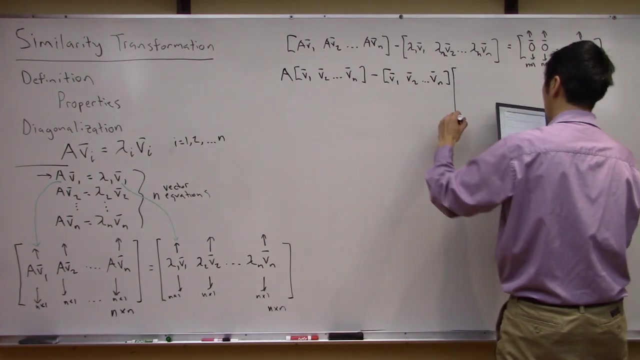 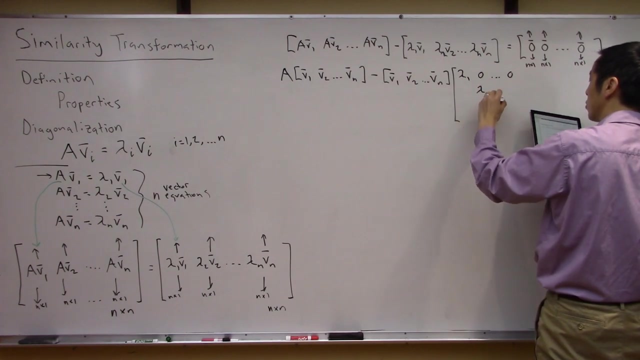 scalar numbers right. So if you stare at this N by N matrix long enough, you'll basically see that you could write this whole thing as V1, V2, all the way up to VN times, a diagonal matrix which is lambda one, zero, zero. Basically it's lambda one, lambda two, all the way down to lambda. 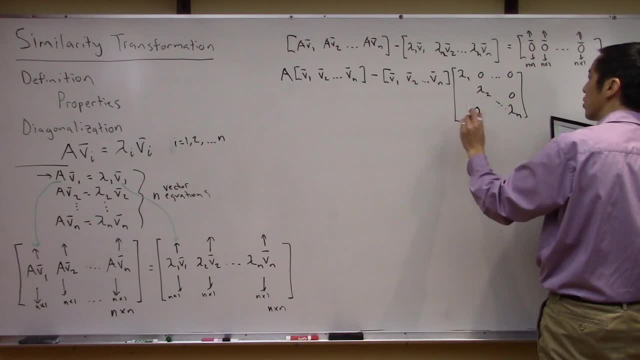 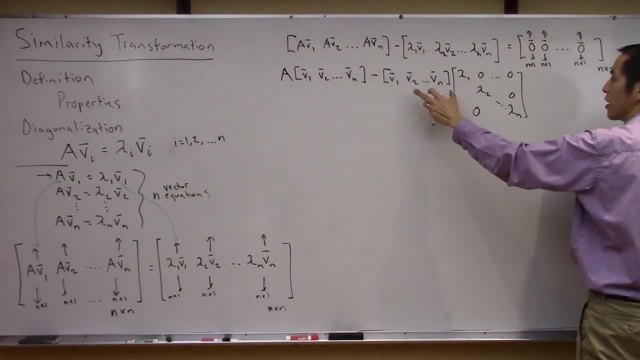 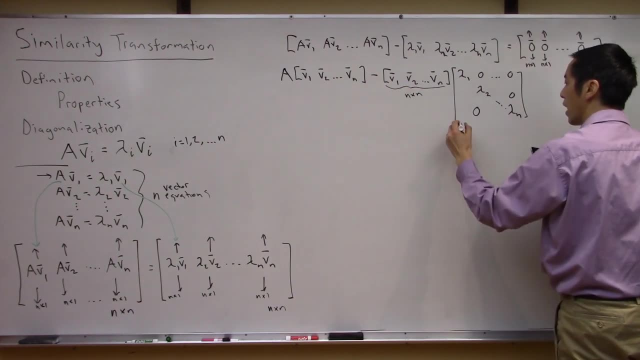 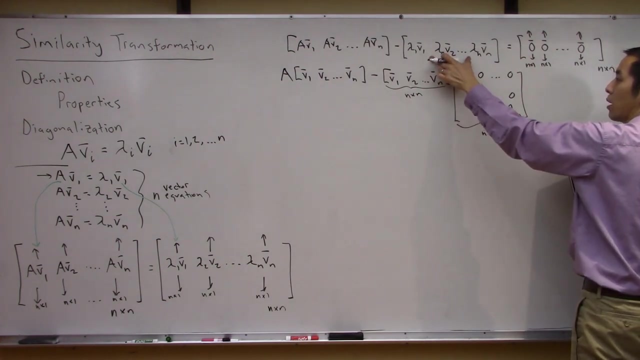 write it like a diagonal matrix. So again, take a little while to convince yourself of this, that this matrix, which again is an N by N, right, This whole thing is an N by N, And so is this thing. This is an N by N matrix, right? The product of these two is this term up here, right? Okay? 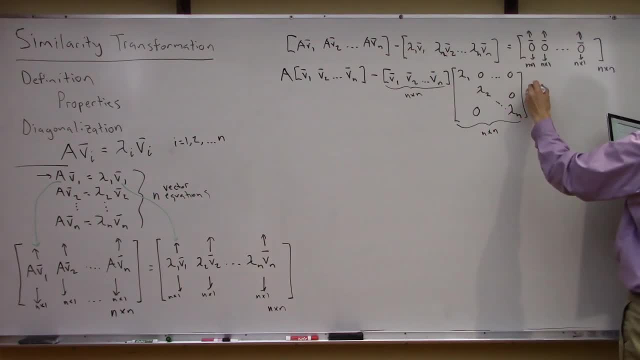 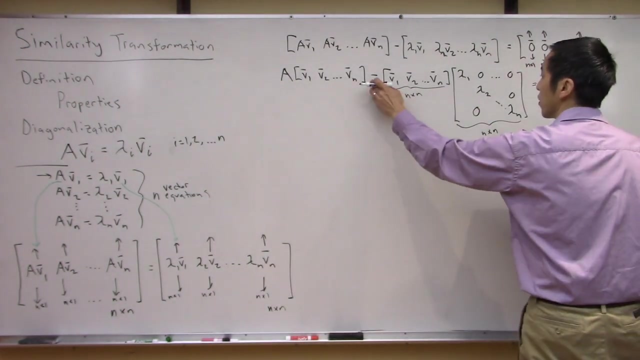 So again, this is equal to again this big giant zero matrix on the other side, right? Okay, Great, great, great. So now, actually sorry for moving things back and forth, But again, let's go ahead, move this to the other side, right? So let's take all this thing, move it to. 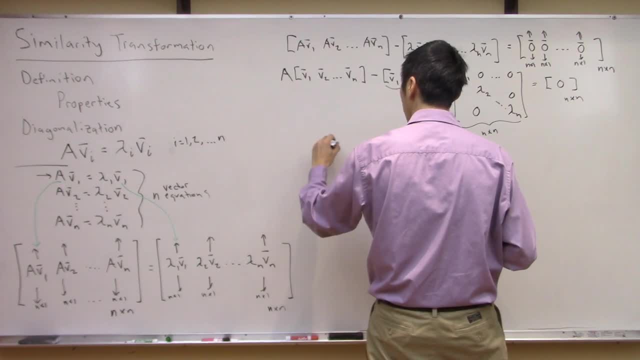 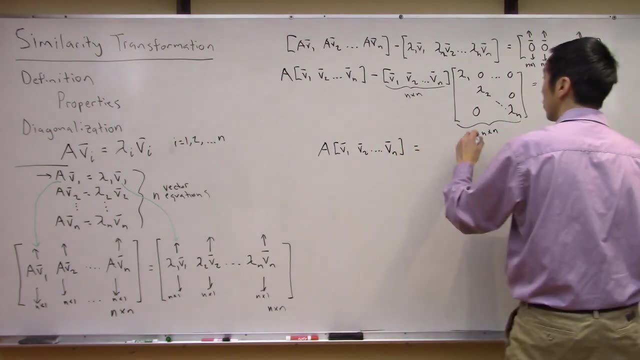 the other side. So we basically end up with this thing where it's A times this V1, V2, VN matrix is equal to this V1 to the other side. So we basically end up with this V1, V2, VN matrix is equal to this V1,. 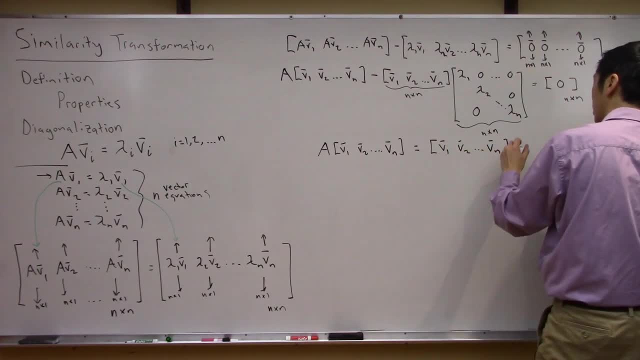 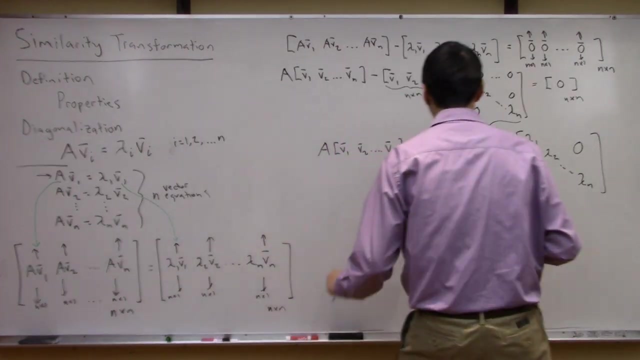 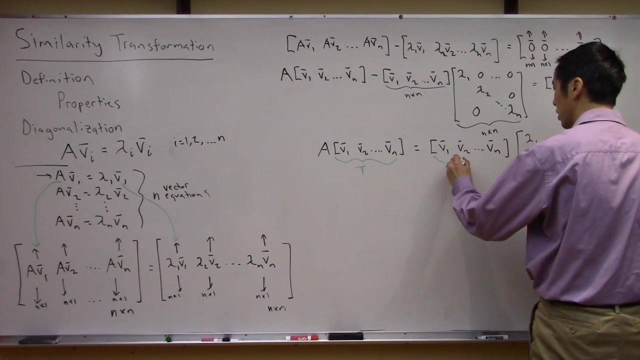 v2, da da, da da da. vn. matrix times this diagonal matrix of lambda 1, lambda 2, all the way down to lambda n and zeros elsewhere. right now, this is fascinating because if you stare at this, why don't i call this matrix here t? this is my similarity, transformation matrix. right, because 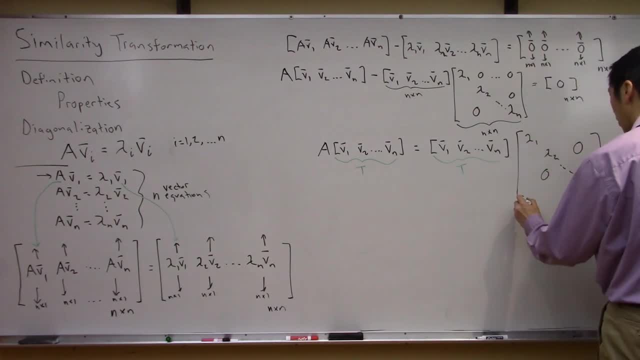 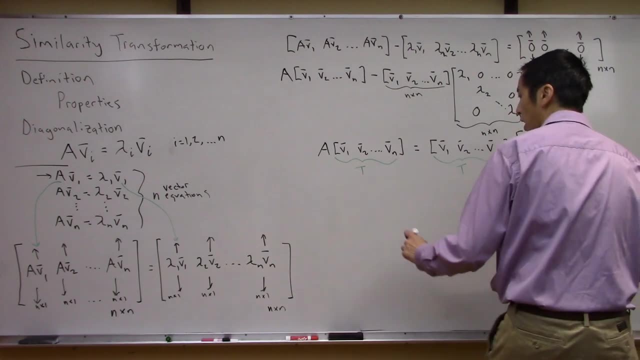 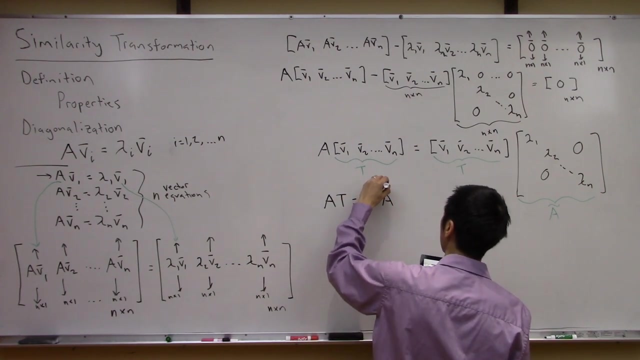 it shows up on both sides, okay, and let's call this thing here. this is, let's call it a tilde, right? so if you look at this, if we go ahead, we can write this now as a t is equal to t, a tilde, right? okay? and now here's the rub. this is fine. this is true so far. so if you look at what we 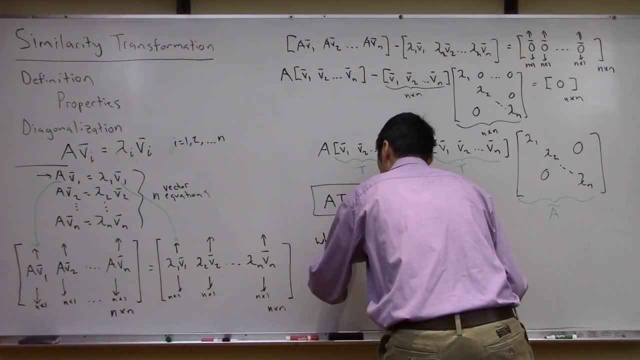 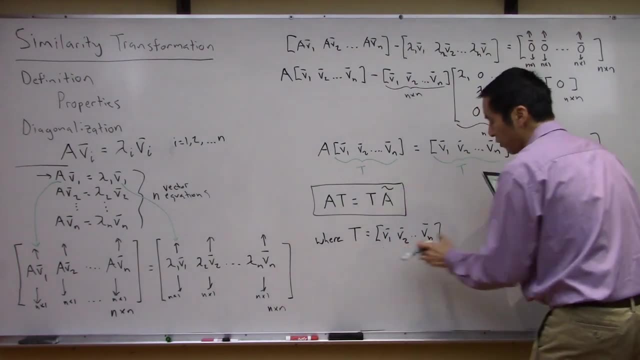 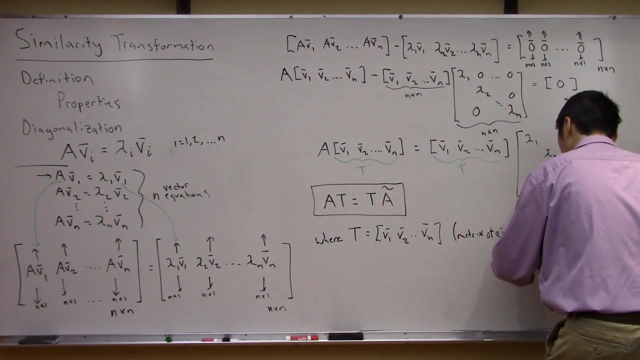 did here is we chose our transformation matrix t to basically be this: v1, v2, all the way up to vn. so what this transformation matrix is, this is a matrix of the eigenvectors right stacked up in column format. and again, i'm going to call that out in column format because, depending on what software packages you're using, 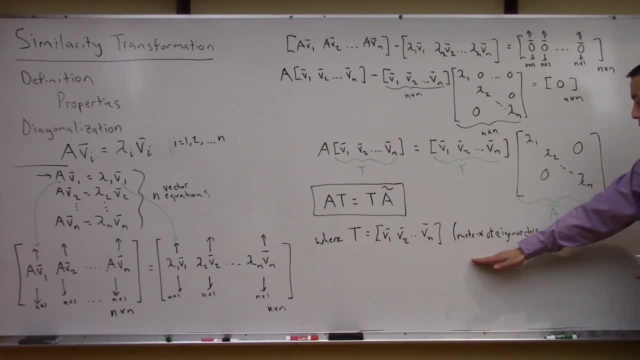 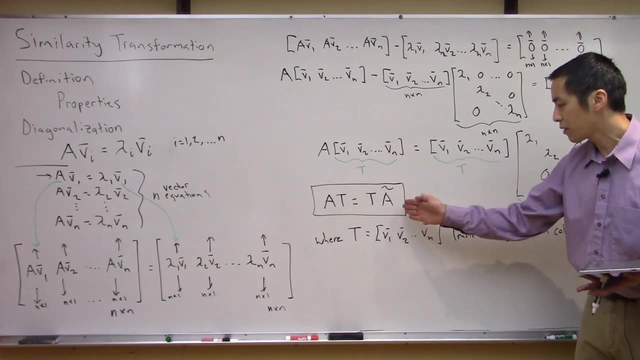 for example, mathematica gives you eigenvectors of a matrix in row format. that's not what we're doing here, right? this matrix t is the first eigenvector as a column, the second eigenvector as the next column, etc. etc. all the way up to the nth eigenvector as a column. here, right, but this is the very special transformation. 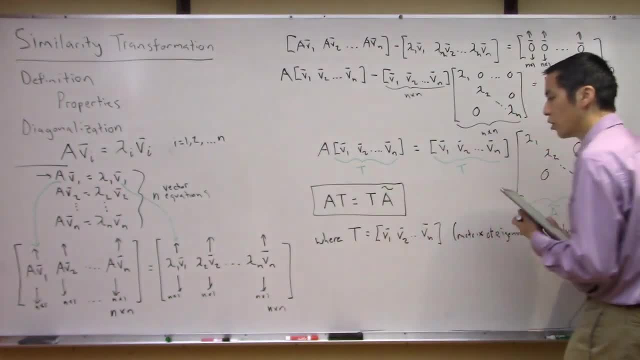 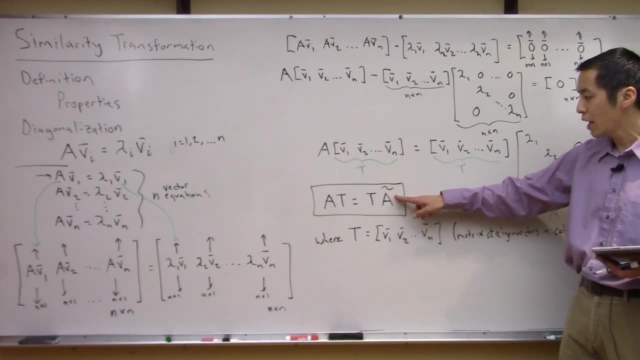 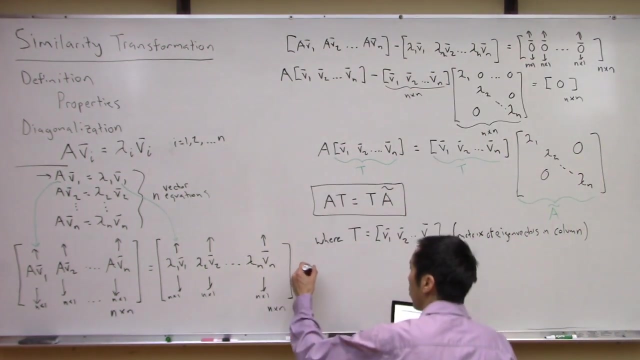 matrix. okay, and this is true no matter what. okay. so we actually haven't done a full similarity transformation, matrix, a similarity transformation, yet, because i haven't isolated a tilde right now. here's where we got to pay a little attention right now. if t is invertible, 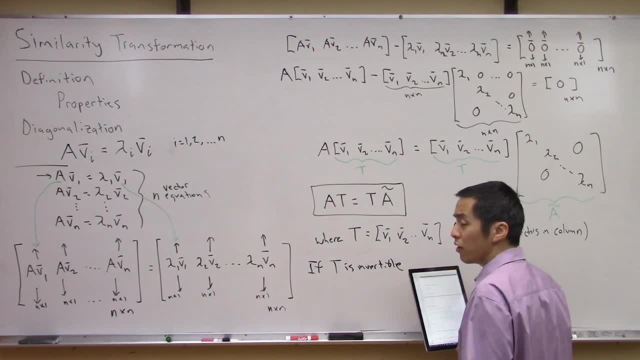 right. if t is invertible, that's great, because if that's the case, what can i do? i can basically isolate a tilde and we end up with our usual a tilde is going to be t, inverse, a t, right, okay. and what's special about that is look at the form that the a tilde took right. so again, 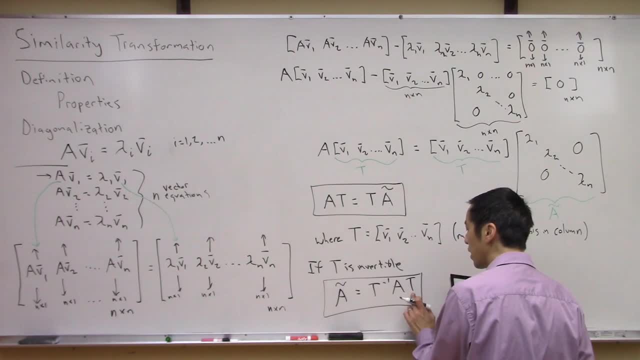 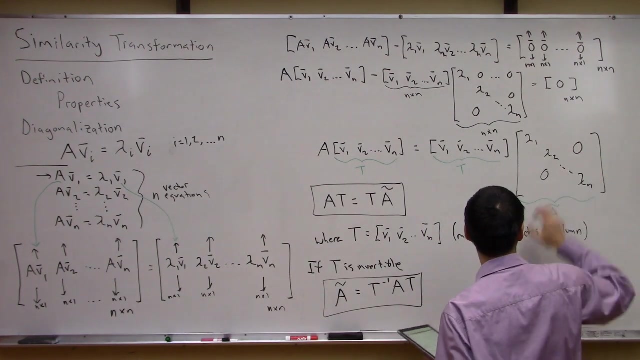 a could have been anything right, but if we use a similarity transformation of the eigenvectors, as are similar to transformation matrix, we end up with this, a tilde format, where you have the eigenvalues falling along the diagonals and there's zero elsewhere. so this a tilde is a purely diagonal matrix right, which is very, very, very nice for a lot of. 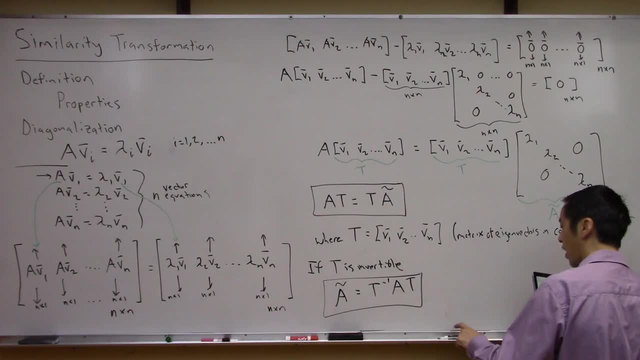 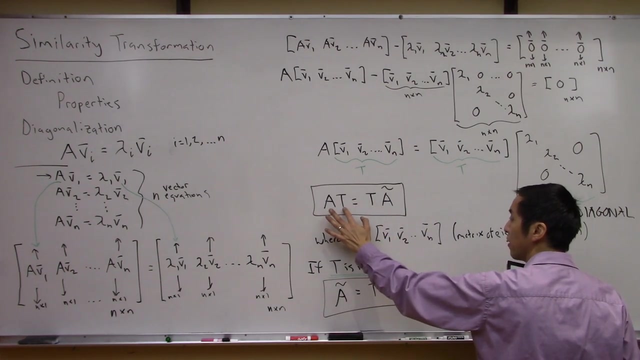 different reasons. right and again. the thing that we have to i want to really hammer home is that this is true if it's invertible- right. if it's invertible, we can diagonalize a matrix, right. if it's not invertible, this is still true. right a times the eigenvectors. it should be equal to the eigenvectors. 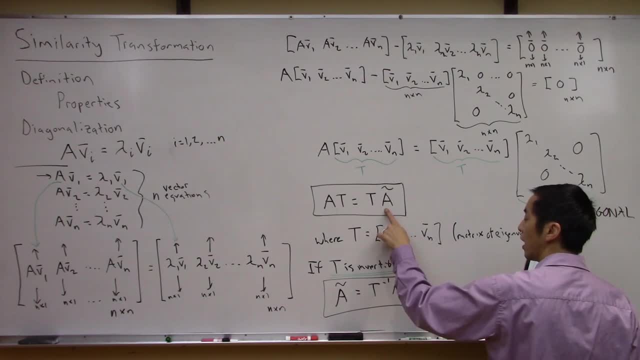 times your diet, your your eigenvalue, uh, diagonal matrix here. right, that should still be true, but you're not going to be able to get all the way down to this, this relationship, if t is not invertible. so again, i think i'm hammering this um home and maybe i'm talking about this too much, but again i 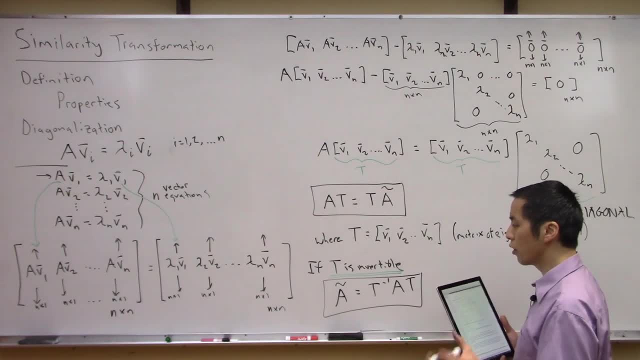 think we're going to see this show up over and over and over, and especially in in control systems and linear system theory. this is sometimes referred to as a um, a modal form um, and sometimes this is this. t is sometimes referred to it, or i should maybe let's just write that down: t is. 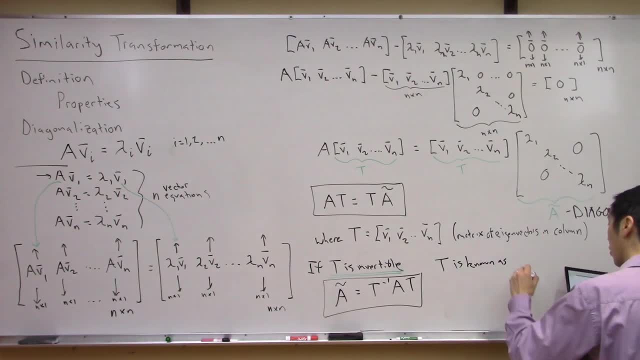 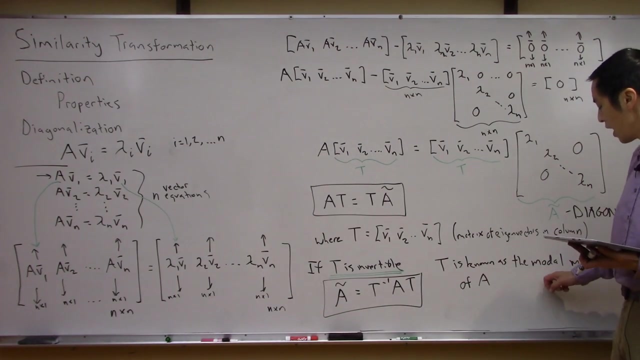 sometimes known um as the modal matrix, modal m, a, m, o, d, a, l modal matrix of a. okay and again. t is just the eigenvectors of a stacked up in column form: okay and um. again. i think it's beyond the scope of the lecture today to talk about what does it mean? for what does the 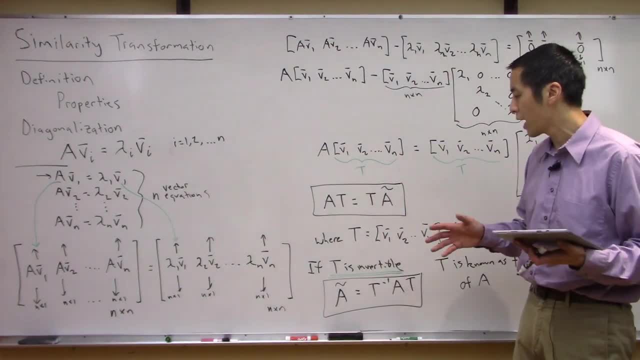 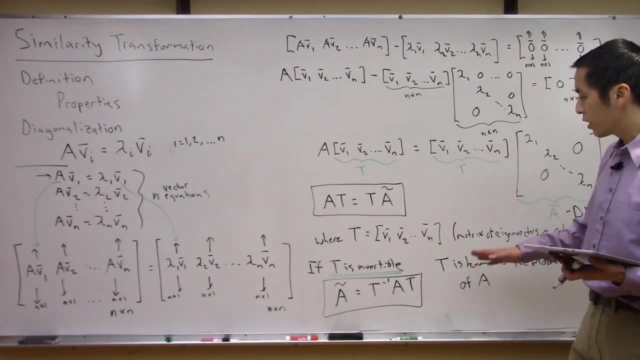 word modal mean. we will talk about that in other discussions. when we look at linear system theory and dynamic systems, i think it'll be much more clear why this is called a modal matrix. but for now we can see that the power of this is that it allows us to diagonalize um a matrix, and we see 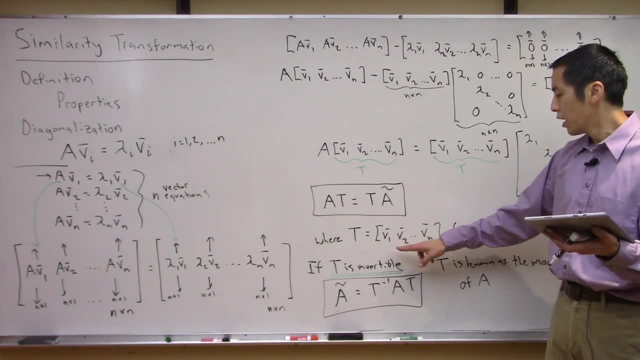 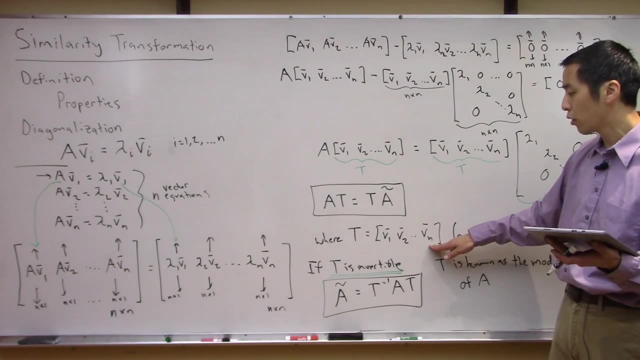 there are some cases where we can diagonalize a matrix and we see that it allows us to diagonalize right. we have to ensure that, uh, the eigenvectors basically span the space right if the, if all the eigenvectors stacked up column wise, are full rank right. that means this: t hold on, let me, let me let. 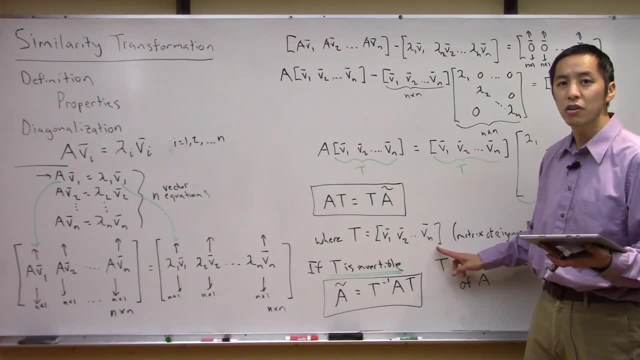 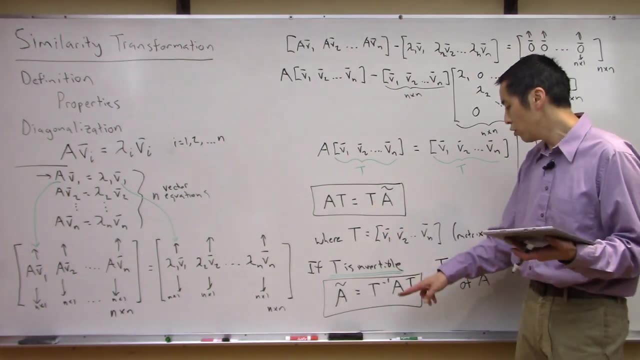 me get. let me get that straight: if the eigenvectors are all linearly independent, right, meaning the eigenvectors span the space, then t will be invertible and you can diagonalize a matrix, right. so again, uh, this is a little bit, uh, it might help us understand a little bit more about the 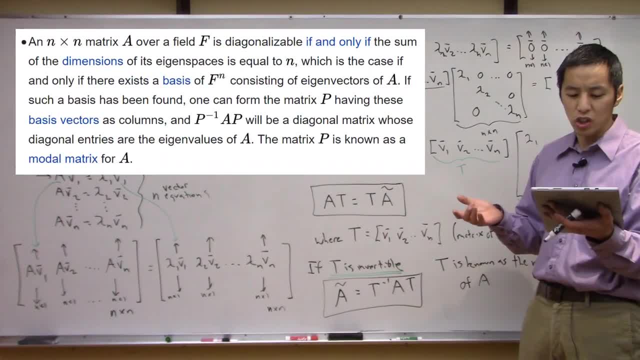 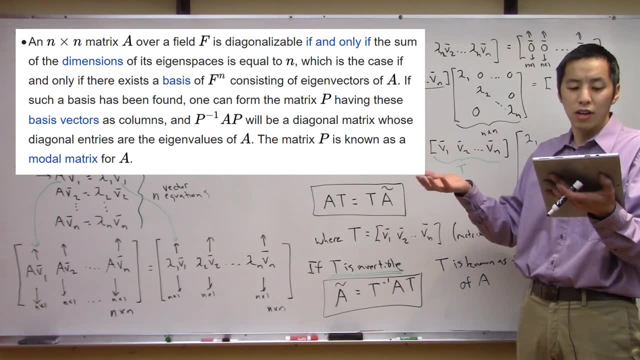 diagonalization. and if you, for example, if you look at the wikipedia page on diagonalization, in fact, in fact, here i'll flash up um a screenshot of the of the text there, right, and says basically: right, you have a square matrix which is diagonalizable if, and only if, right, the sum of 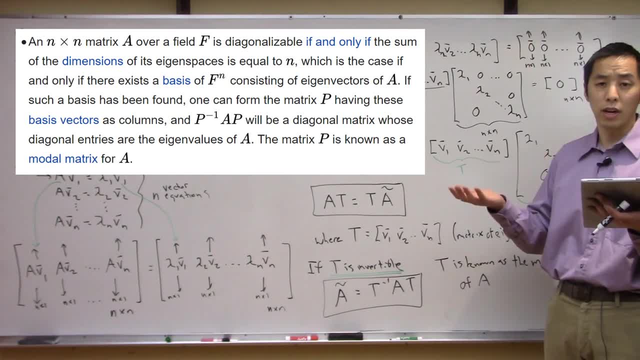 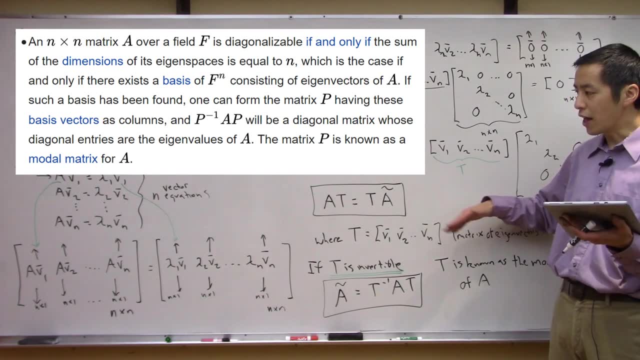 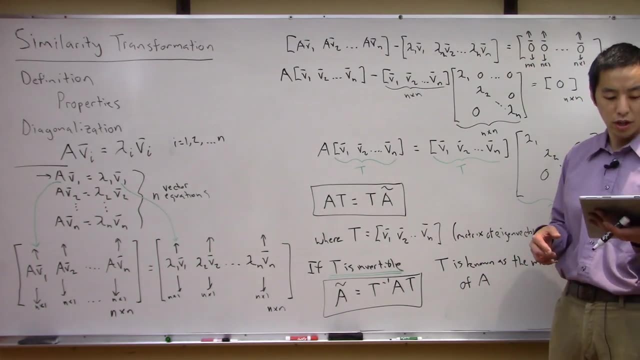 the dimensions of its eigen spaces is equal to n, right, the full space. so basically, that's exactly what we're talking about. right? if the eigenvectors span the space, then the matrix is diagonal, is right, you can perform this diagonalization, uh procedure. okay, now um, if it's and, and and in that, 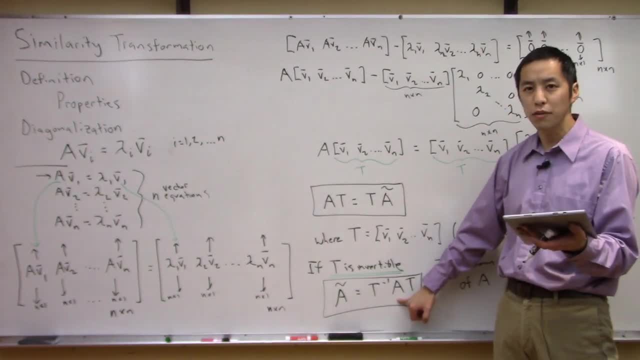 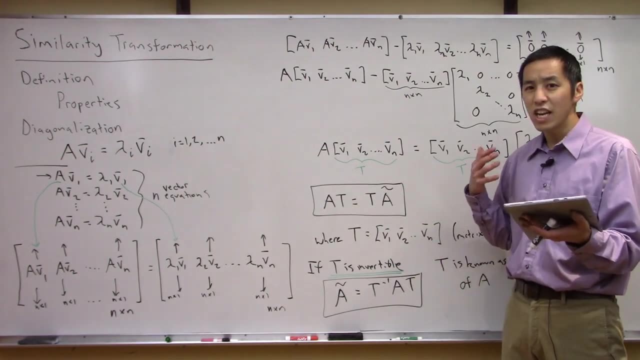 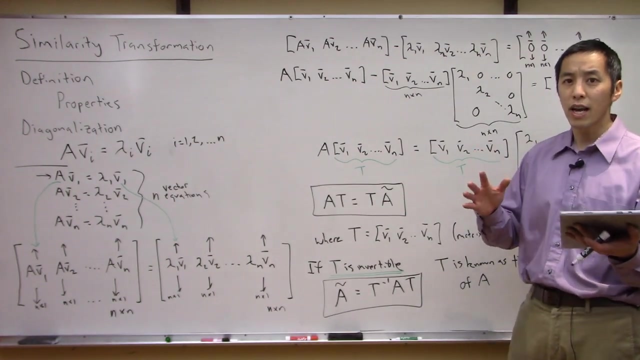 case a is sometimes referred to as a non-defective uh matrix because it can be diagonalized right um. if it cannot be diagonalized, it's sometimes referred to as a defective matrix, and in fact, that's what i want to look at right now. why don't we take a look at an example um of all of these? 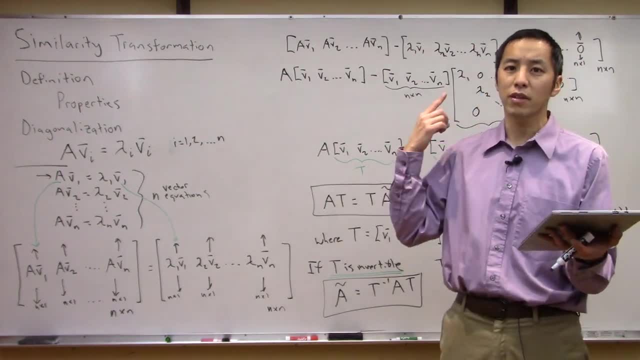 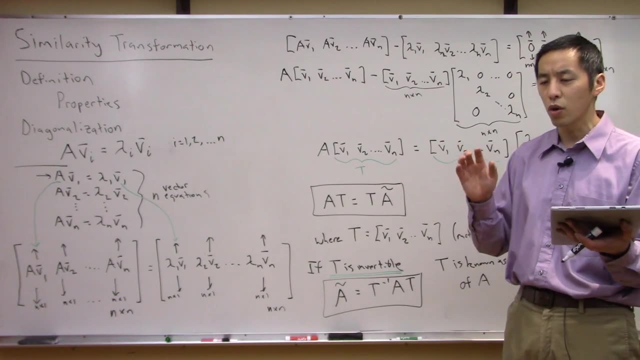 uh, with those two situations- a non-defective matrix and a defective matrix. so we'll run through all the properties we talked about. we'll show those properties are true regardless if the matrix is defective or not. um, but we'll see that this diagonalization is only possible for a 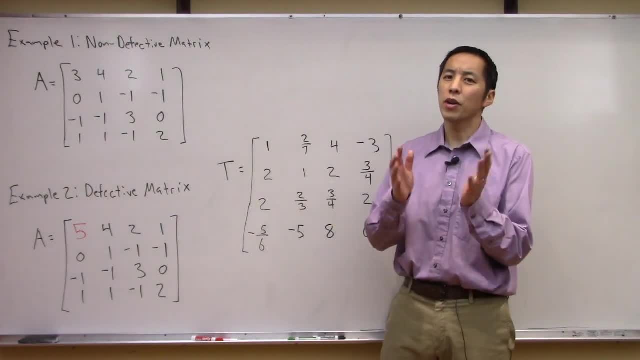 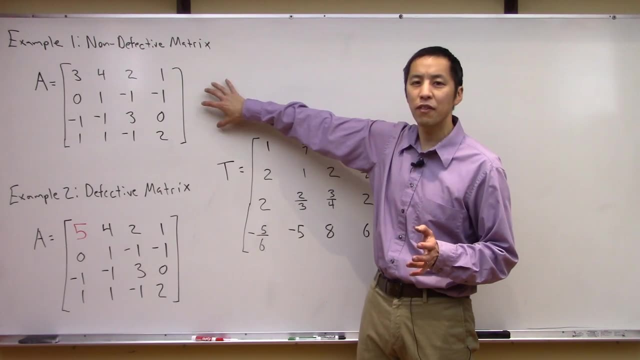 non-defective matrix. all right, so here are the two example matrices that i'd like to look at. so the first one is a non-defective matrix, so we'll see that this one has eigenvectors which span the space, and again, that only matters for the non-defective matrix, so we'll see that this one has. 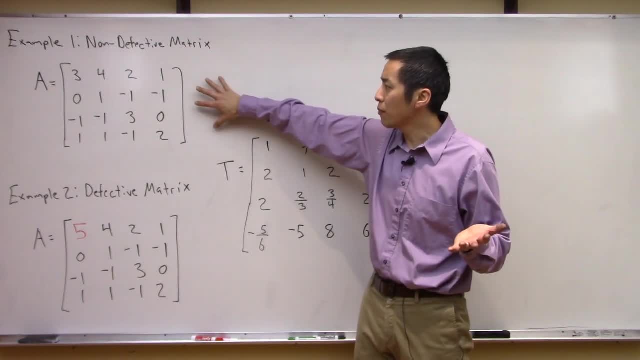 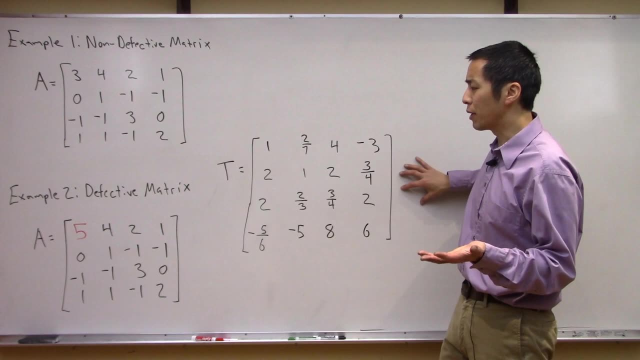 eigenvectors which span the space, and again, that only matters for the non-defective matrix. so we'll show that this matrix when we go ahead and use a similarity transformation, namely i'm going to use this similarity transformation of t here um to basically compute our similar matrix- we're going 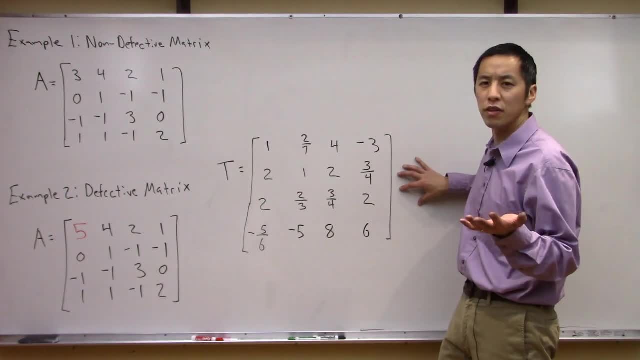 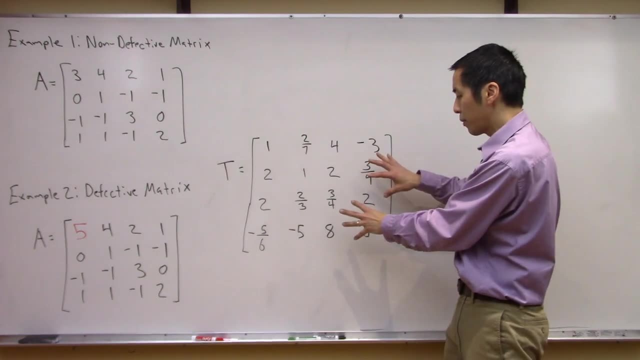 to see all those properties hold of properties, one through five, regardless if it's defective or not, and we'll see that, since this matrix is non-defective, we'll then be able to use a another transformation matrix, which i think we're going to call it m instead of t. we'll use m to denote. 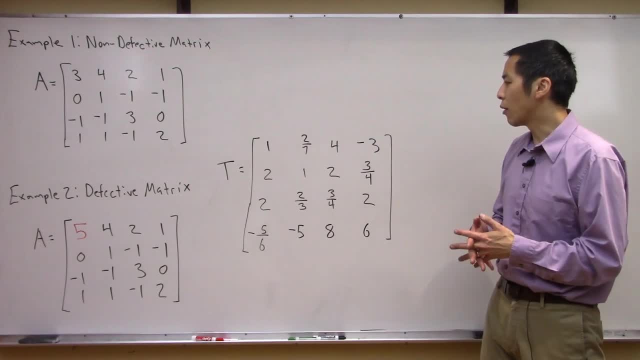 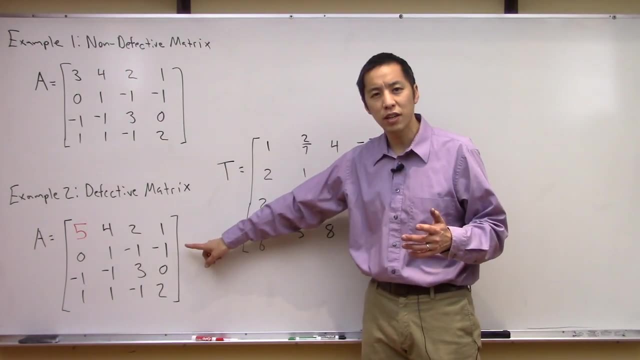 the modal transformation, which is just the eigenvector of the non-defective matrix, and and we'll go ahead and look at diagonalizing that matrix, a okay, um. and then the second example. i'd just like to look at a slightly different matrix. it's the same as the first matrix, the only entry. 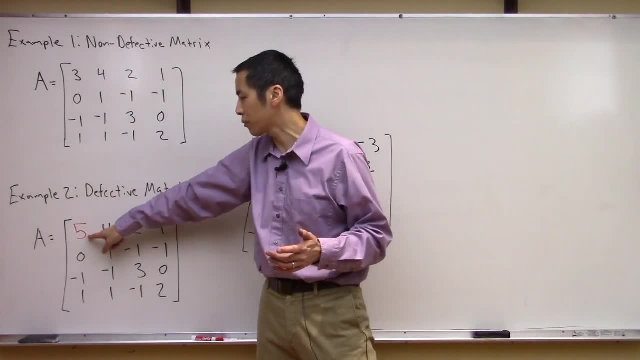 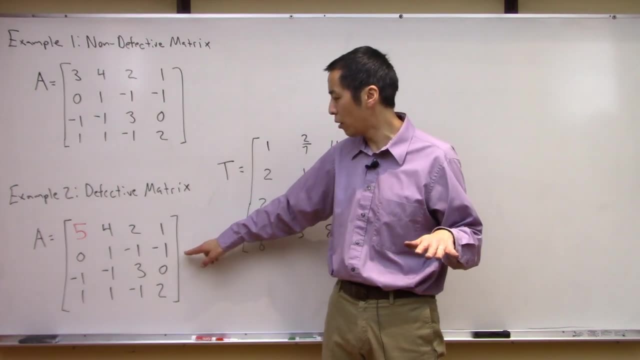 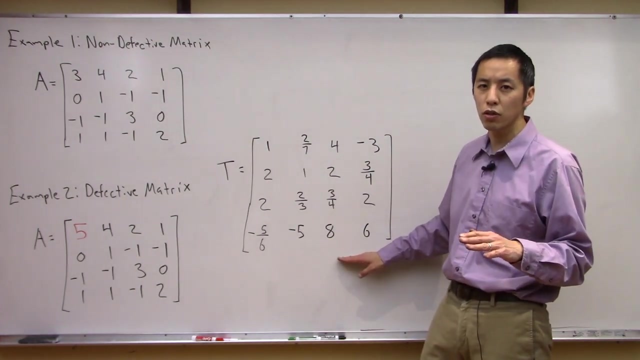 that's different is this red one in the one one position. so instead of a three, let's make it a five. this matrix is actually defective, so its eigenvectors do not span uh r4 in this case. but again, we will go ahead and use the exact same transformation, uh matrix, here to. 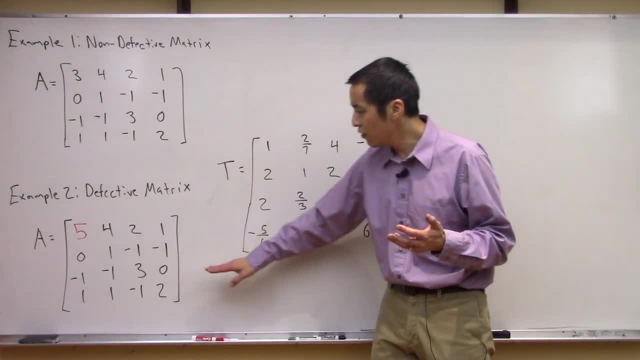 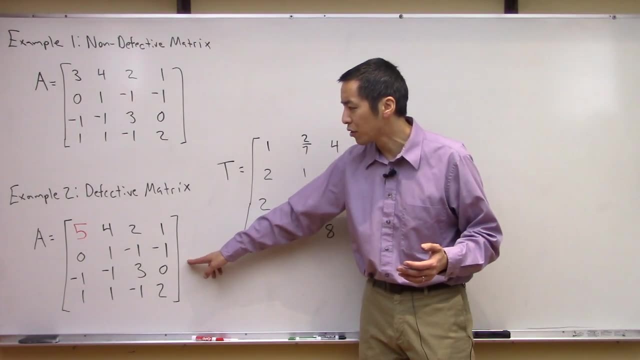 perform our similarity transformation and we'll see that still, even though this matrix is defective, um properties one through five still hold. it's just going to be an issue: we're not going to be able to diagonalize this matrix using the modal transformation of its eigenvectors. so, um, why don't? 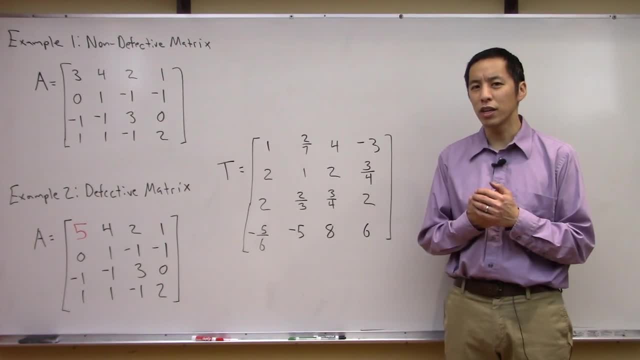 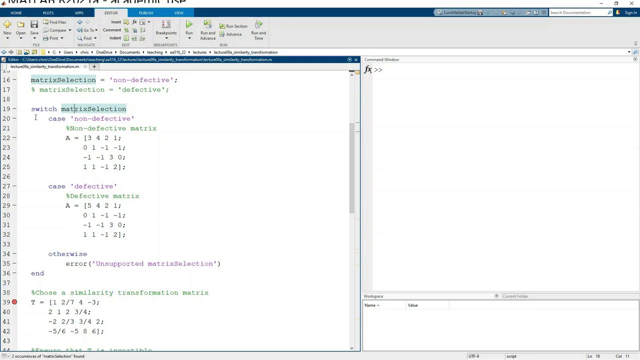 we jump over to matlab and actually do this, because it'll be a lot quicker and easier just to to have matlab do a lot of these operations. all right, so here we are. i've just written a little bit of code. i had a time to save ourselves some of the code that we're going to be using in this. 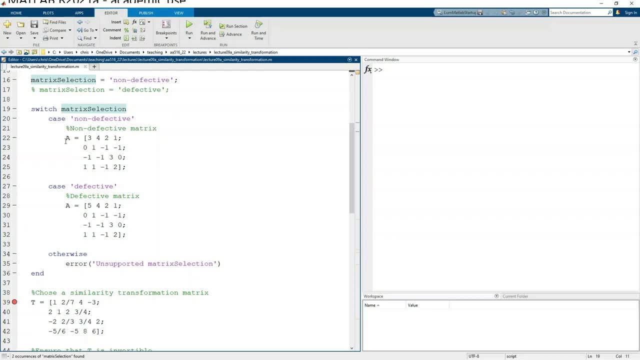 um, headache and um, as you can see, i'm just going to go ahead and get the- uh- non-defective matrix to start with. so let's go ahead and run this and uh, okay, here is our transformation matrix, our similarity transformation matrix that we talked about, up on the board. um, so again, uh, let's just 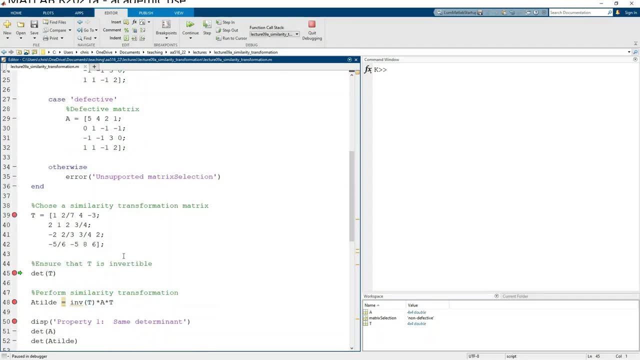 go ahead and run to the next breakpoint to get t into the uh system. now let's again make sure that t is invertible. so let's compute its determinant and we see: yep, that does not look anything near 0. think we are good to go. t is definitely invertible, so we should be able to perform our similarity. 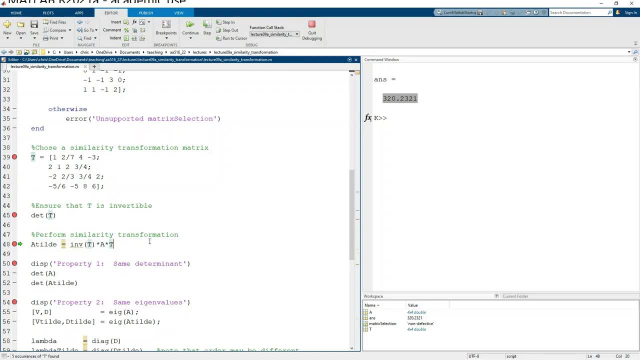 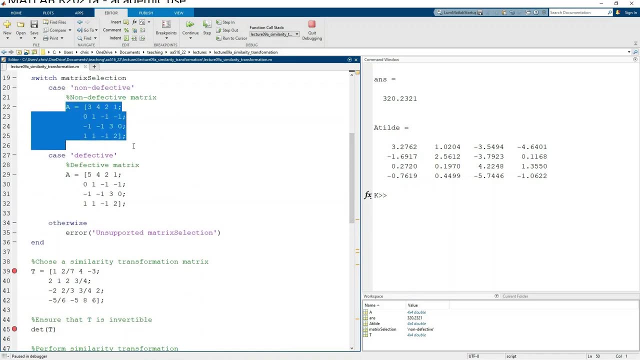 transformation matrix here using just t, inverse a, t. so let's go ahead and do that and, as you can see, we get something totally different than what we started with, right? so here was a and now here's a tilde. it looks completely different, but, as we discussed on the board um a lot of these things, 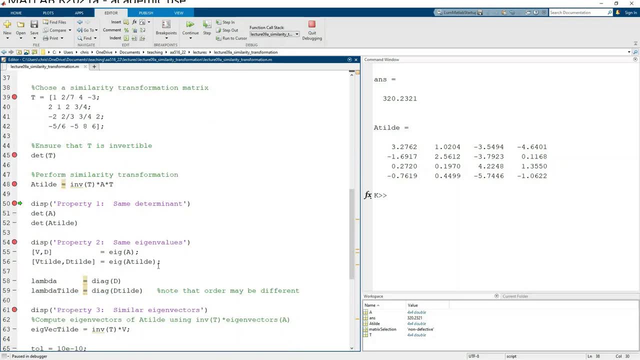 are the same. four properties should be the same and the fifth, one, right, the eigenvector, should be the same. let's just go ahead and take a look at this. so, property one, the determinant right, both determinant of a and a tilde, those should be the same. so let me just execute that and we see. 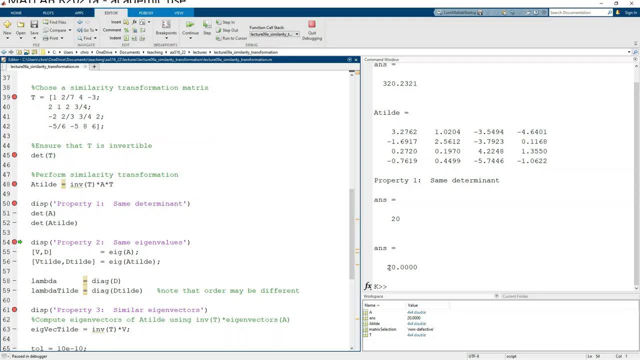 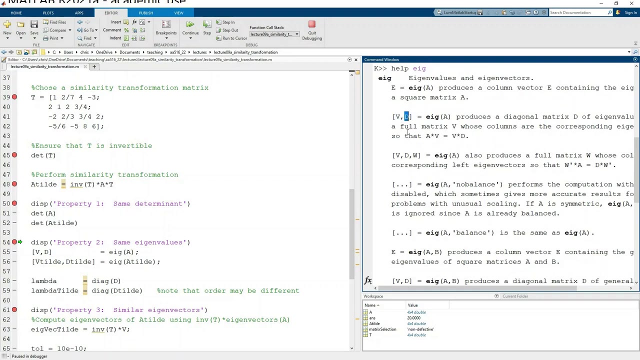 yes, the determinant for both matrices is 20 in this case. um, how about the eigenvalues? so matlab, remember, has a function called eig which is going to give you the eigenvalues, uh, in a diagonal matrix d and the eigenvectors in column form. so that's what we're going to look at as a matrix v. so that's what i'm doing right here. i'm going to 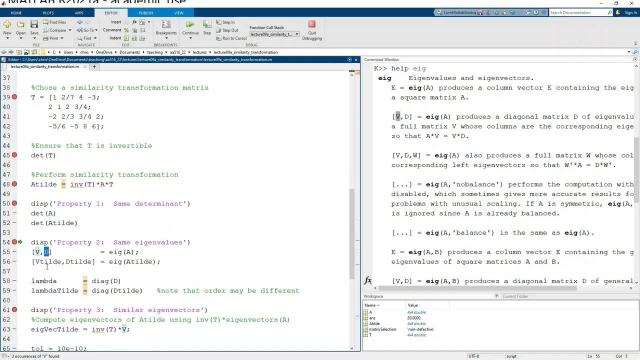 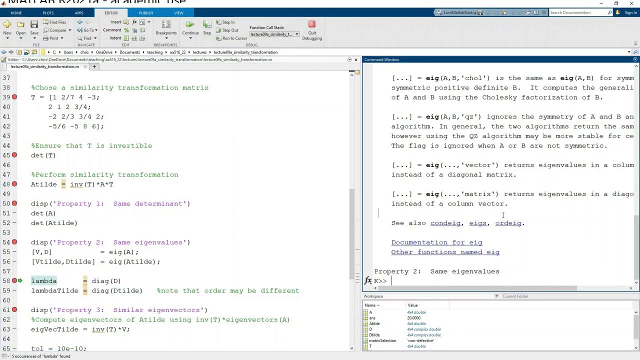 look at the eigenvectors of a and the eigenvalues of a, and then we'll look at the eigenvectors of- uh, a tilde and the eigenvalues of a tilde. here, um again, maybe let me put a break point right here and i'll run just at this point, and we can look at in, in this case for property two. i only care. 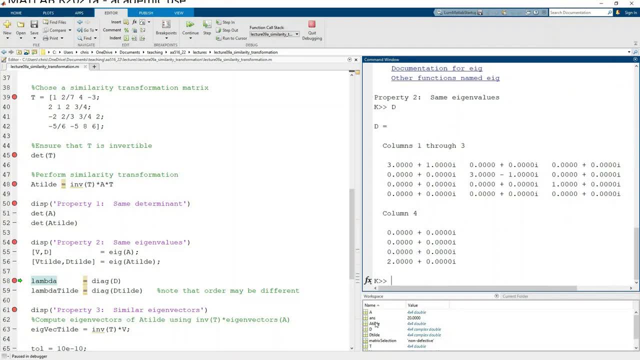 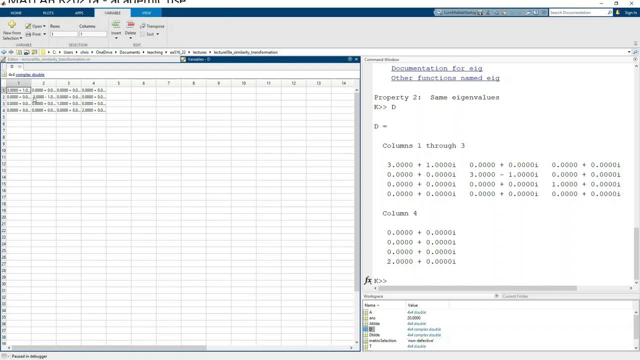 about eigenvalues. so let's look at d right and, as you can see, d is basically a diagonal matrix. i guess if we look at this- let me open up- you can see it's a diagonal matrix. these are all zeros. if you look at zero plus zero i. that's what all these other entries 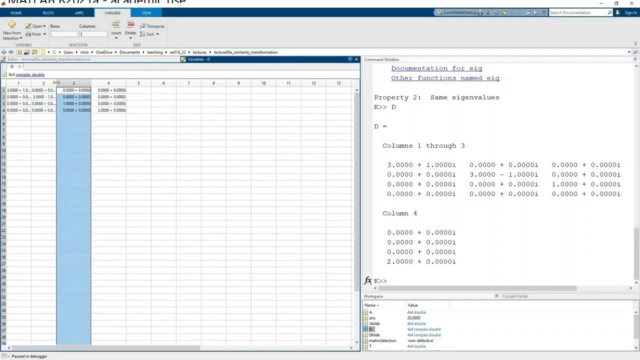 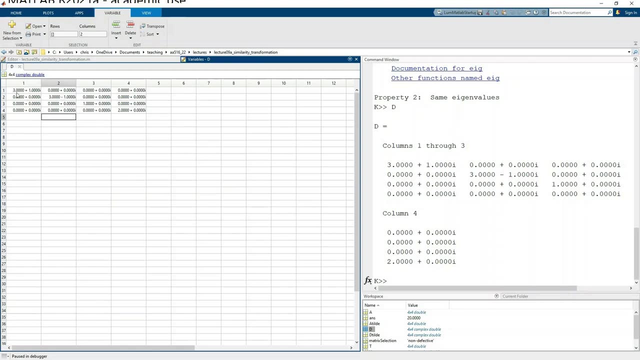 are. so there's only entries along the diagonals, and the diagonal entries are the eigenvalues. so that's what the i function is giving us. so it looks like for this matrix a, there's an eigenvalue at three plus one, i three minus one, i one and two right. that's the eigenvalues. so 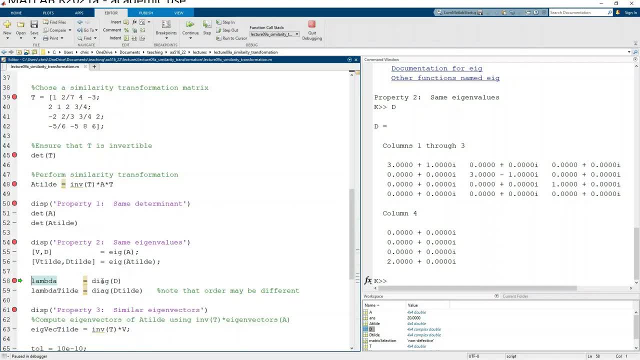 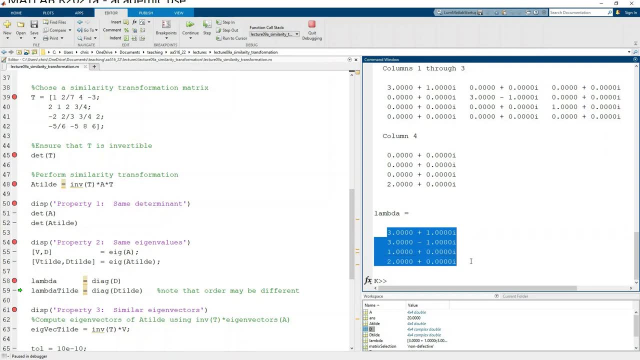 i'm actually going to rip them off using the diag function to just extract the diagonal entry. so again, if i f10 this and run that line, you'll see that lambda here. this is a list of all the eigen values of the matrix a. so again, it's like we said: it's three plus one, i three minus one, i one and two. 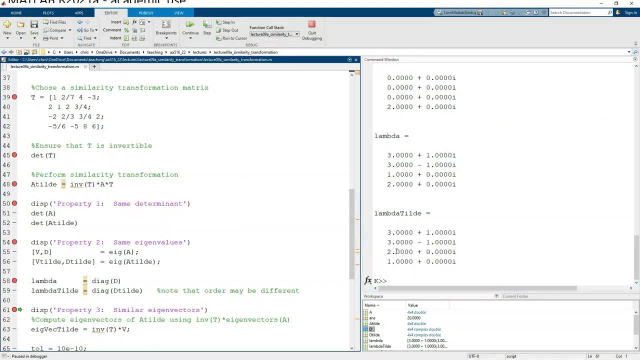 right, let's do the same thing for a tilde. and here you see that it's the same but a little bit different in the sense that the ordering is different. so look, the first thing that we're going to try to do here is replace the eigenvalues of the matrix as such. so again, the first two eigenvalues. 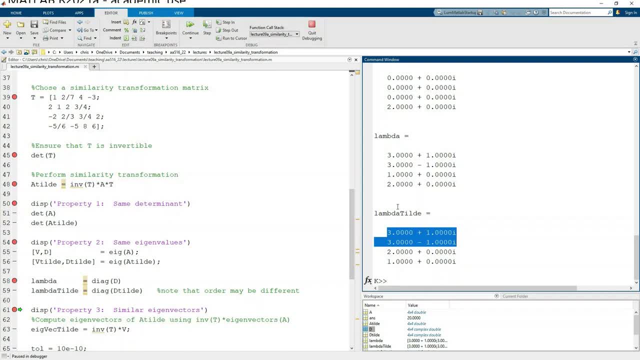 have the exact same value and order. but then you see that, for whatever reason, matlab's i function uh- decided to return us the eigenvalues in a different order. but regardless of that, the eigenvalues are actually the same. we just need to be a little bit careful that, for whatever reason, 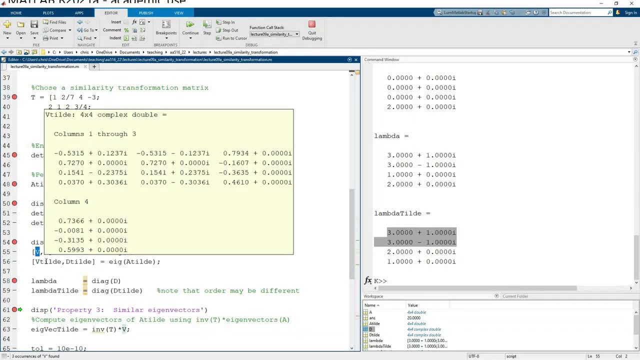 matlab decided to give us the eigenvalues in different orders. therefore, this matrix of eigen vectors are also- we got to be a little careful how, how we're going to play with them- all right, but property two: that basically- well, not basically, they are the same right- The eigenvalues of both. 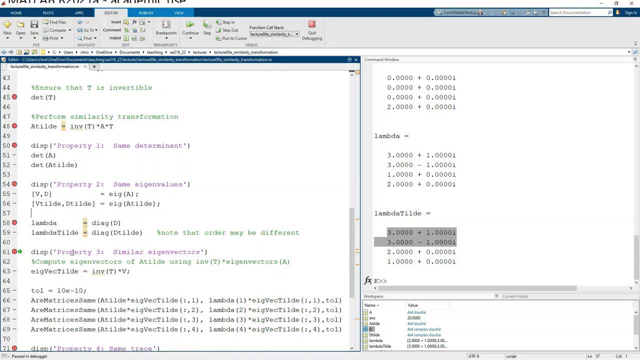 A and A tilde are the exact same. Now let's look at the eigenvectors, right? We discussed on the board that the eigenvectors of A tilde should basically be the eigenvectors of A, but then we have to multiply by inverse T, right? So that's what I'm going to do, right here. I'm going to 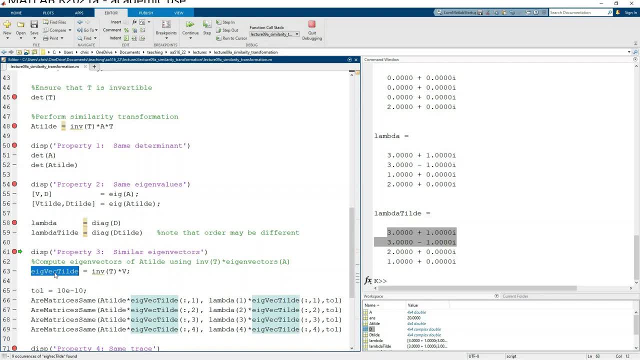 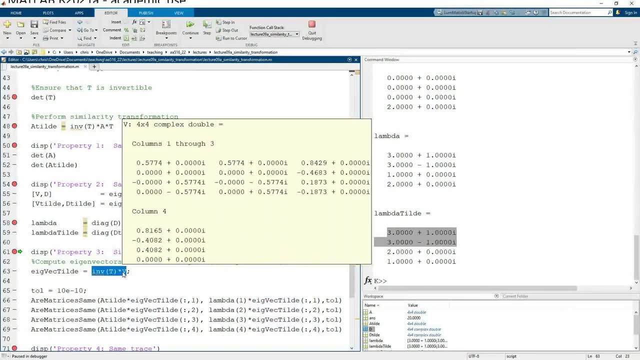 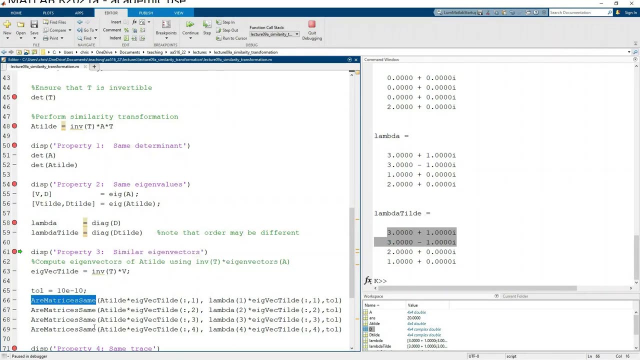 compute. what are the eigenvectors of A tilde? What should they be? using our relationship, we derived on the board of T inverse times the eigenvectors of A right. Now, what I'm going to do here is I wrote myself a small little function called are matrices same, So don't try to search. 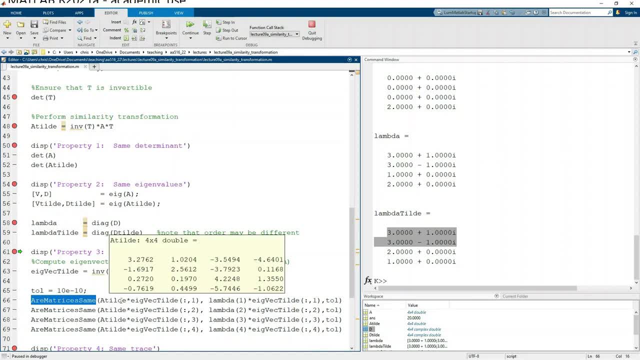 for this function on the MATLAB help. It's my own custom function, but I'm just checking to see if two matrices are the same within some tolerance. In this case it's 10E to the minus 10.. So it's some very small value. So, as you can see, what I'm doing right here is I'm checking that this. 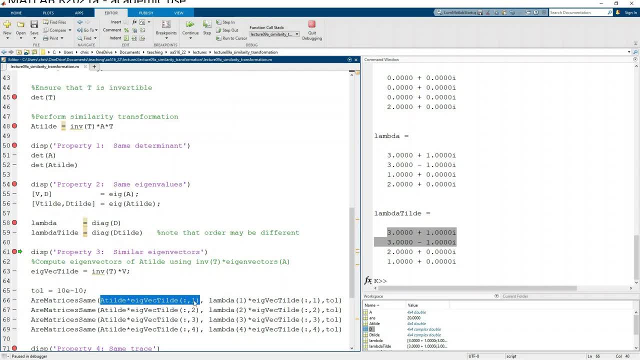 quantity A times the eigenvectors of A tilde is the same. So I'm checking that this quantity A times the eigenvectors of A tilde is the same. So I'm checking that this quantity A times the eigenvector one right Or what I think the eigenvector should be using this equation. 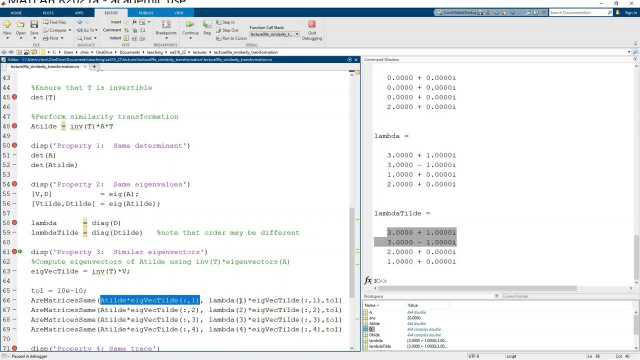 should be equal to the eigenvalue of A tilde, which is the exact same thing we just showed as the eigenvalue of A and A tilde. the exact same thing, right, But multiplied by this eigenvector of A tilde, right? So what I'm doing here is I'm checking to make sure that. 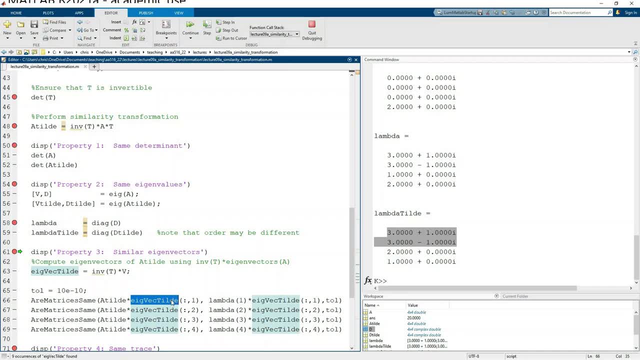 this thing: what I'm calling eigenvector tilde is actually the eigenvector of A tilde. So all of these should come back and say: true, true, true. So let me just step through this step, step. So, yep, the first one matches right. So this first eigenvector is correct. The second, 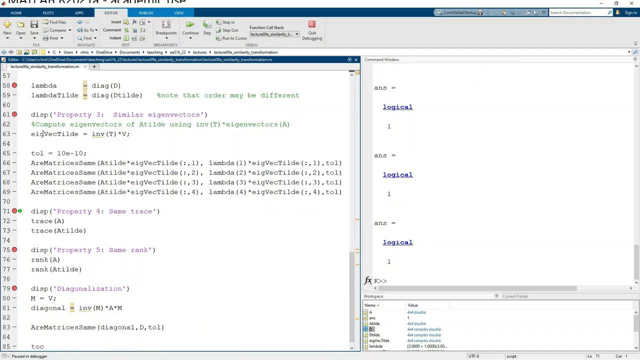 eigenvector matches, the third one matches and the fourth one matches. So I know that this thing right here, this eigenvector tilde, this is in fact the four eigenvectors of A tilde right. That's what we just proved. So 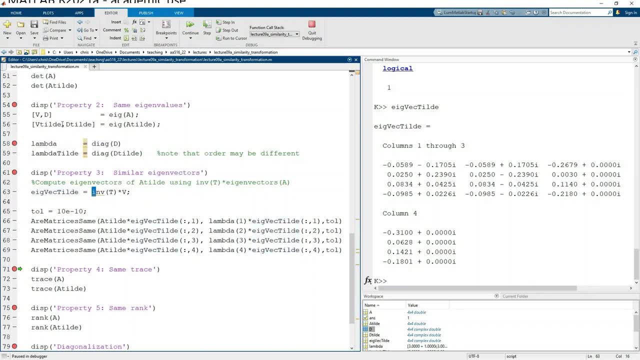 that's great because you saw we actually I did not use this at all. right, I did not use the eigenvectors that the MATLAB function I computed for me. I used the eigenvectors of the original A matrix and then used our similarity transformation to get those eigenvectors. 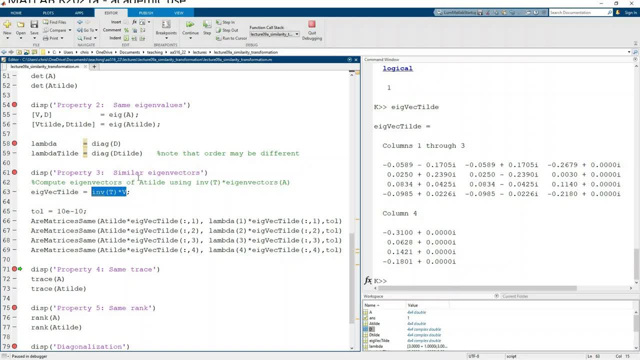 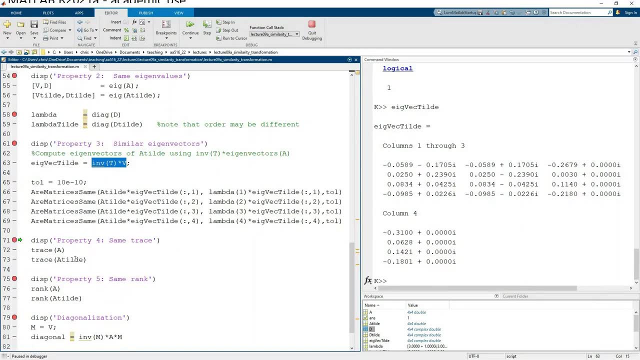 right. So this is great. It shows. property three is it works for this case where the eigenvectors are similar. They're related to the original A matrix eigenvectors through this transformation And the last two properties are almost trivial right. So again, I'm just going to look at the 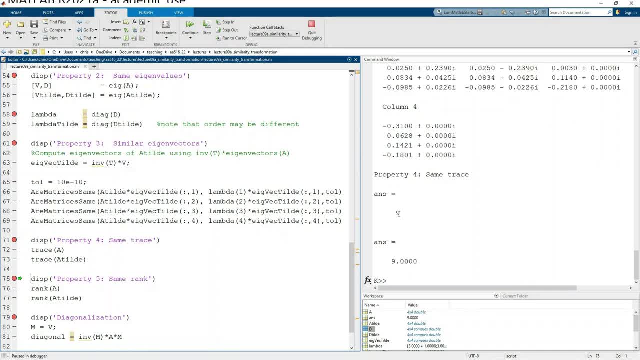 trace. Let's take a look at both those And we see, yeah, in both cases- A and A tilde both have a trace of nine and they should both have the same rank. So both of them have a rank of four. 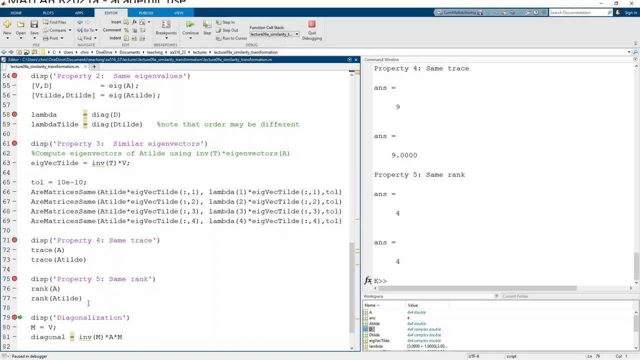 Now let's talk about diagonalization. So again, we just saw that those four, five properties were fine, regardless of the similarity transformation. Now let's switch gears and talk about diagonalization. So in this case, I do want to use a transformation. 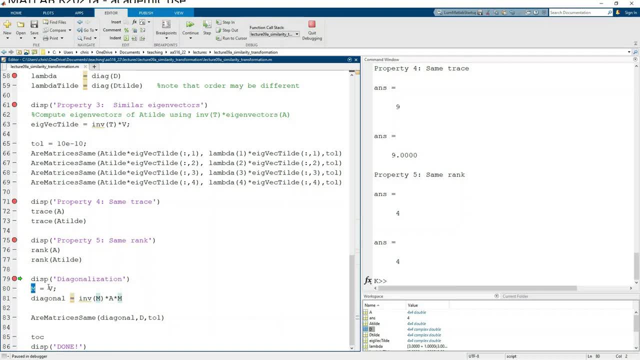 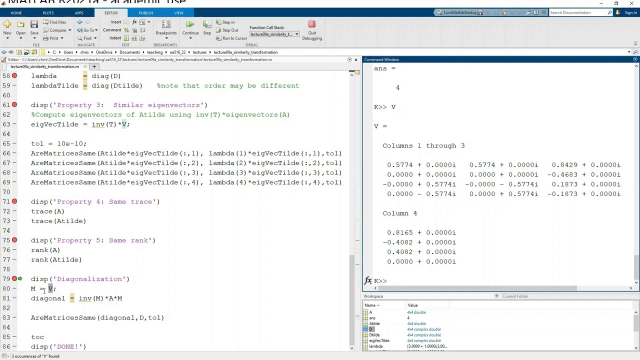 matrix. I'm going to call this the modal transformation matrix M and I want that to be the eigenvectors of the original A matrix. So again, make sure we're very clear on this right. This matrix V, this is the eigenvectors of A, not A tilde. So if I use the eigenvectors of A, 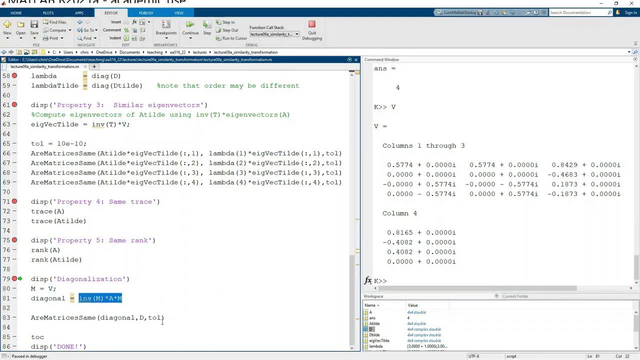 I can go ahead and perform my similarity transformation here using the modal transformation matrix And I should end up with a purely diagonal matrix with the eigenvalue along the diagonal. So again, let me just step, step, step And look at this Diagonal. 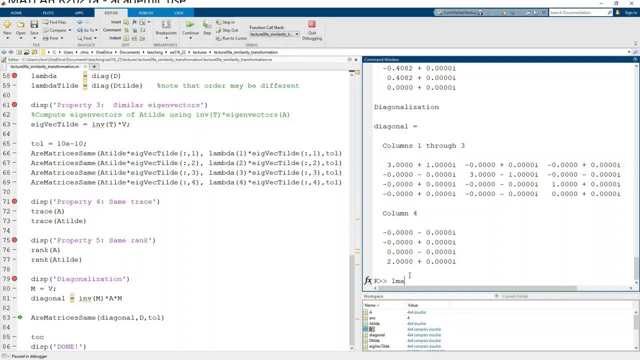 this totally works, right. If you remember, what do we call this thing? I think I made a variable lambda, right? This was the eigenvalues. It was three plus or minus one and one and two. And look at this: Here's three plus one, Here's three minus one, Here's one, And then here's two. 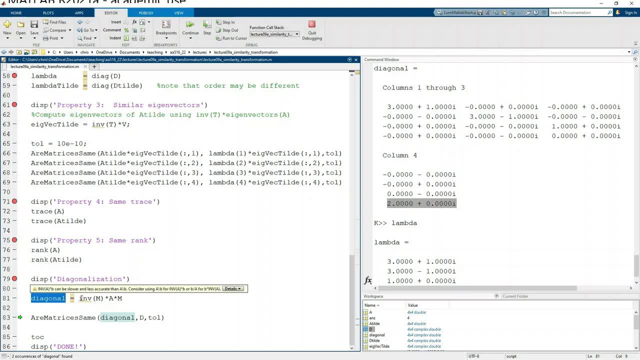 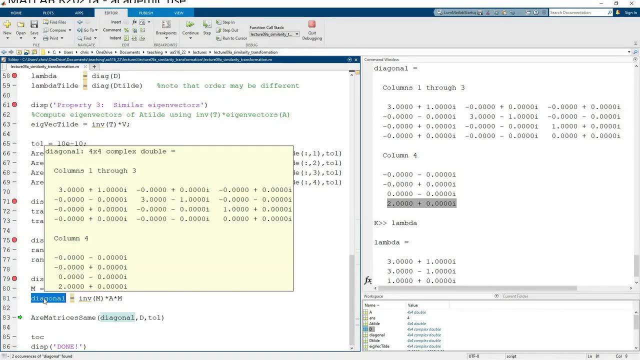 all along the diagonal. So, indeed, this similarity transformation, this similarity transformation or this modal similarity transformation, has gone ahead and diagonalized my A matrix. So this A tilde, which I call the diagonal, is indeed diagonal. So in this case it totally worked. 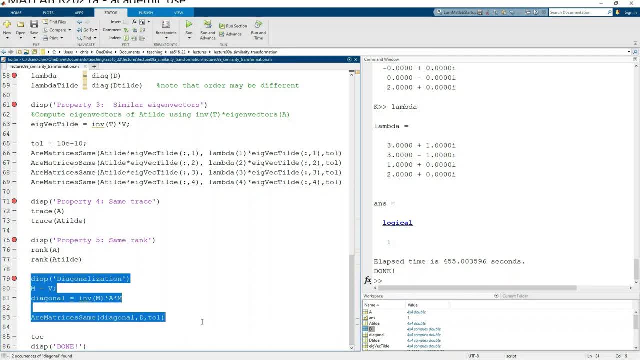 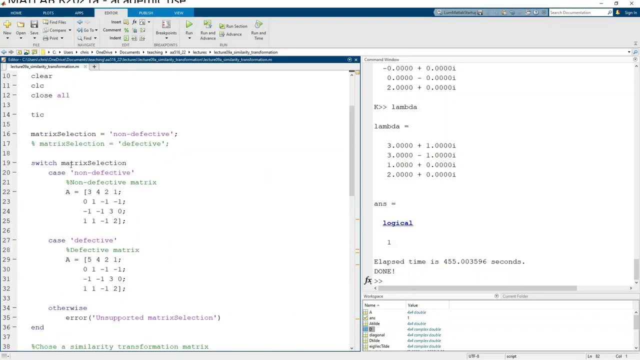 And when I say it totally worked, I mean the diagonalization process worked for this non-defective matrix. okay, Now let's go ahead and change this. Instead of using a non-defective matrix, let's use the defective matrix And go through this exact same exercise. So again, let's go ahead, and I guess I can take. 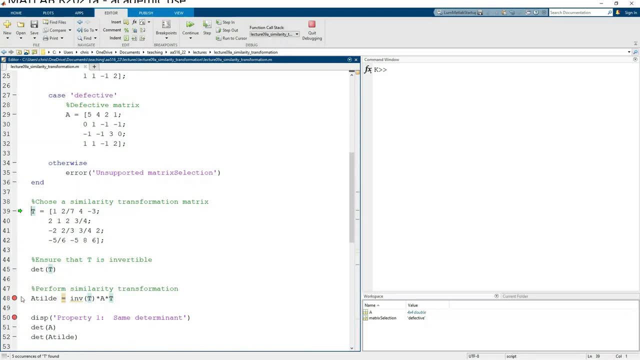 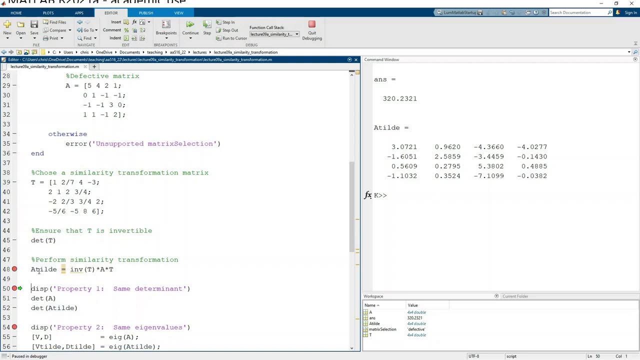 all these breakpoints off, because none of this is going to change. Yeah, this transformation matrix is still going to be invertible. I can still go ahead and compute A tilde, which again here this looks a little bit different, right, But again, we should be able to see that all. 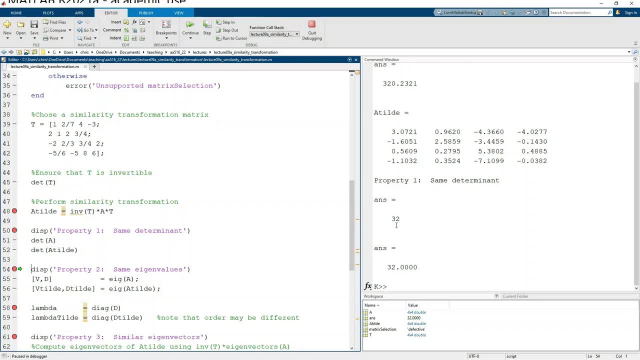 these properties are the same. So again, let's check the determinants. Yep, in both cases the determinants are now 32.. I think it was 20 earlier, But again, it doesn't matter because they're both the same. We can also see that the eigenvalues are also the 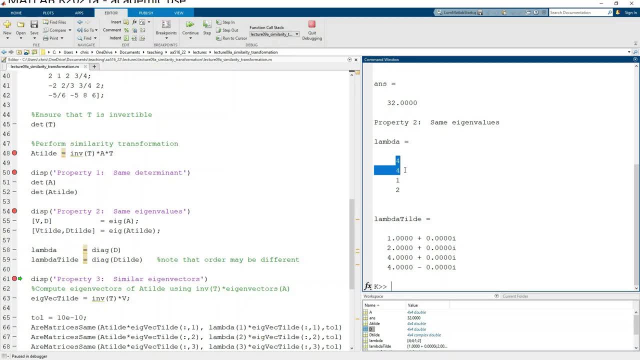 same. So now, in this case- aha, now look at this- We've got multiplicity of the eigenvalues. here We've got a 4 and a 4, okay, Which is going to potentially cause us problems when we start. 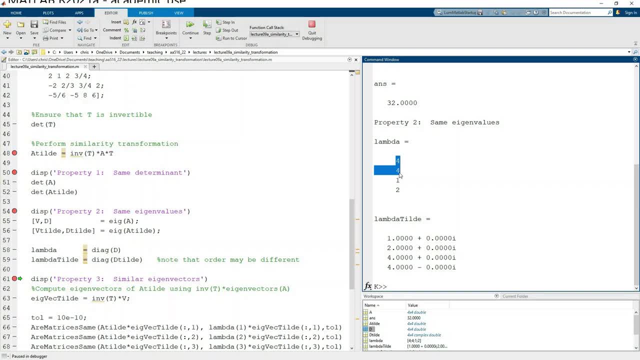 looking at the eigenvectors. But again, what's important to note here is that both A and A tilde have the same eigenvalues, namely 4, 4, 1, 2.. And again, look at this, For whatever reason, 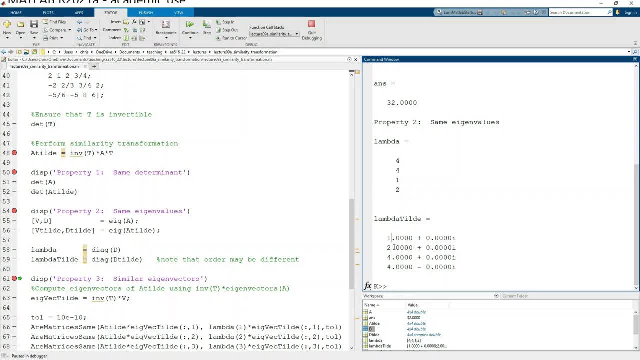 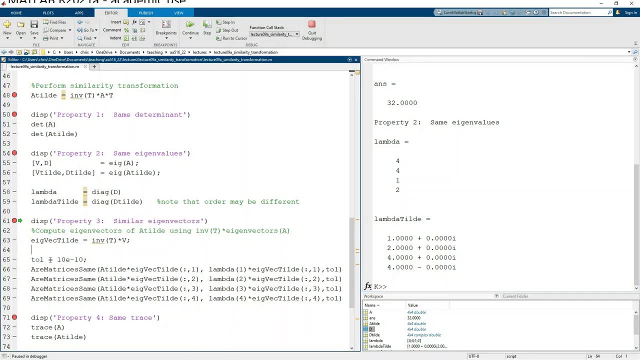 the ordering is different, But still it's 4,, 4,, 1,, 2, right, Same eigenvalues, And again we can do the eigenvectors. Let's go ahead and compute the eigenvectors. So again, I'll just hit F5, run through all these And we see. 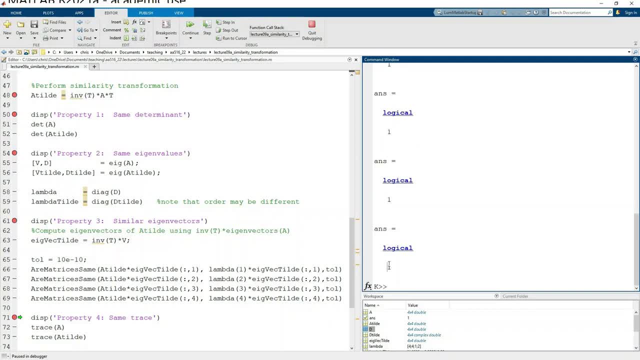 that yep checks out 1,, 2,, 3, 4.. So all four of these eigenvectors- yeah well, they are eigenvectors of the A tilde matrix. Now, what's interesting is- maybe we should interject here- is if we look at 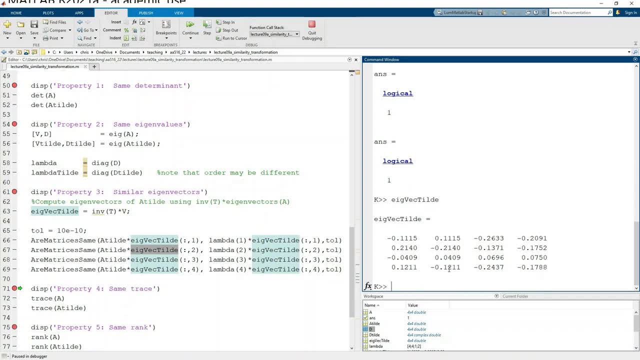 this eigenvector matrix. if we look at the rank of this thing- aha, look at that- The rank is only 3.. So in this case, the eigenvectors of A tilde do not span the space, And in fact, the same is true. 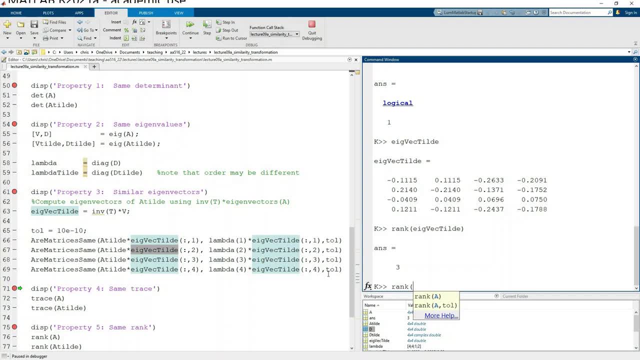 of the rank of the eigenvectors of A, And in fact, that's probably what we wanted to look at in the first place, because this is what we're going to use down the road when we start talking about diagonalization. And again, 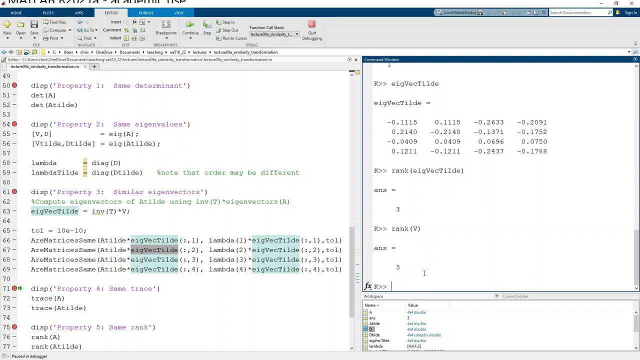 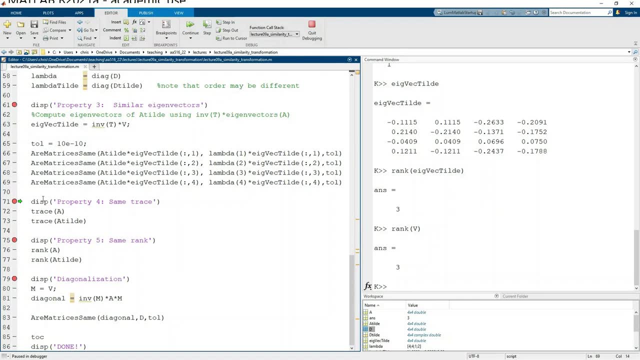 look at this, It's also rank 3.. So, okay, well, keep that in the back of your head. We'll revisit this in about 60 seconds, But in the meantime, let's go ahead and convince ourselves that, even with this defective A matrix, it doesn't matter. The traces are the same, right In this case? 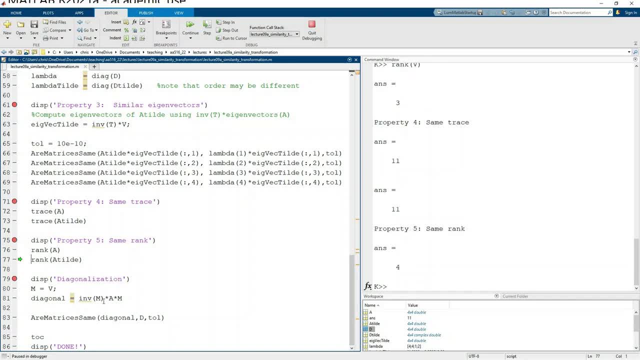 they're both 11.. And now the rank of A and A tilde are the same And again there's still full rank. right, There were no zero eigenvalues But the eigenvectors. now this is where we come to it when we start trying to do diagonalization. So if I tried to use a 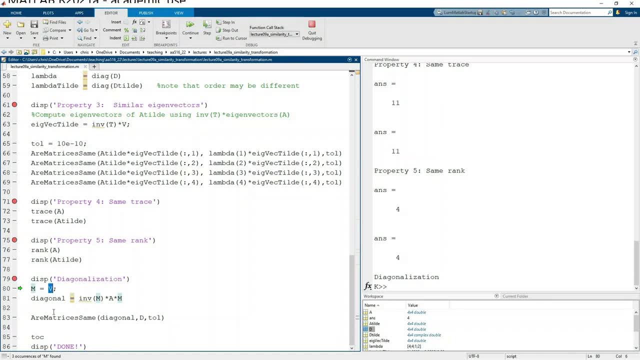 transformation matrix M, which is now the eigenvectors of A. the problem with this, as we saw earlier, is the rank of this thing is only 3.. So I can't actually do this. You cannot diagonalize any longer. You can't go ahead and say inverse M, right, This is going to fail. 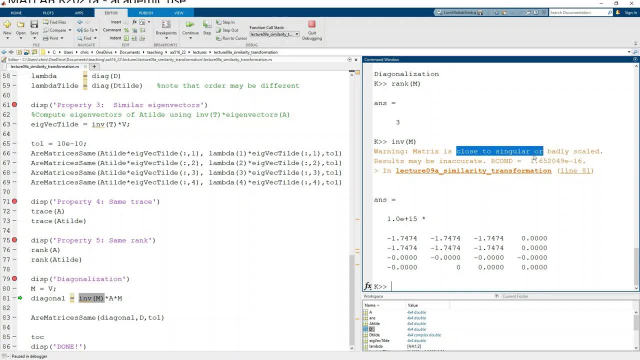 right, Because this thing there- look at this- It is singular or badly scaled, So it's not going to work. And again, when I say it's not going to work, we mean that we can't diagonalize the A matrix in this case, because it's a defective matrix and its eigenvectors do not span the. 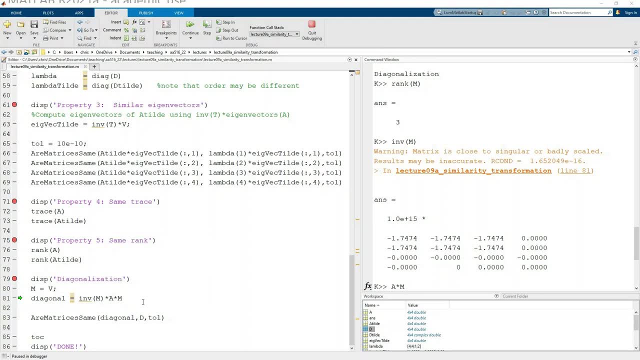 entire space. okay, So now this could be ameliorated to some degree by investigating what's known as Jordan normal form, But again, I think that's outside the scope of this discussion. We'll try to have another discussion in another video later, discussing Jordan form of matrices. 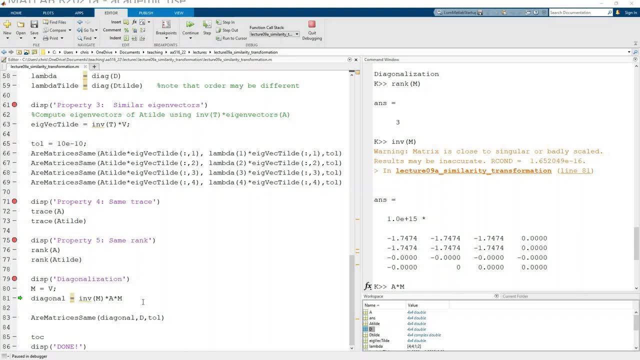 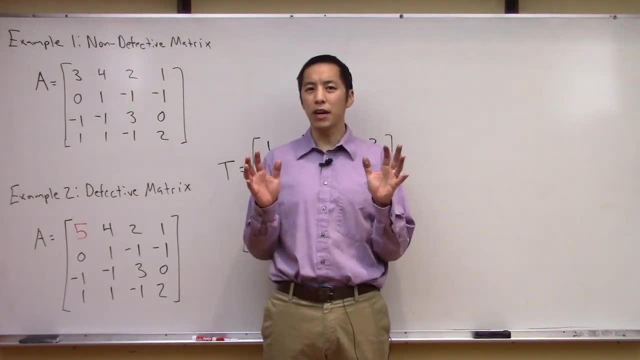 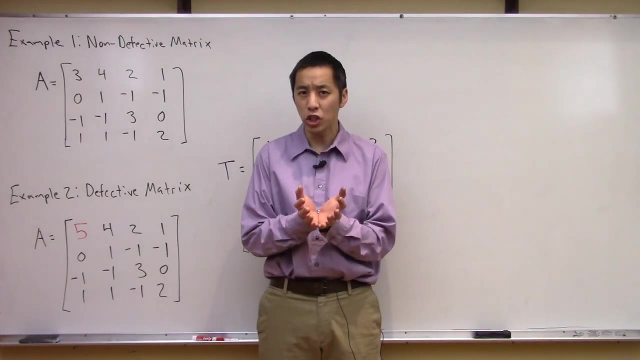 But for now, I think this is a good discussion, showing an example of all of these different properties under the similarity transformation. All right, so there you have it: a pretty mathematical sort of sterile approach and discussion and investigation on similarity transformations. In our immediately following video we'll take a look at trying to apply this. 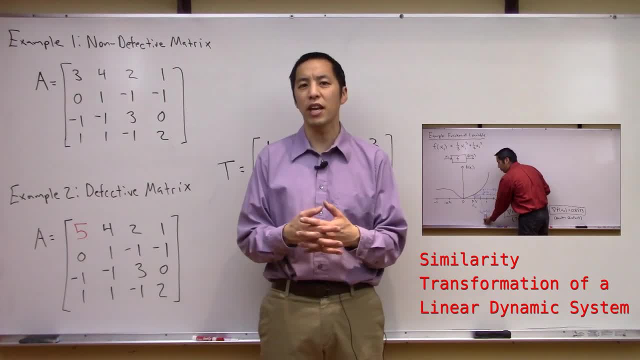 to an engineering problem of basically changing the states in a linear system using a similarity transformation. So we'll take a look at trying to apply this to an engineering problem of basically changing the states in a linear system using a similarity transformation. We're going to see how. 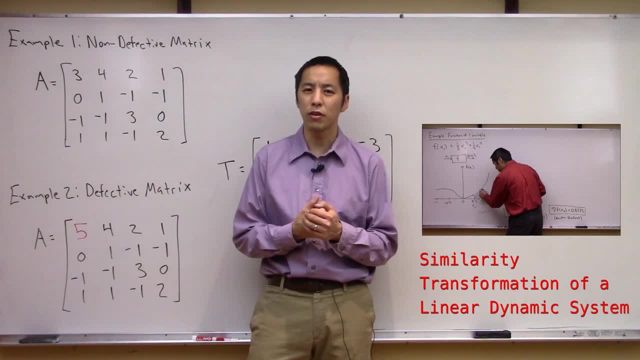 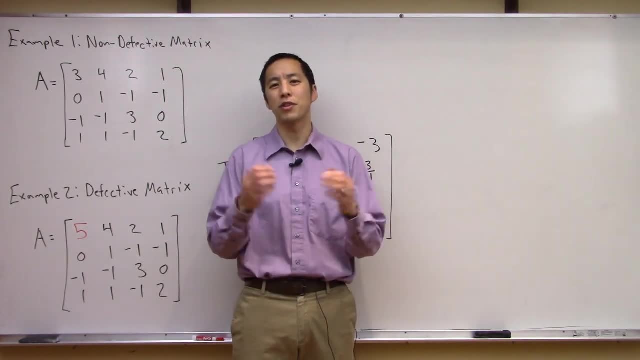 this might be actually applied to some control or dynamic systems applications. So, with that being said, I think this is probably a great spot to leave it. I hope you enjoyed the video And, if so, I also hope you'll consider subscribing to the channel If you scroll a little ways down and 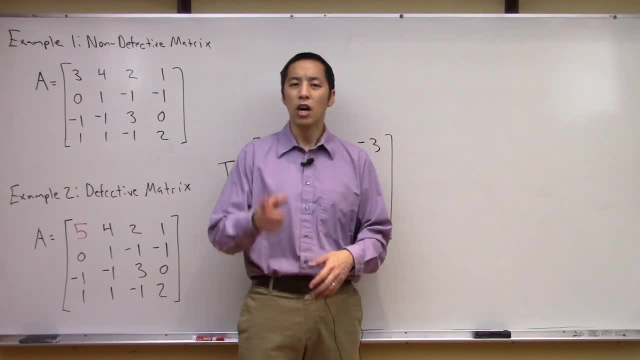 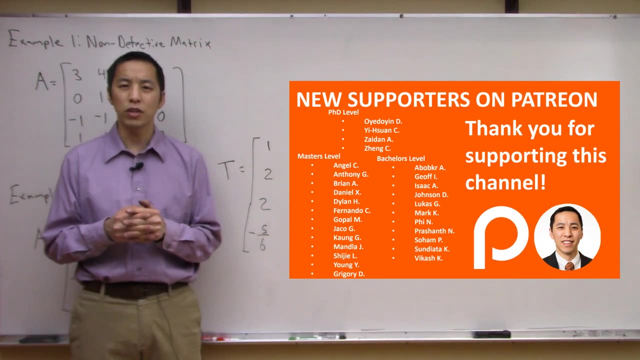 click on that subscribe button. it really does help me continue making these videos. The other way you can contribute and help the channel is via Patreon. I want to take a moment to thank some of our recent patrons. The nice thing about this method is that 100% of the proceeds that the